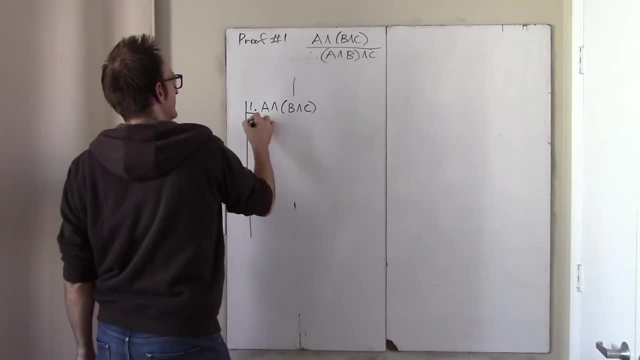 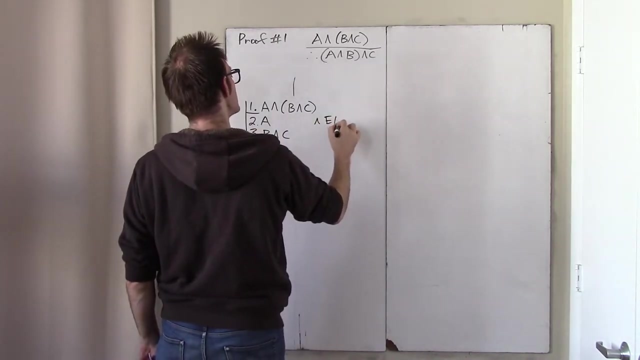 premise of our argument and we need to work down to here, okay. well, I think it's just clear what to do. we squeeze information out of this conjunction by decomposing this conjunction into the conjuncts a and B, a and B or C. Reason is: and elimination- It's a rule and elimination which tells us that. 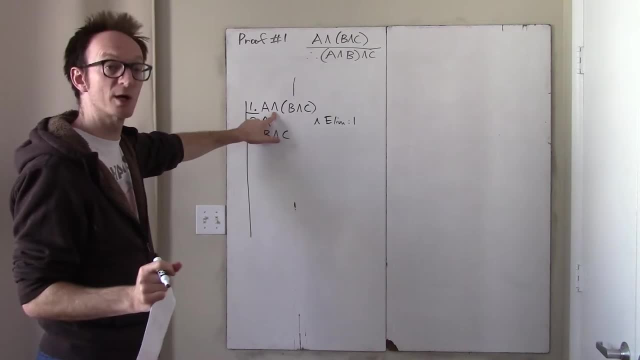 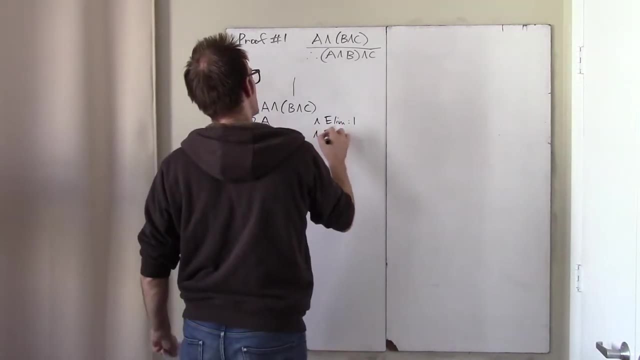 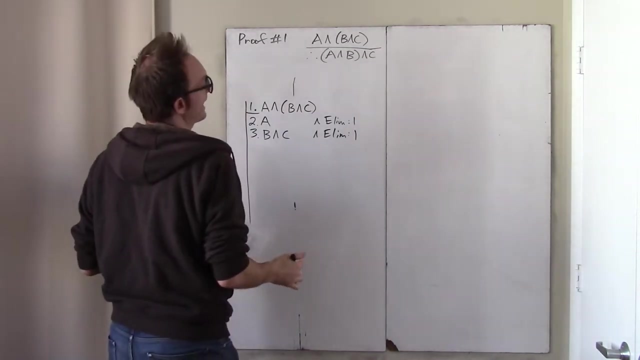 sort of the power of a conjunction is that if you know a conjunction or have a conjunction or are sure that it's true, then you can assert the truth of the conjuncts. So, applying that rule two times to decompose it, I'm now getting. 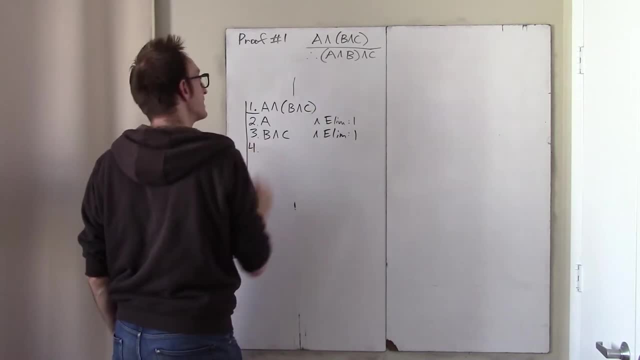 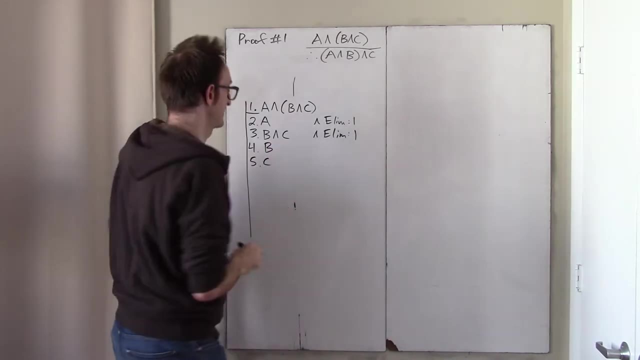 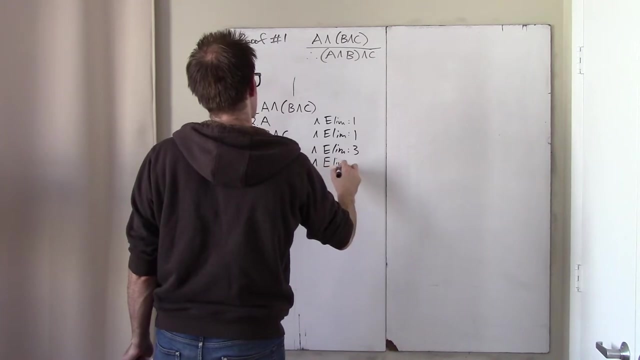 closer to what I want, I'll do one more thing, which is to decompose B and C into B, and might as well, at the same time, get C Reason and elim three. And so I notate, with a kind of a justification, every line of my proof, except for the 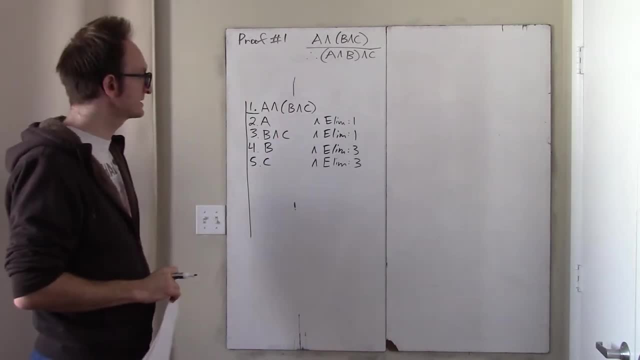 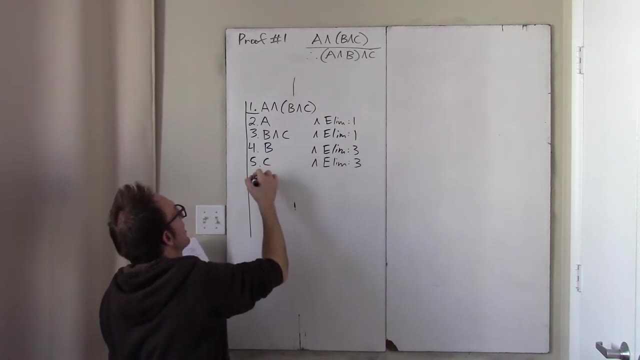 assumptions, Assumptions or premises don't get annotations because they don't need to be justified. Okay, here we are. Now. I want to show A and B and C, so I conjoin A and B together and that is a rule called an intro, which says that if you know two propositions, then you can. 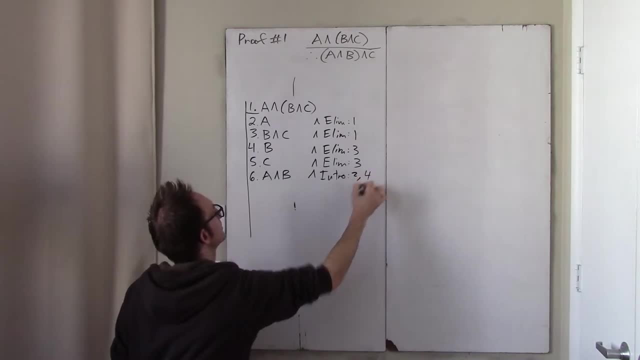 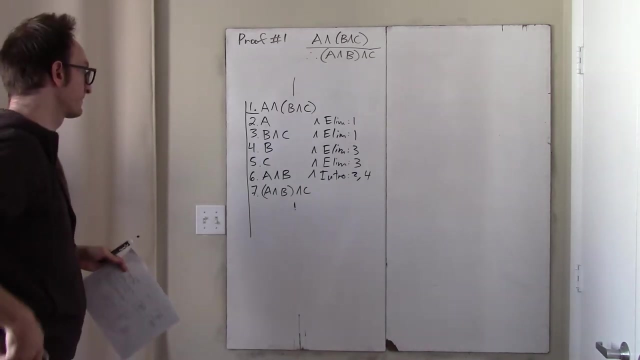 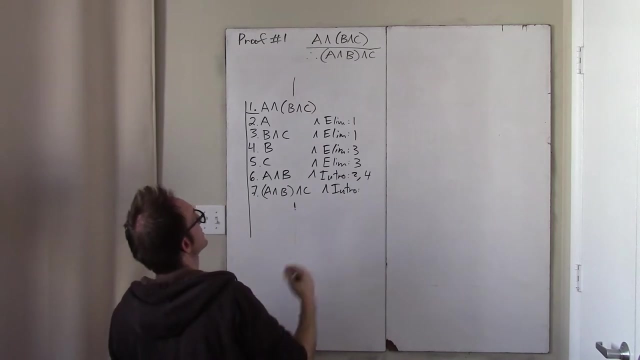 assert their conjunction. And so this is two and four. And finally, I and together cha-cha, I and together line five, and I get the thing that I want: justification and intro. What did I say? Six, five, Okay, good. 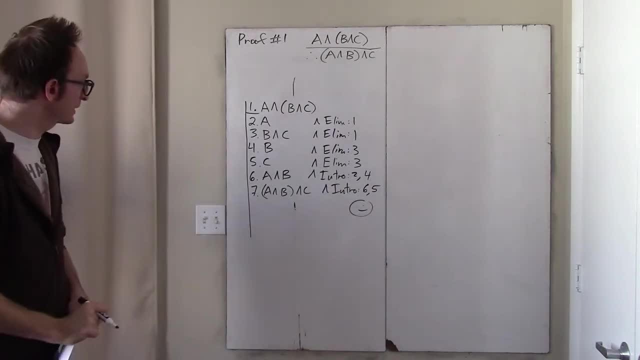 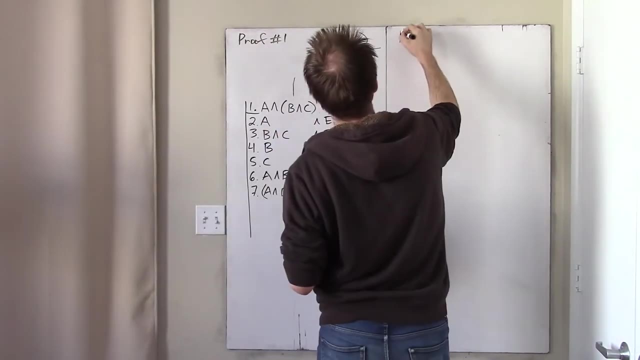 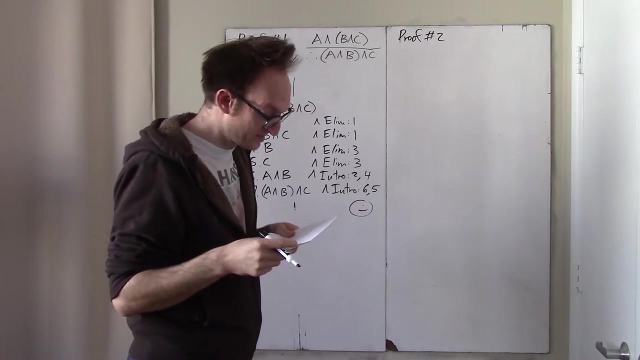 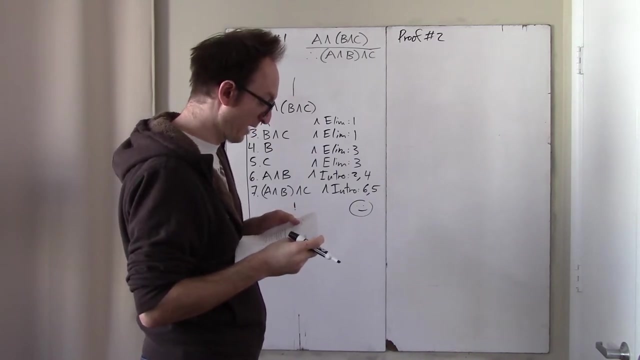 Whew Done. That was extremely straightforward and, you know, bordering on kind of just boring Good. More They get, more interesting, I swear, But not so quickly. Here we go. Here's proof two: This is going to exhibit some new properties. 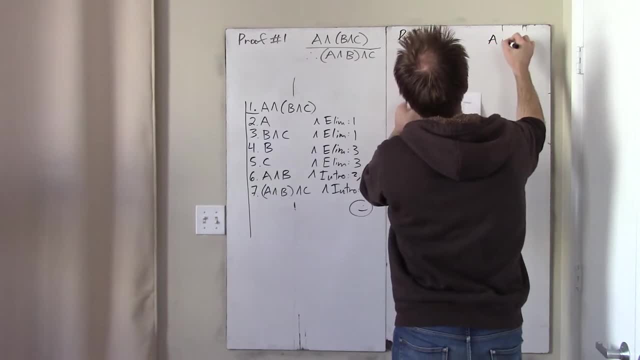 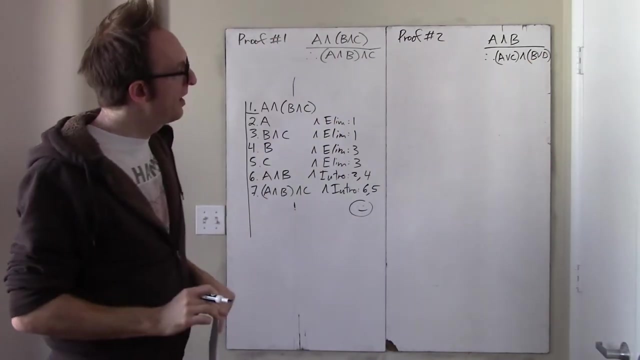 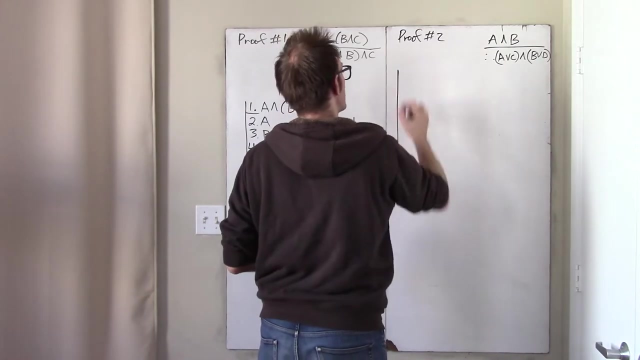 or something like that. Okay, well, what are we doing? Here is the argument. The argument is: premise A and B, conclusion A or C and B or D. Okay, well, if you think that out, you can convince yourself that that's surely true. Let's do the argument right now. This: 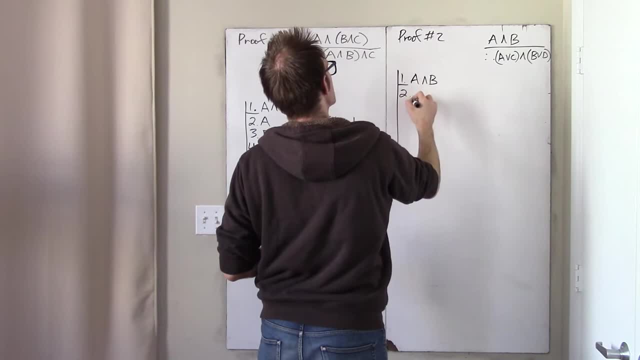 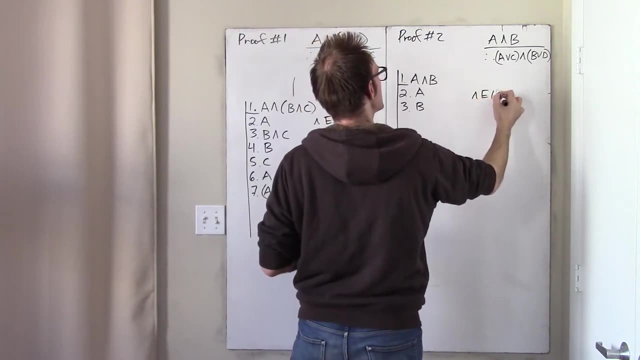 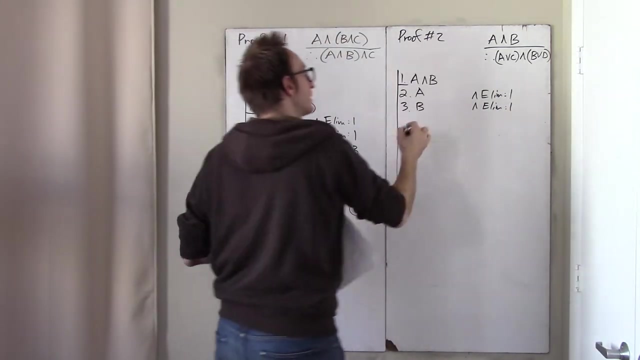 argument has one premise- A and B- and from this conjunction we can break it down into its two conjuncts, and elim one and elim one. But then we have a rule which says that if I know A, or rather if A is true, then I can break it down into its two conjuncts. 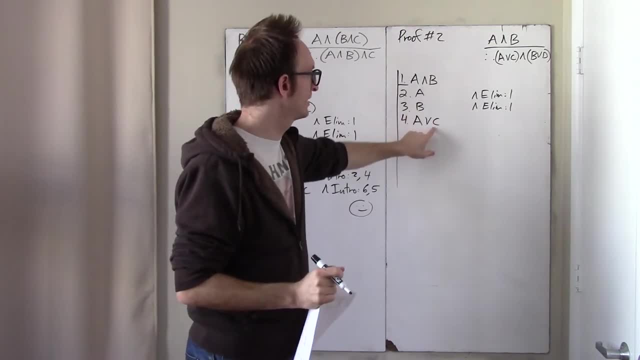 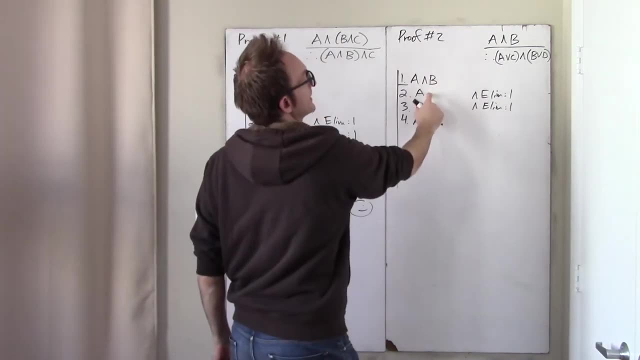 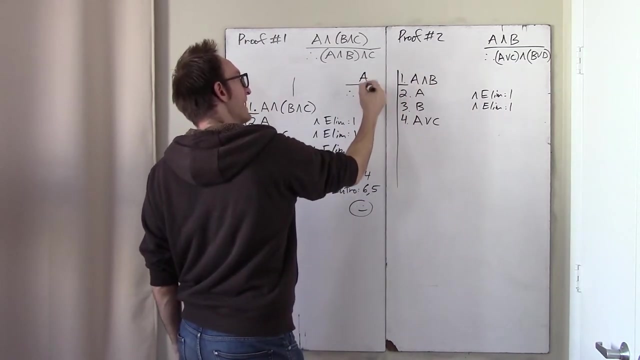 If A is true, then A or C is true. This is sort of a. you can think of it as kind of a weakening of the information in line two, but it is certainly valid that the argument that I'm claiming is valid now is the argument that says if A, then A or C. This is a valid 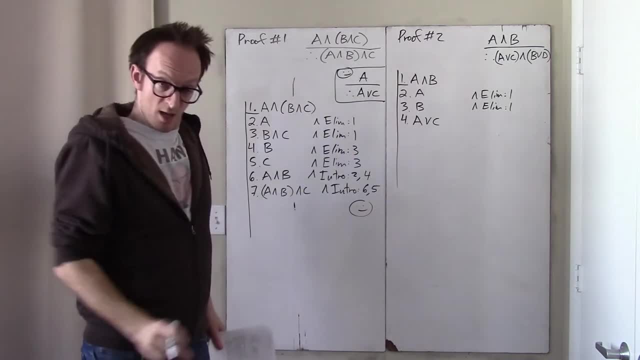 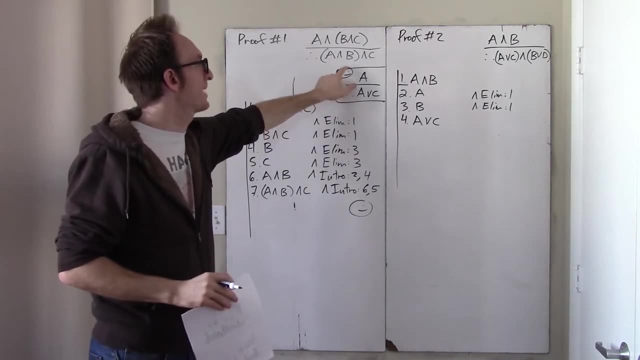 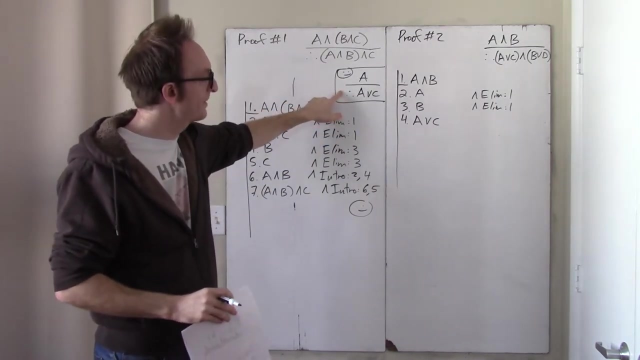 argument and that itself the validity of this argument can be checked, sort of by brute force, with the truth table. Okay, Okay, Okay, The truth table gives the semantics of these propositions. It tells you under precisely what conditions these propositions are true and false. And so, by making a truth table, 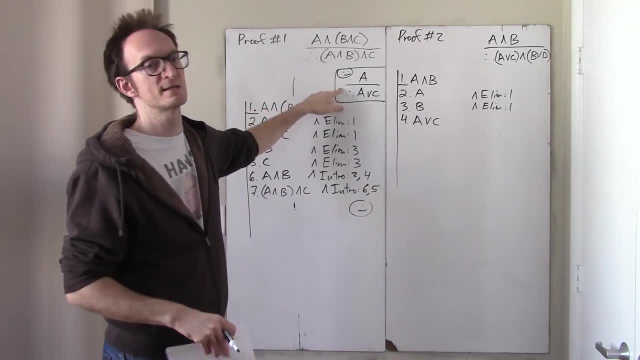 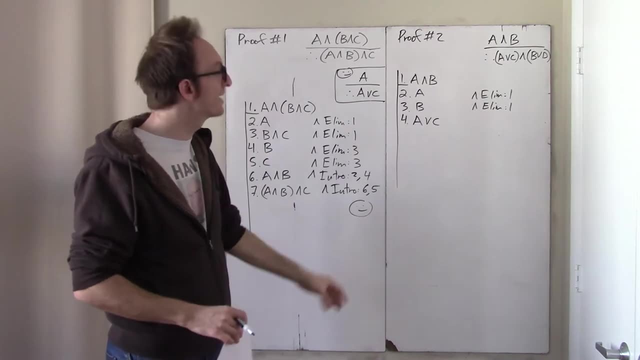 you can see that this argument is valid. The definition of validity is that whenever the premises are true, the conclusion is true, And if A is true, then by the definition of the or connective A or C is true as well. So since this argument is valid, then that 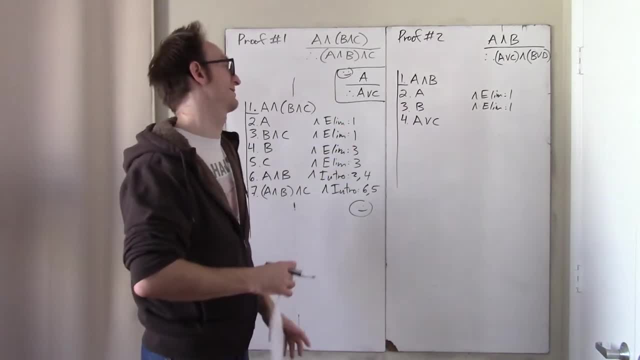 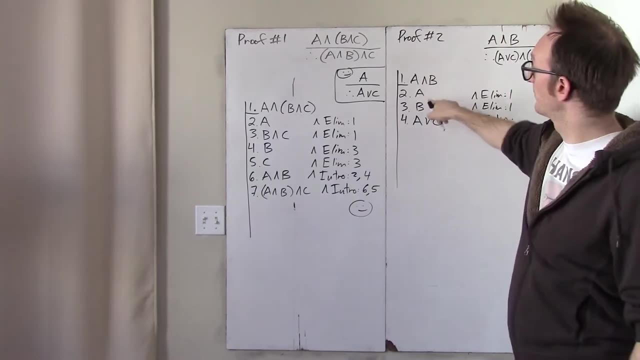 sort of is what justifies our rule. This is one way of looking at it, And the rule that I'm talking about is this rule, called or intro The rule. the sort of rule of logic that takes you from line two to line four- says that you can just add a. 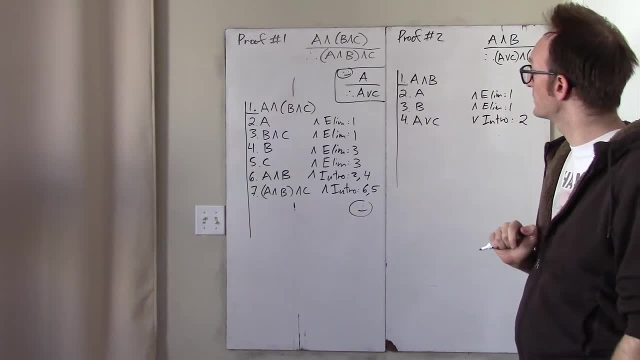 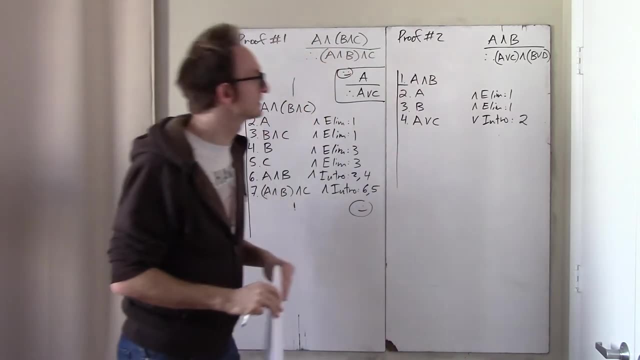 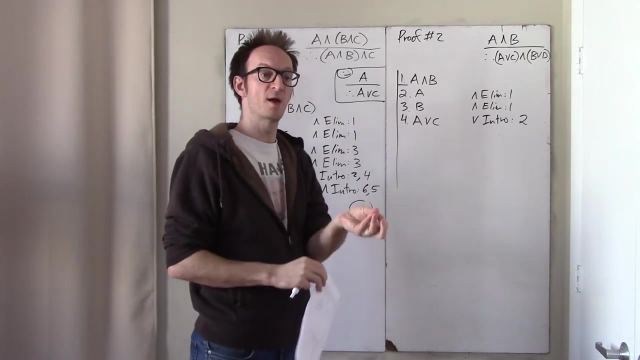 disjunction on to any proposition once you know that that proposition is true. Okay, So just to kind of repeat that one more time: the sort of understanding of what's going on here is that we have these rules that we're proposing, And then we have these: 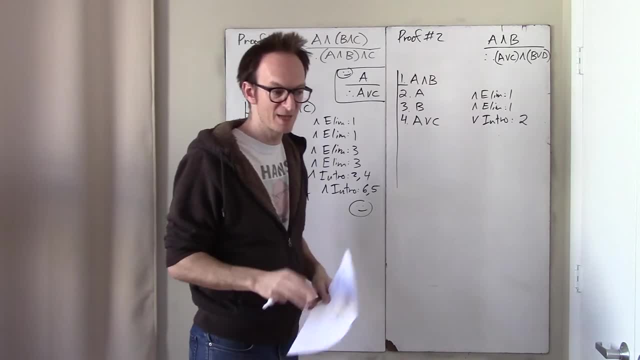 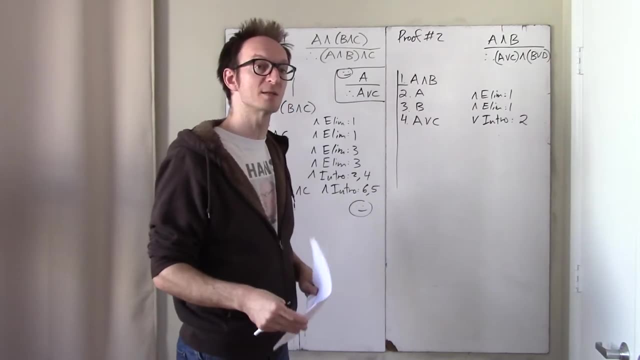 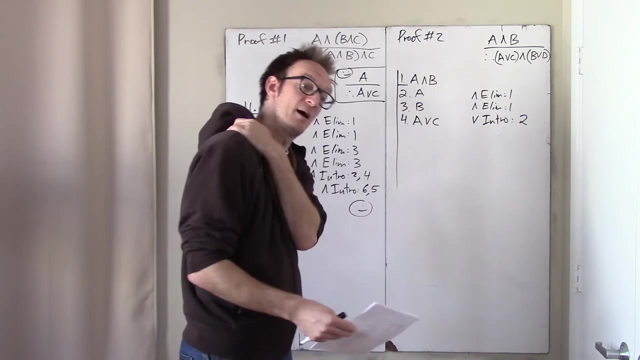 rules that we're proposing for our fit style proof system. Each of these rules can well- I think they're also very, very intuitively clear the rules, But if you want, the rules can themselves be justified as being sound, which is to say that the rules are truth-preserving. 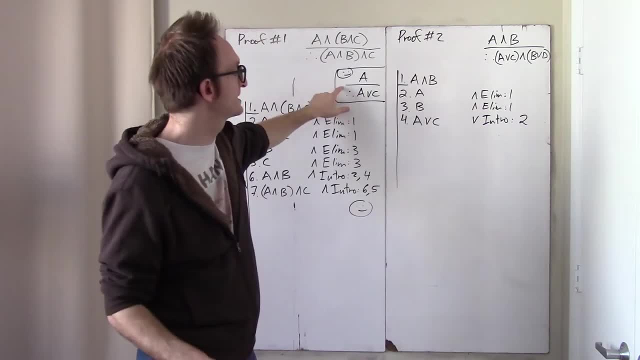 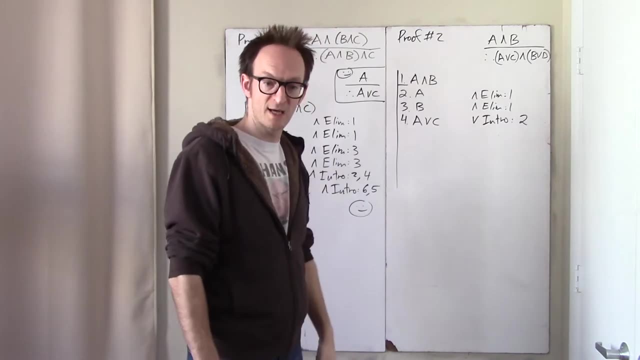 or that the rules produce valid arguments, And I didn't even bother doing it, but I talked it out. What I just did here is a sort of justification of the or intro rule. And so if the individual rules of our system are each produced valid arguments, then sort 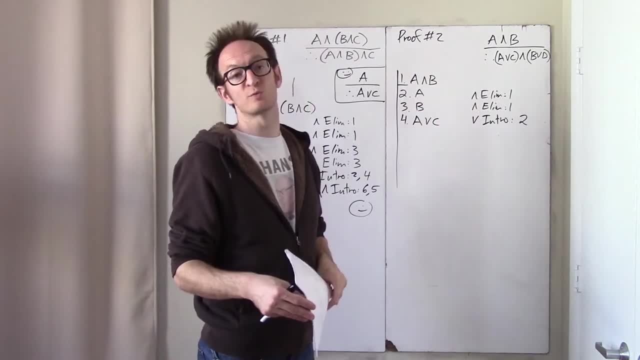 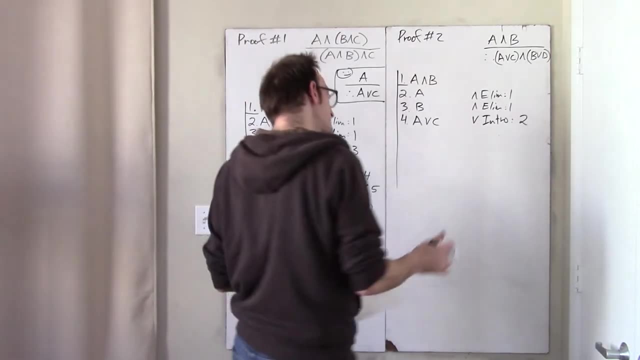 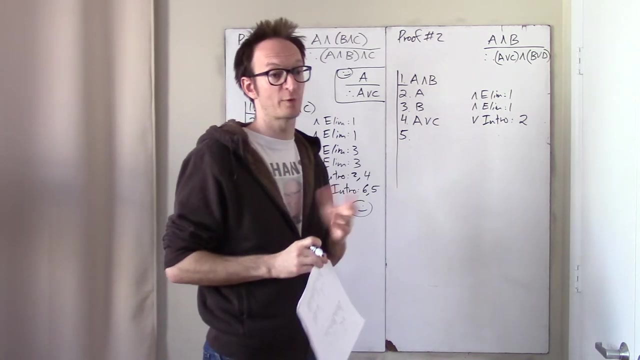 of repeated arbitrary applications of those rules will produce valid arguments. And that's just what a proof system is. It's a method for sort of generating valid arguments. Okay, And by limiting ourselves to some small number of basic rules. here we have two for. 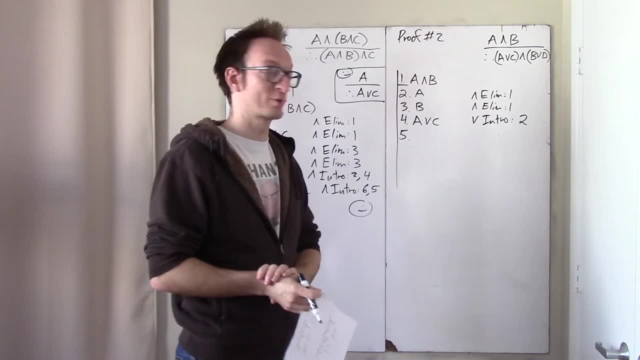 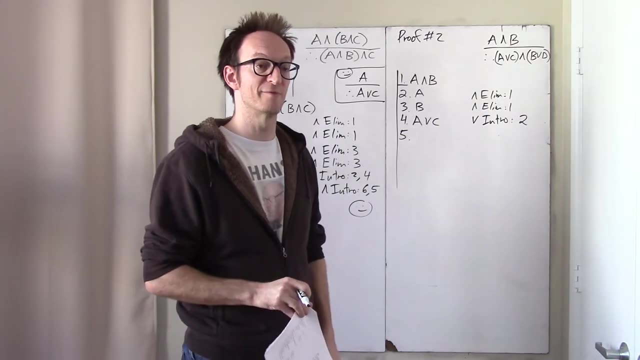 each connective. we then sort of reduce the burden of the argument, And so we have two for each connective. we then sort of reduce the burden of justifying our valid arguments via truth tables down to a sort of small number of basic arguments And more complex arguments. 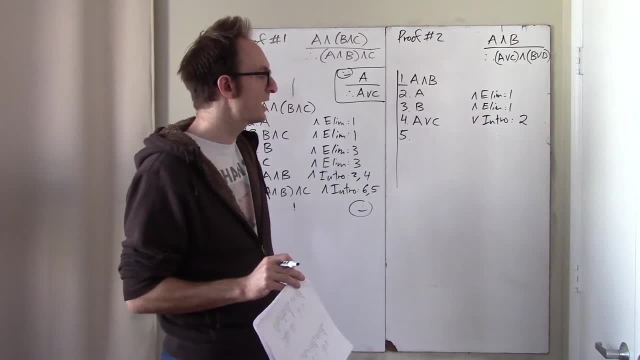 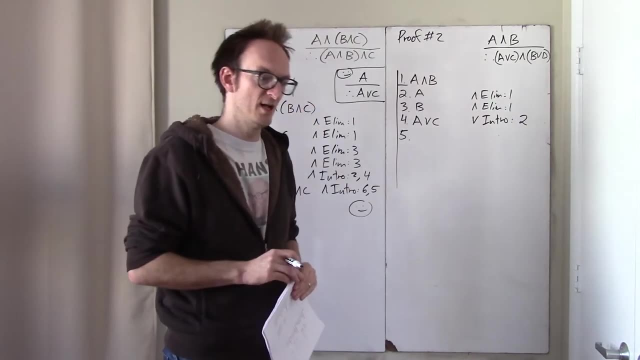 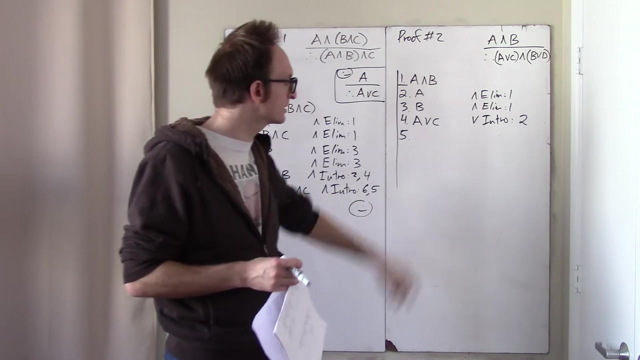 can be justified by virtue of these rules, And this is sort of to me, this is sort of doing logic. I think this is the point. When you're making truth tables, you're not really doing logic. in a certain sense, This is really doing logic, or constructing logical arguments. 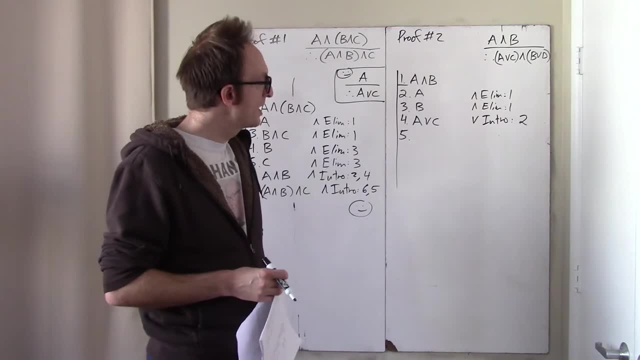 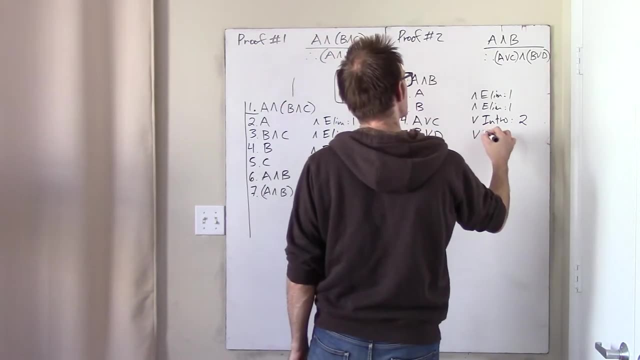 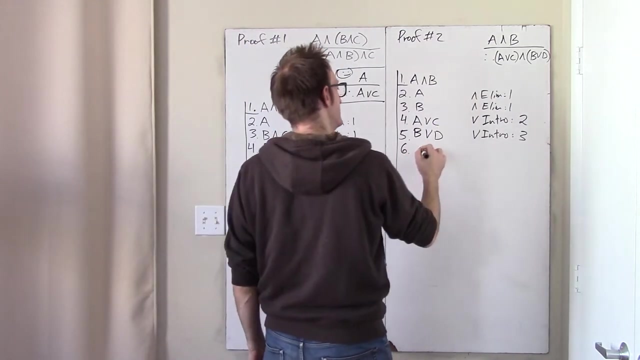 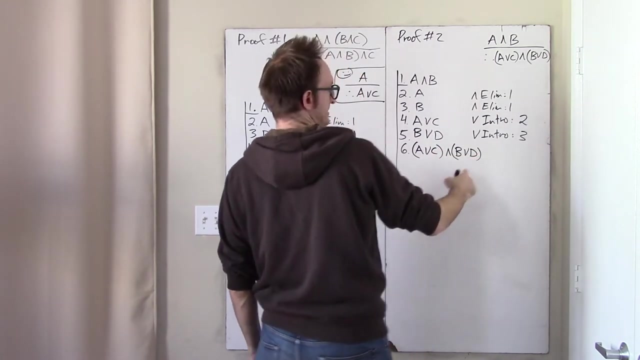 kind of the point of logic to begin with: Okay, Where was I going? Oh, yeah, I'm going to, or on a D, to this B reason, or intro line three. And finally, in rule six, this says that A or C and B or D, And that is coming. 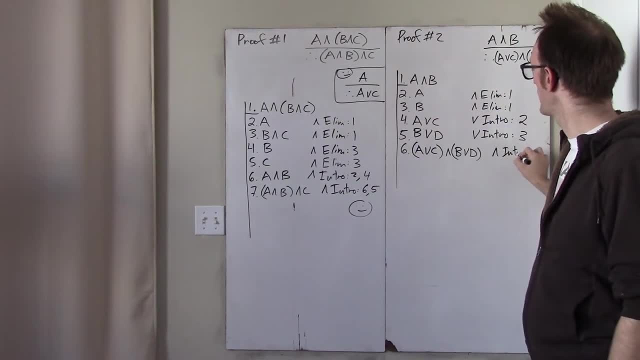 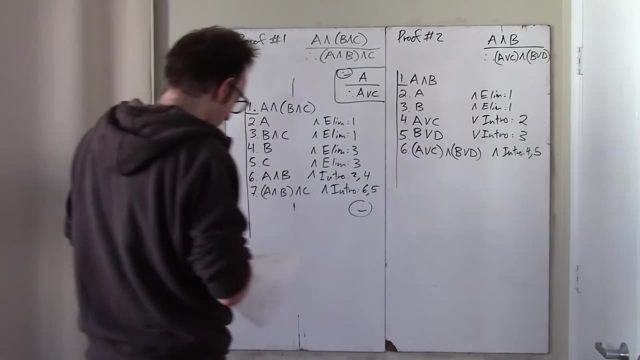 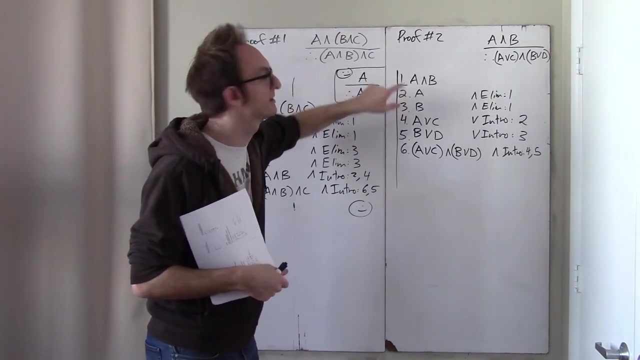 from the rule and intro: Yeah, Line four and five And so sort of, we sort of win. So okay, The way these proofs work. if this is not sort of clear, I'll just make it explicit. I didn't really say all this. 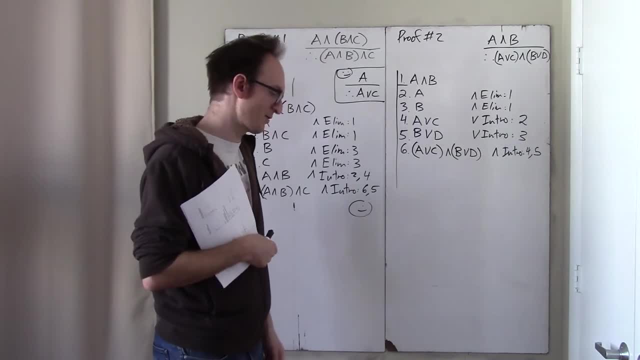 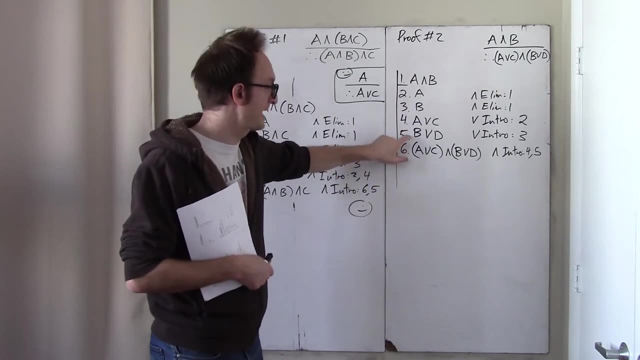 didn't go into this kind of level of detail in class. I took it as kind of I don't know obvious or something. But you know, the proof goes into kind of a linear fashion and every single line of the proof is potentially a place where you could have stopped, And so if the goal was to show that this argument is not going to stop, then it's going to stop. And so you know, the proof goes into kind of a linear fashion And every single line of the proof is potentially a place where you could have stopped. And so if the goal was to show that this argument 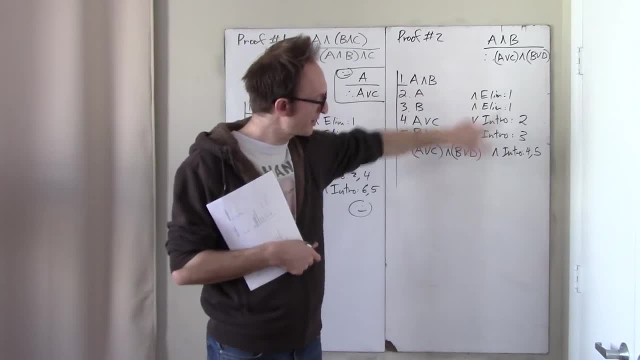 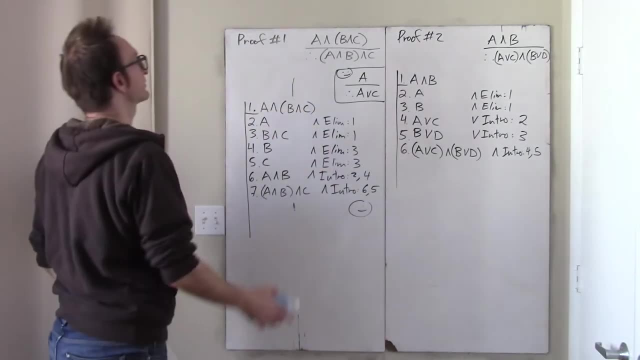 is valid. well, I have shown that this argument is valid As long as we know that all these individual rules are valid. I have gone from one to line six and there it is Okay. These two proofs were, you know, not that hard or interesting sort of or fun. 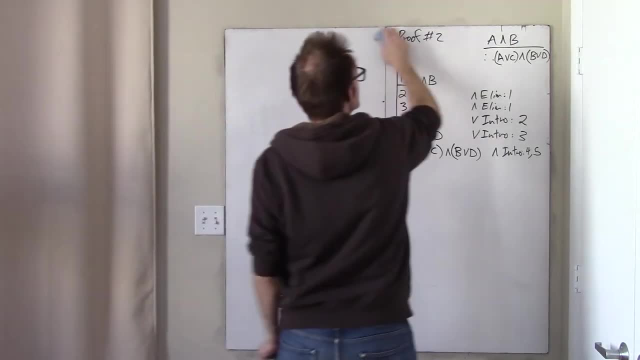 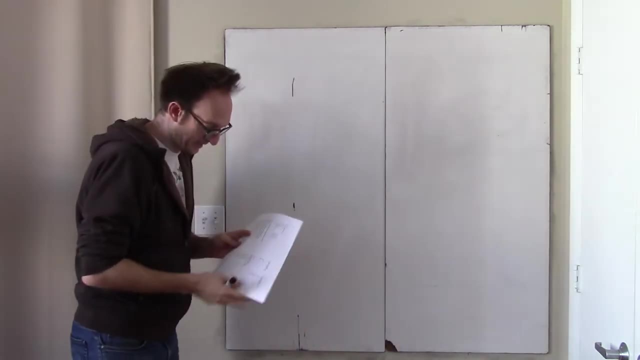 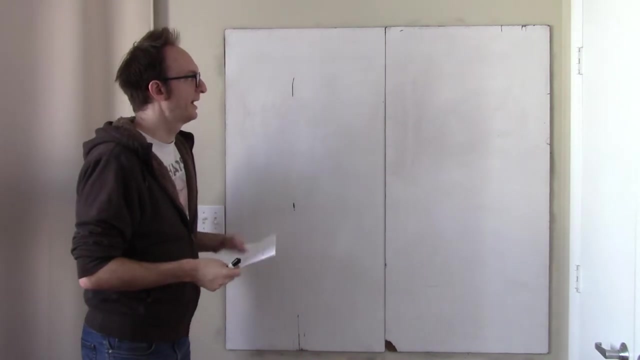 But they just give you a kind of a gist of our system. When it really gets kind of interesting is when you sort of start to think about the rules. And so you know, I have shown that when you sort of start expanding to a logical argument, that requires sort of 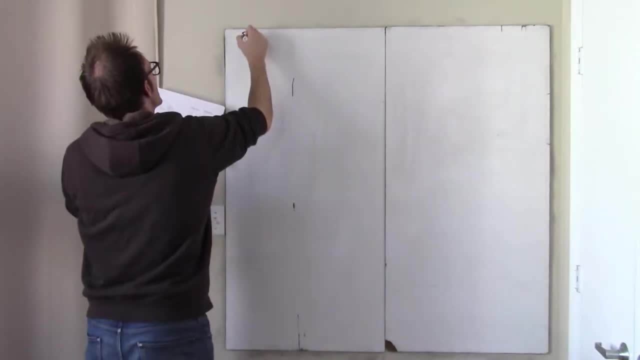 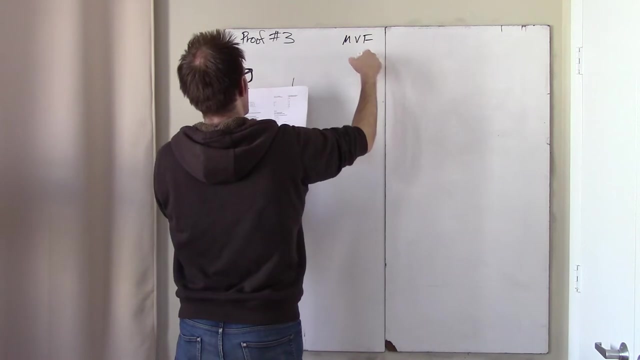 more complex arguments And here, okay, I will just do it. This was proof number three in the packet. This was given sort of verbally as a well, I will say over here that we have these premises: M or F. F implies C, M implies C, M implies 4.. M implies 4.. 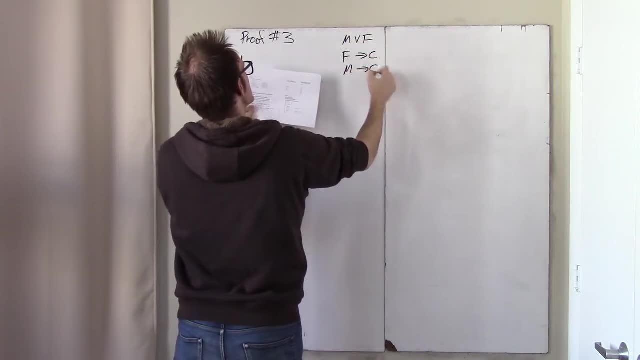 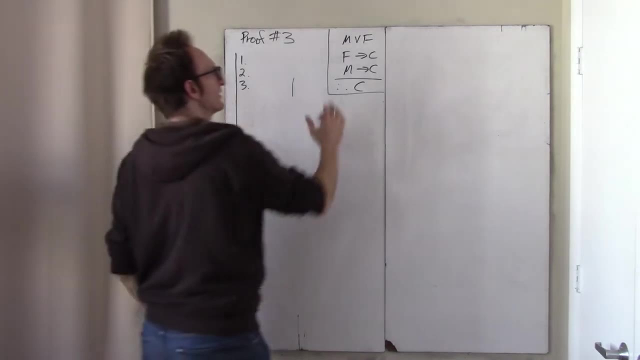 So 1 or 2.. These two points are pretty straight forward. I will say: One is that this was provided certain to provide a shared and bargaining process. So one is that that wasn't already C and therefore C. Okay, and in the package this was kind of stylized as some sort of 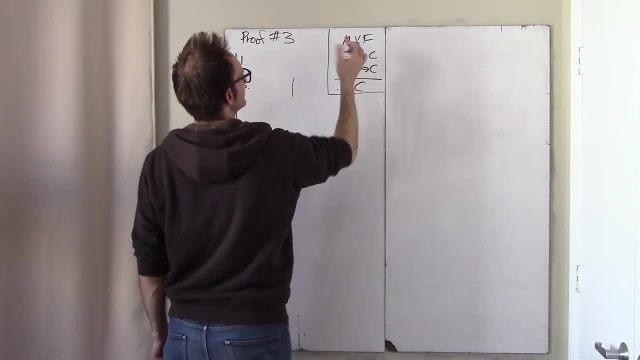 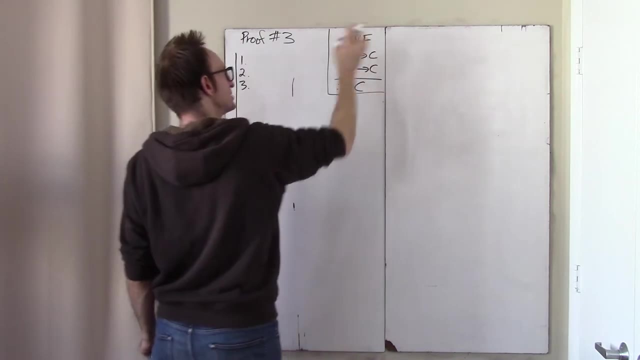 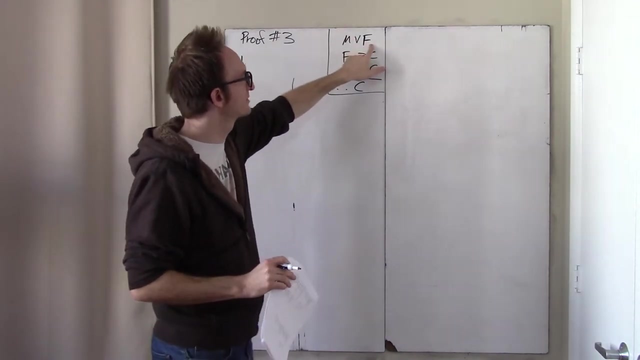 this was a sort of a bad example. that's very not bad, but kind of not interesting, or I should change it. but it was something like: you know, either my mother or my father, you know, is happy with me, or something like that: If my father is happy with me, I'm going. 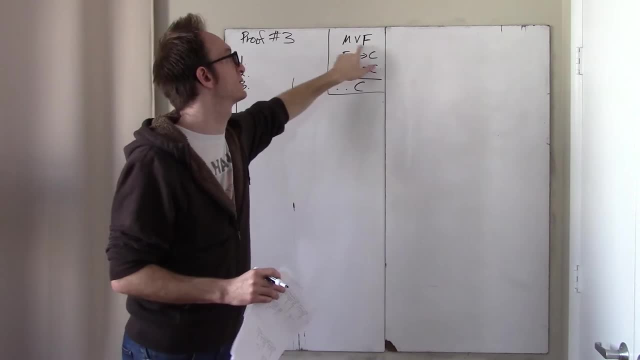 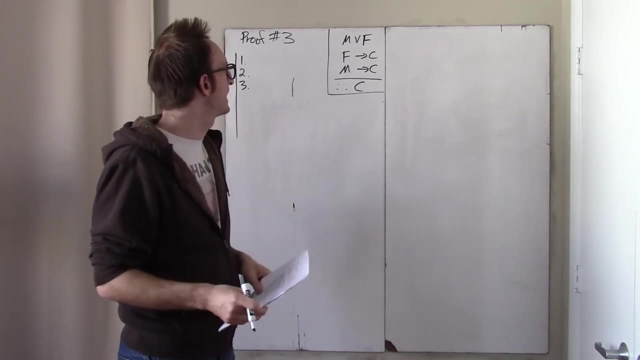 to get a car. If my mother is happy with me, I'm going to get a car. But since one of those must be true, then I'm going to get a car, Okay, Well, anyway, that's not important. What is important is that this argument here is sort of intuitively valid, never mind what. 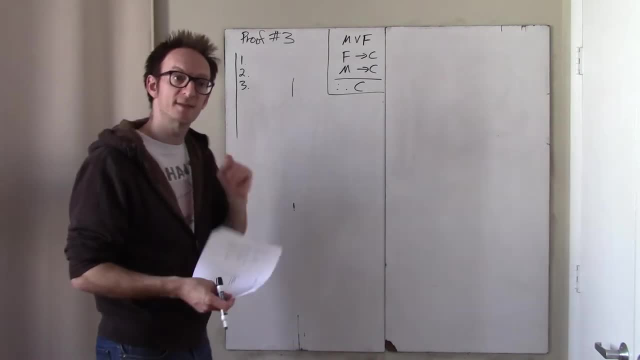 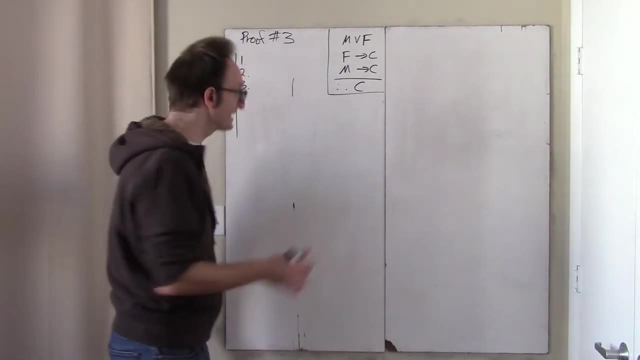 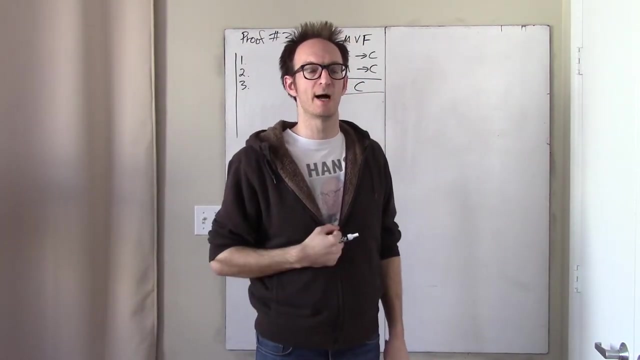 these propositional variables were supposed to represent. taking this more abstractly, Here we have this argument and I claim this argument is valid, And showing that this argument is valid Is well okay. there's always the option available, which is to just make a gigantic. 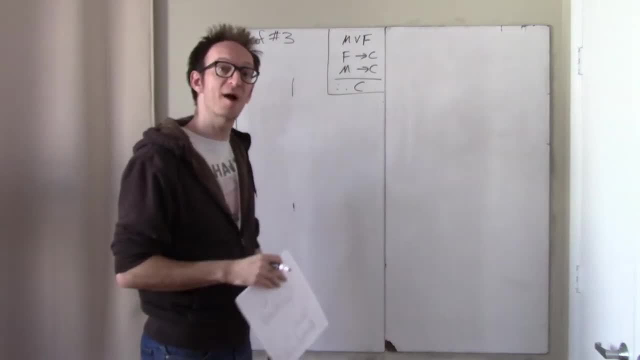 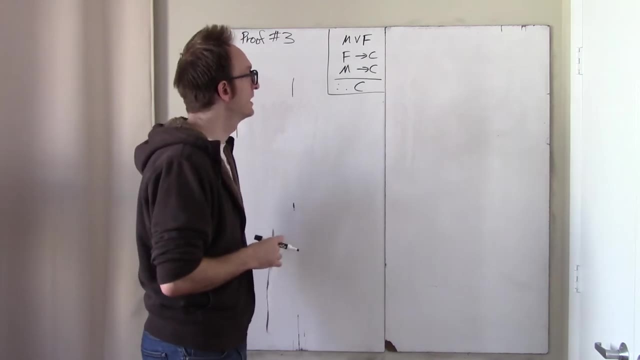 truth table. In this case it would be. you know, we have three propositional variables, so this would require this would require you know eight rows of a truth table and you could just sort of confirm that this is true. But of course no one reasons like: 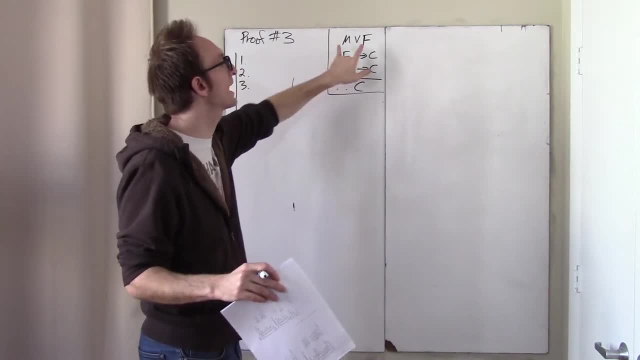 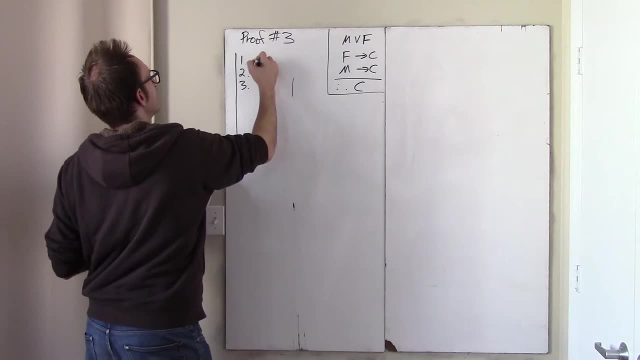 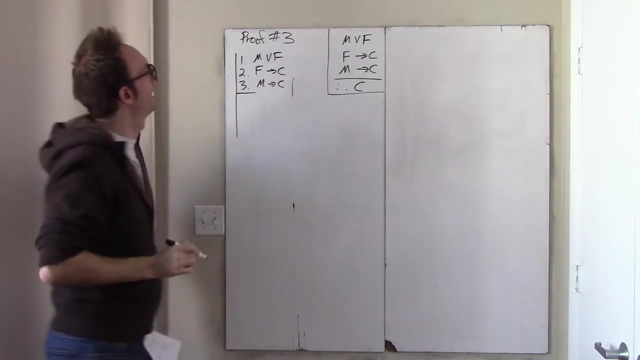 that The way they actually reason is by doing a kind of proof by cases. Okay, well, since one of these must be true, but each of these leads to C, then C must be the case. Okay, and well, let's do it. Yeah, Well, this formal proof system that we are introducing. 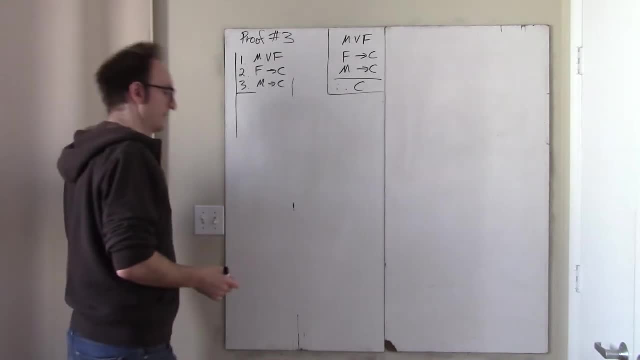 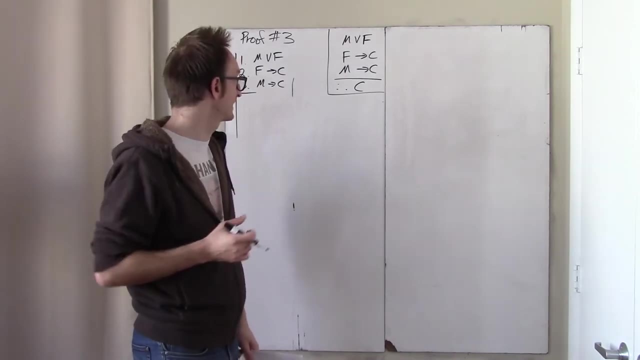 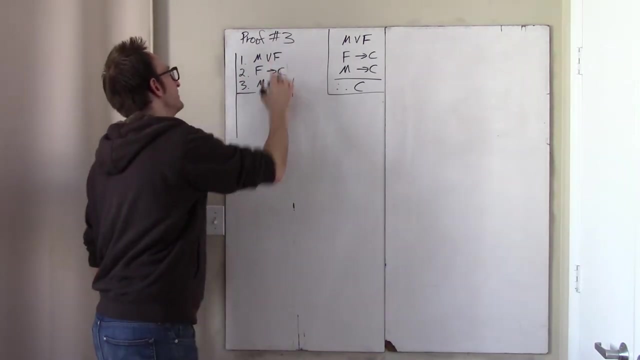 the Fitch-style proof system is a really a. it's Fitch-style is just a kind of style and of indenting and kind of some naming and notational conventions, but they're all overall kind of proof. This is. this is what's called a proof, a natural deduction proof. 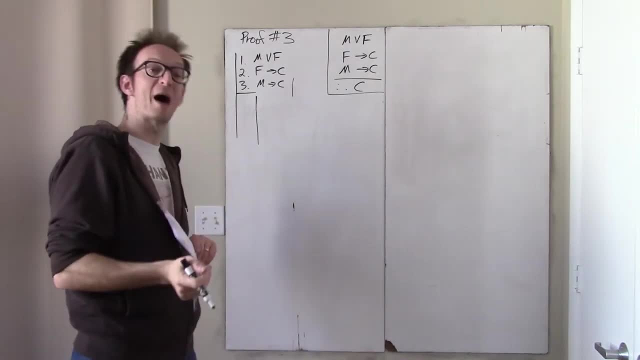 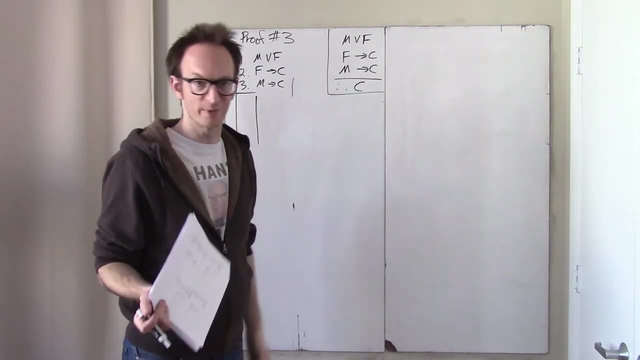 And it's a natural deduction proof in the sense that it's supposed to model the way we actually reason. And the way that we actually reason is not by making a truth table. We don't. no, no one would sort of confirm to themselves that this is a valid argument by 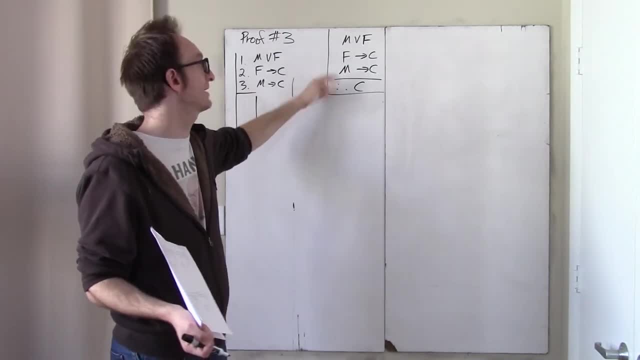 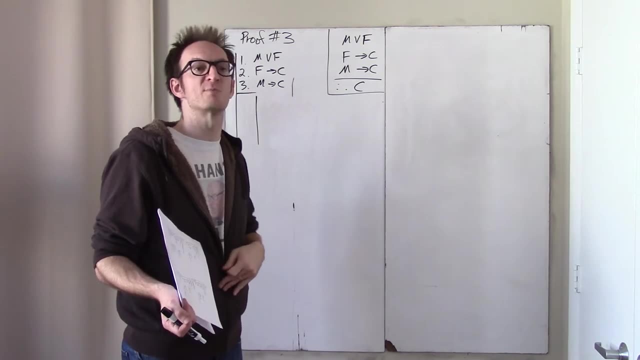 constructing a gigantic truth table and checking every case. Instead, they just perform a proof by cases, as we have just done. And so our we are creating a a a, a formal proof table which models that way of reasoning. So it's by natural deduction. That's why it's called. 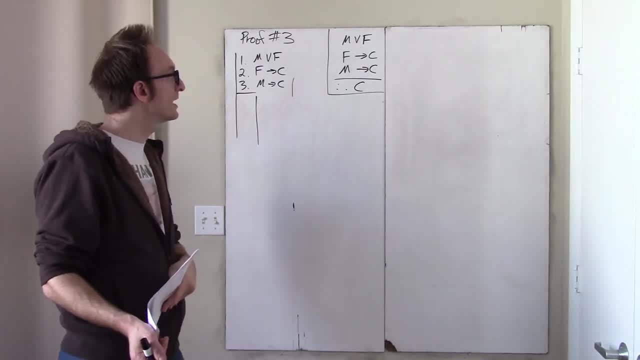 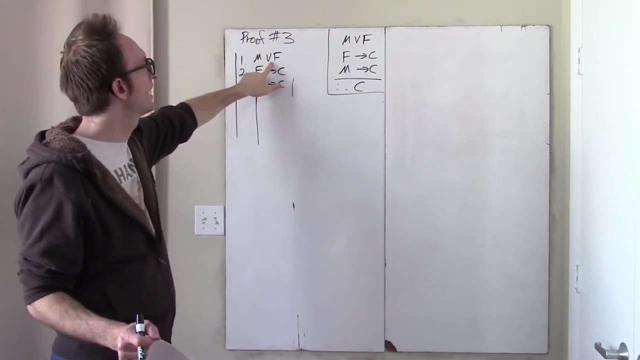 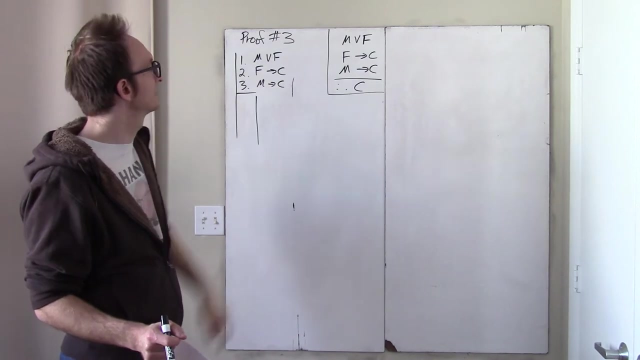 natural. Okay, and so how? how do these natural deduction systems work? They involve, or how does this proof by cases work? rather, If I have this disjunction, then what I need to do is I need to show that both of these cases leads to C, And I don't know. however, 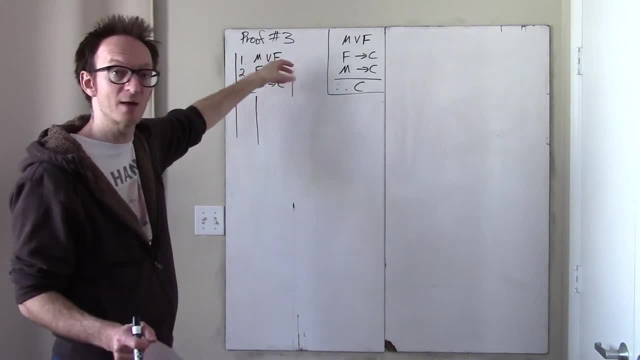 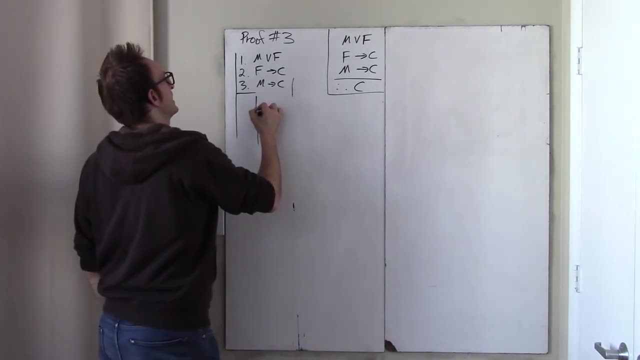 which one of these is true. I just know that the disjunction is true. I have line one or F is true, But I don't know which one of them it is, or it could be both, And so I have to now make a subsequent assumption, And that's what the idea behind this indentation. 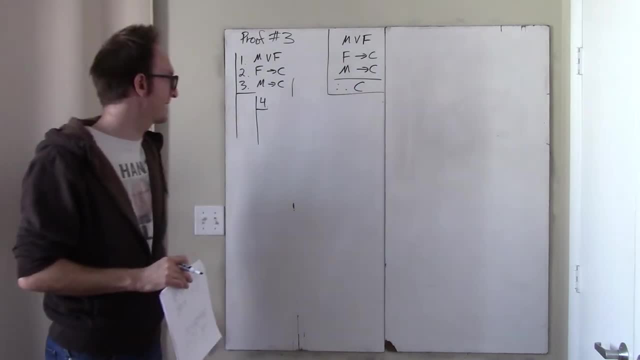 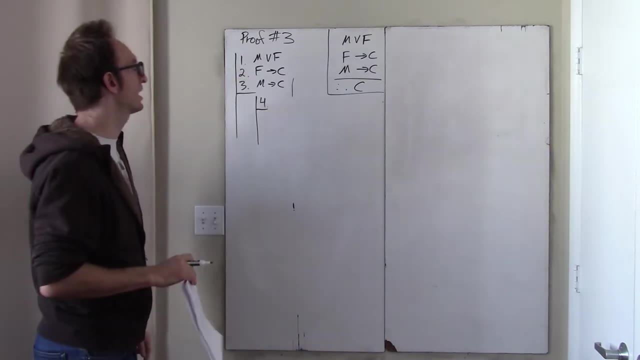 is We indent, when we, when we make another assumption, And and there's this kind of echo of the horizontal bar which separates premises from the body of the argument, Because now every assumption is kind of like a new premise of a new mini argument, And so there's. 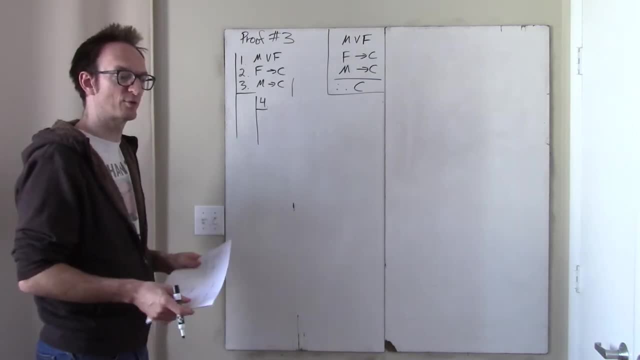 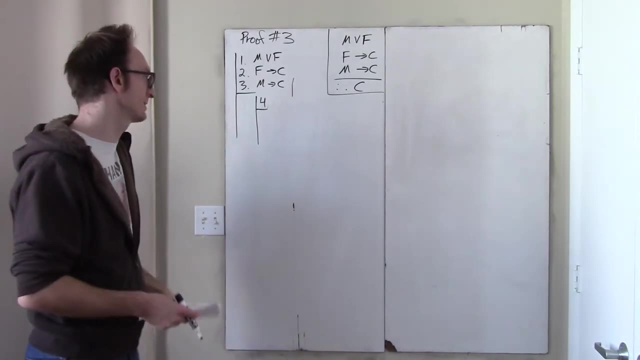 a kind of a fractal nature or something like that. So this proof not fractal, but it's recursive in the sense that I now sort of start a new argument inside of my main argument. That's really the best way of thinking about it. 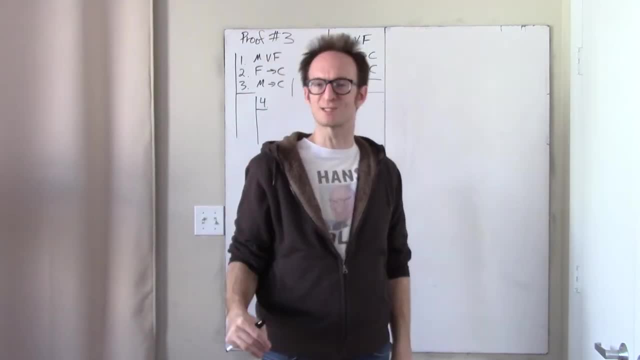 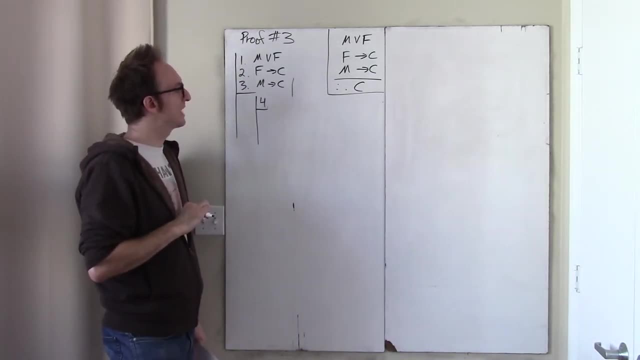 So this, all this kind of stuff that I do know how to teach this. It's just very time consuming to explain all this stuff out. So, anyway, we're doing it by video that no one will watch, I assume I'm. now I reach for this line three, which says: if F is true, 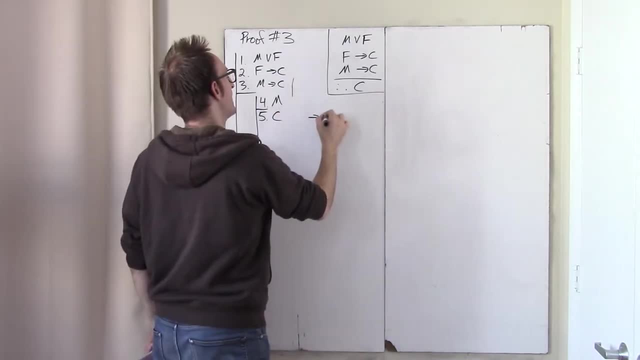 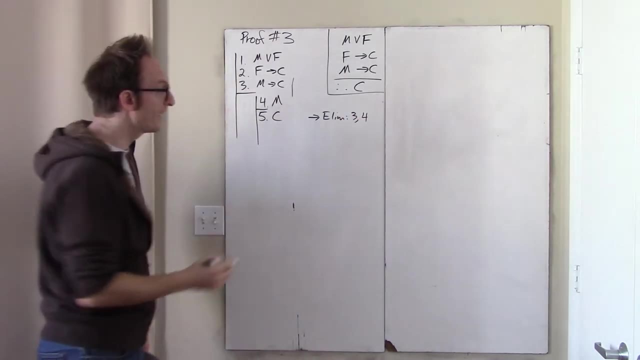 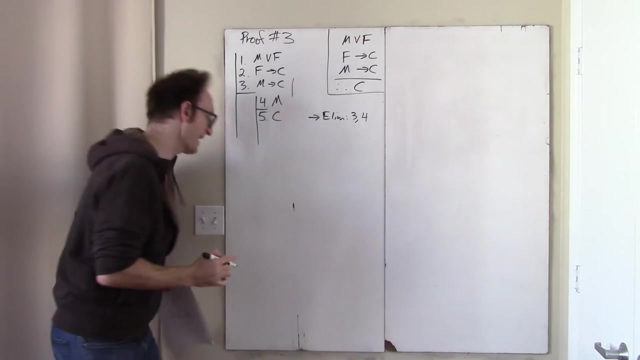 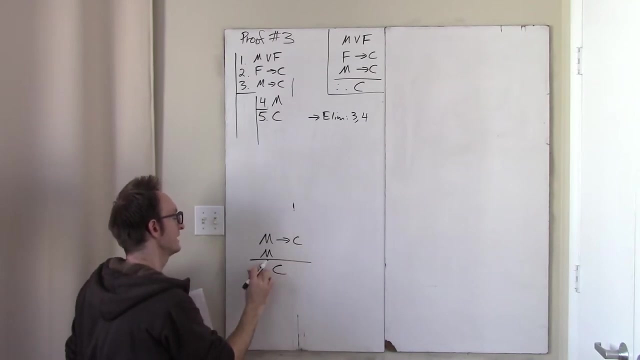 M, then C, And so I conclude C. Okay, this is called arrow elimination, and three, four and well, arrow elimination is just the technical name for modus ponens, And okay, you know here this some of the stuff I did say in class. but ultimately that rule, the rule. 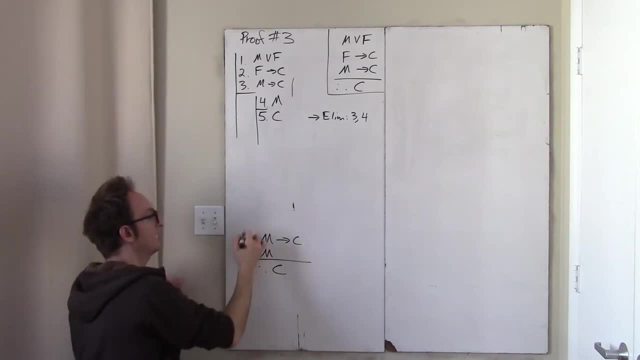 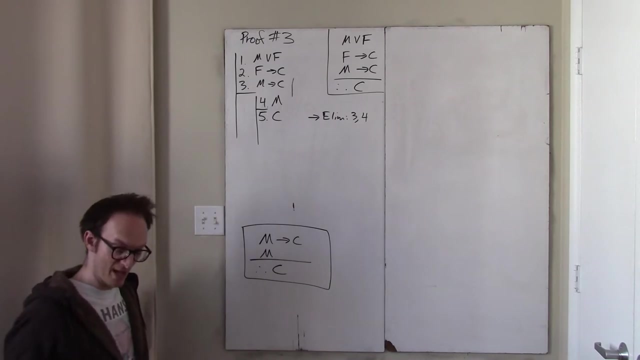 arrow elimination, which I'm using for the first time in this video I'm going to use. it can be thought of as sort of codifying this argument And, once again, this argument is valid. You can convince yourself it's valid by making a truth table and once you've convinced, 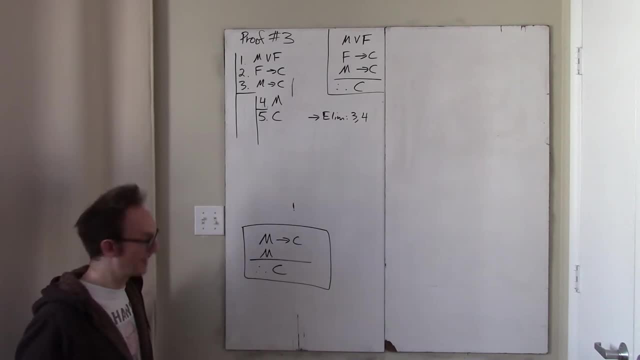 yourself that it's valid, then it's a legitimate rule and we're going to use this rule from now on. But sort of on a deeper level, this rule sort of explains you know what even sort of conditionals are. You know what is a conditional, What is the sort of, what is the sort of meaning or purpose. 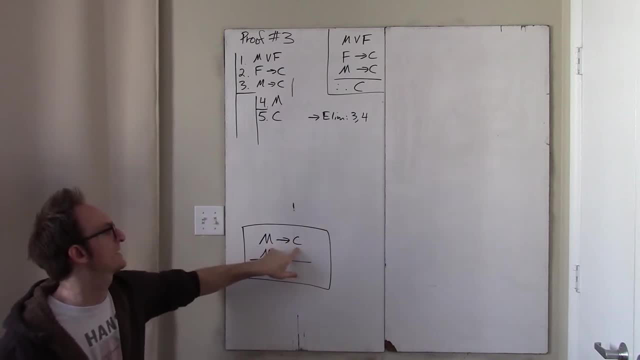 or destiny of a conditional. And the answer is: a conditional tells you that well, if the antecedent is true, the conclusion is true, And so one may, when given a conditional, if you also have the information that the antecedent holds, then you know that the conclusion 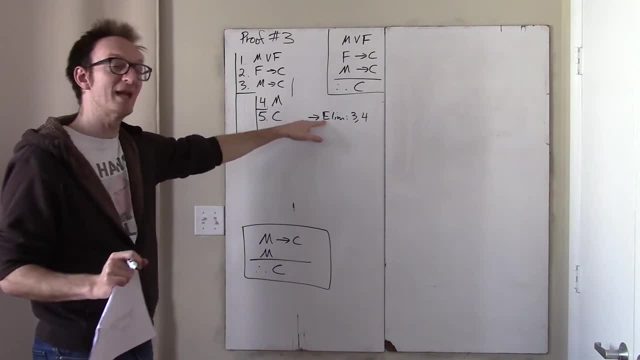 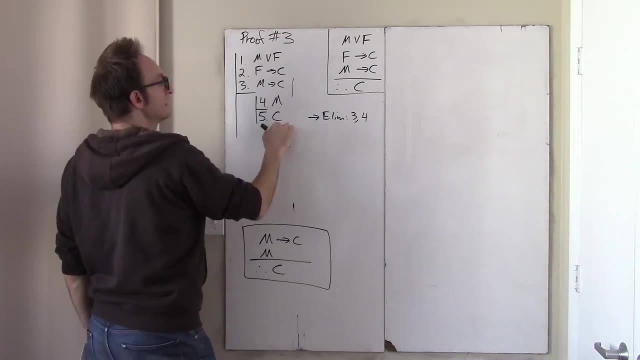 holds, And so this is arrow elimination, in the sense that we eliminate the arrow, We use the arrow, We squeeze information out of the arrow. Okay, and notice that C, I've reached a sort of as my goal here. what was the overall goal of this proof, which? 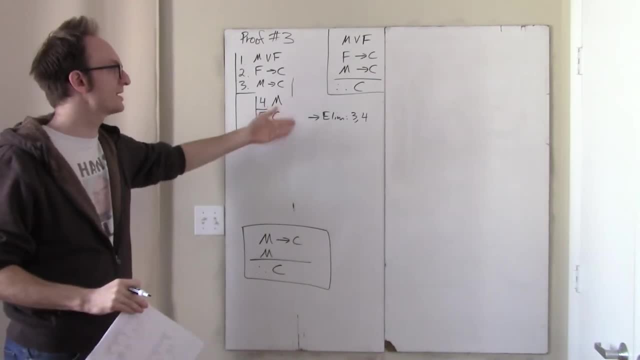 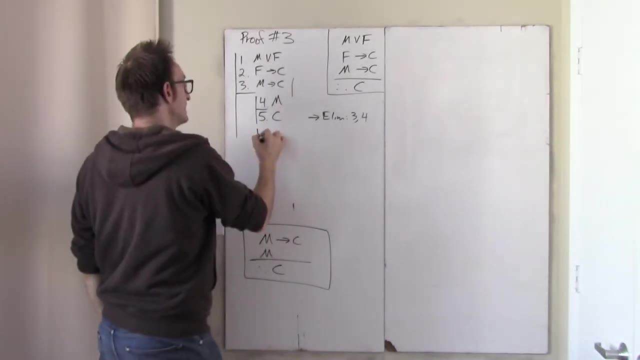 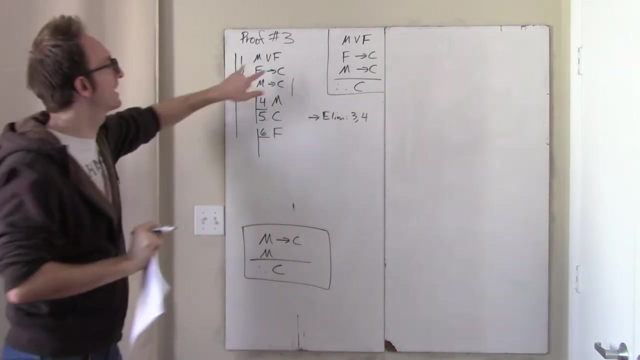 is to conclude C. And so now I've shown it. just took me two lines, or one line. you might say that this M leads to C. Okay, and now I immediately begin with the other half of the proof by cases. So I knew that from line one that either M was true or F was true. 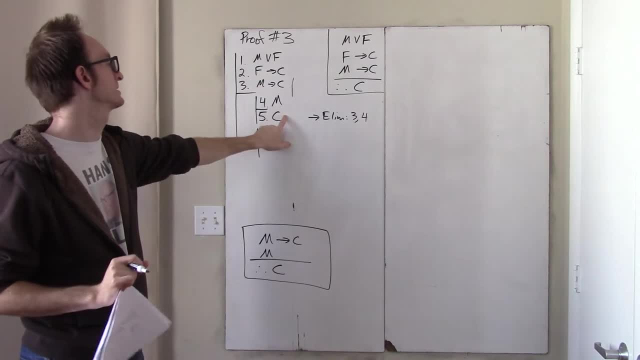 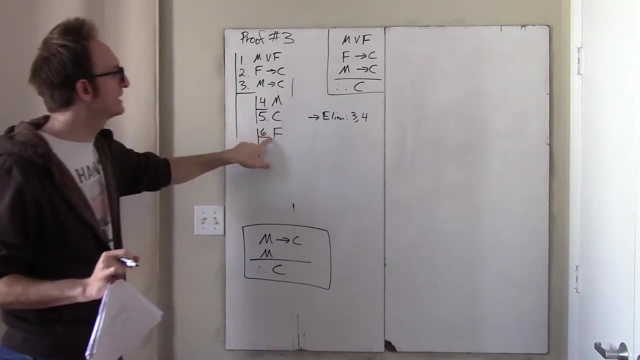 So I assumed, on the one hand M I got the conclusion I wanted, And now I stop. note this break here. I stop that sub-proof, that sub-proof has kind of ended and I begin immediately after it. another sub-proof, And now I get to also conclude. 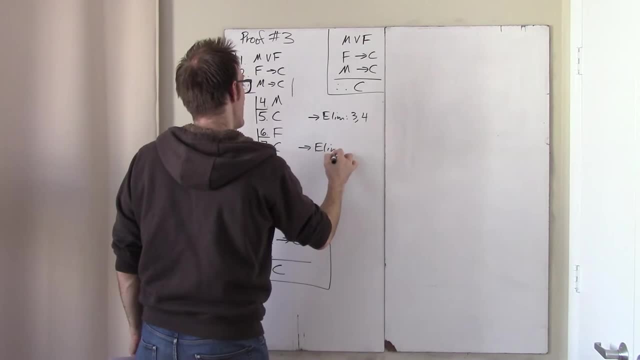 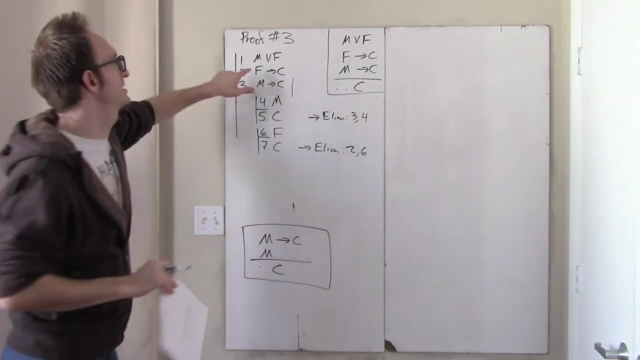 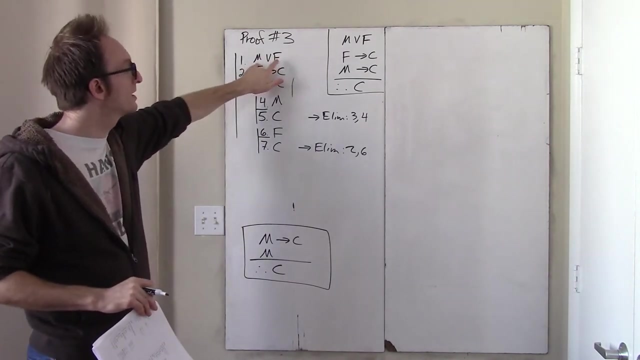 C from this sub-proof reason, arrow, elim, two, six. In other words, I have this conditional: if F, then C, but I know F, therefore I conclude C. And so I've shown, looking at line one, M leads to C and also F leads to C. 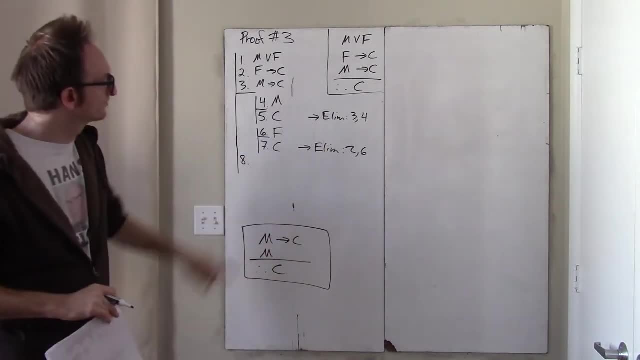 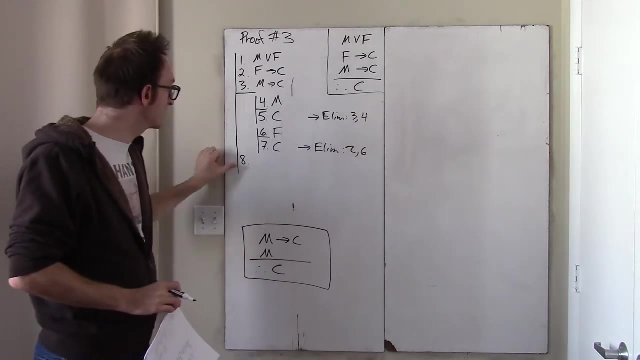 And so, and here's the key idea now I, you know, I de-dent, that might even be a word, I un-indent, and I go back down to the main body of my proof. I sort of I end the sub-proof. 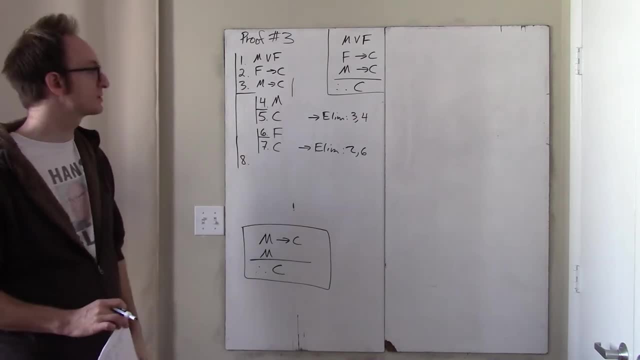 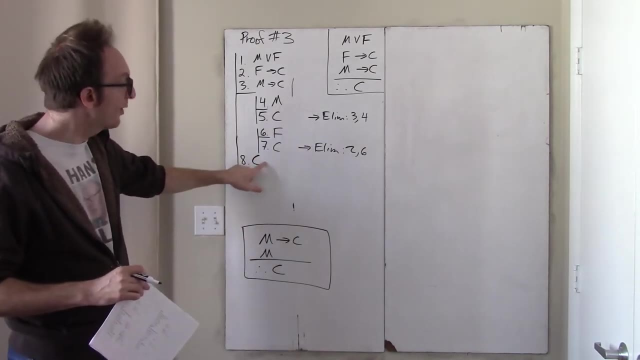 This was in fact sort of two back-to-back sub-proofs, each of which were linked, and I conclude C And okay, intuitively I'm entitled to that conclusion because I showed, by virtue of the sub-proofs in 4 through 5 and 6 through 7,. 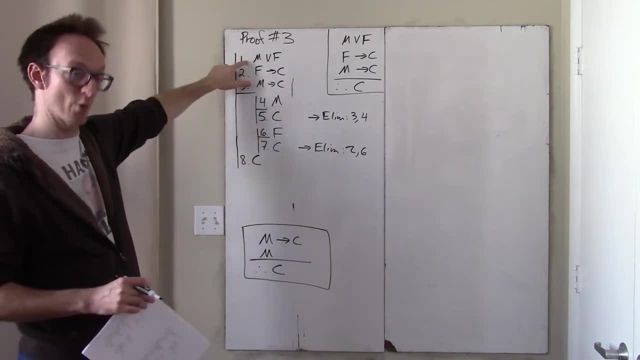 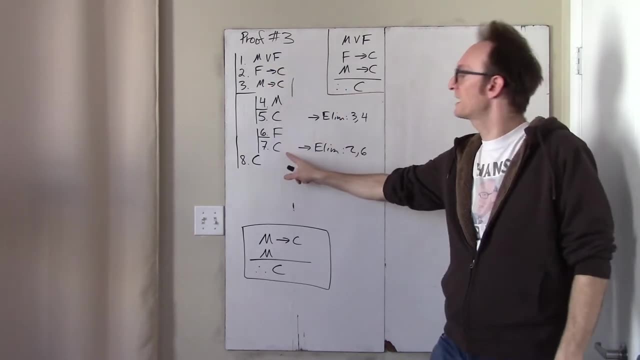 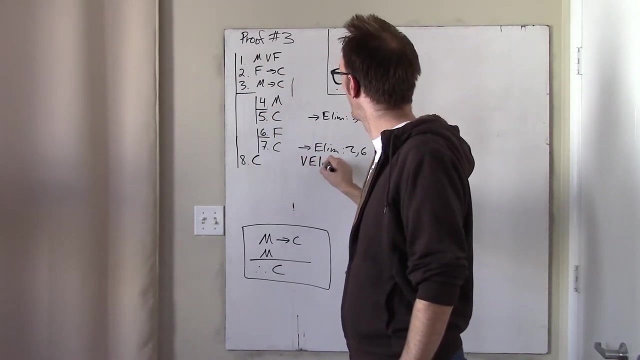 that C is a consequent of line 1.. And it is in fact the disjunction in line 1 which let me engage in this proof by cases. A proof by cases is an exploration of a particular disjunction, and so this rule which is called or elimination. 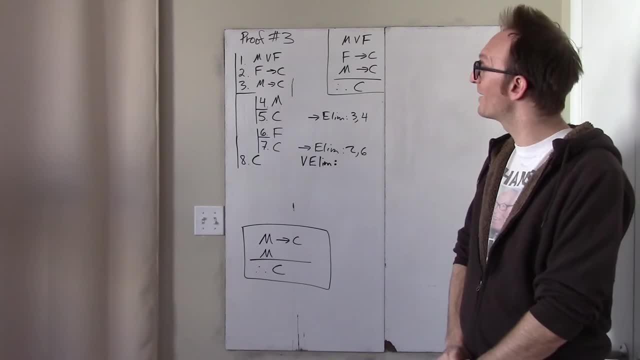 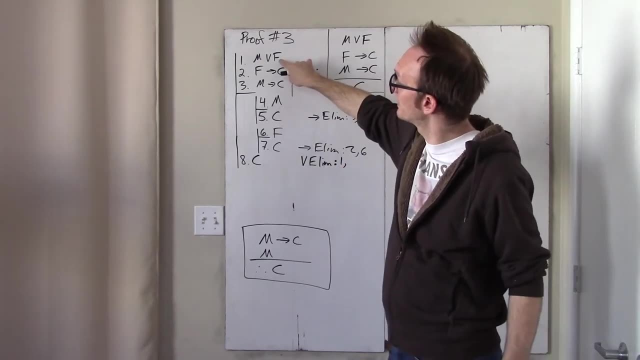 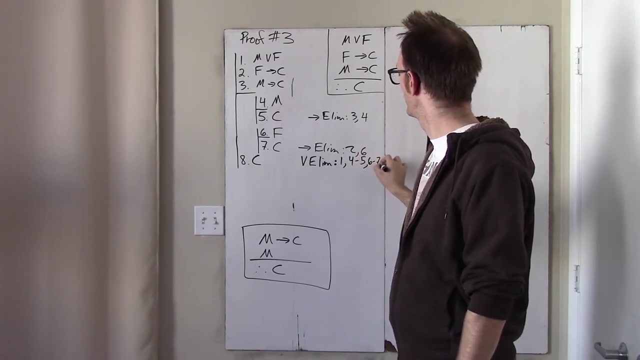 is a way of squeezing information out of a disjunction, And the notation here is one: you note the line number of the disjunct that we're eliminating and then you, you do the. you list the line numbers of the sub-proofs. 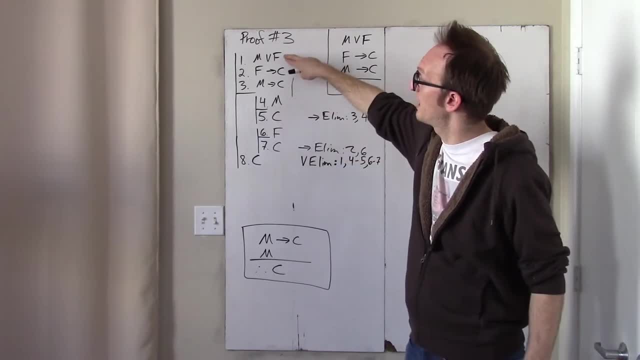 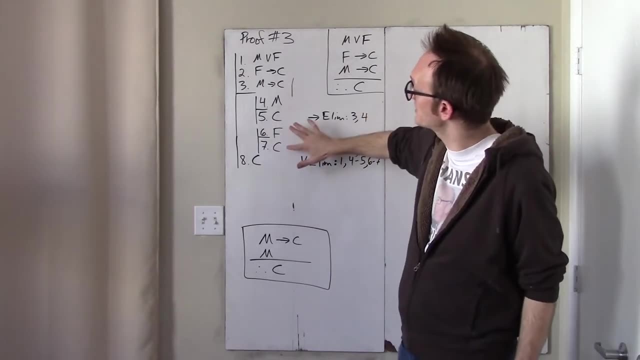 the back-to-back sub-proofs in which you explored that disjunction, And the formal nature of this rule says that you have to conclude each of these sub-proofs with the same and if you reach the same conclusion in both sub-proofs. 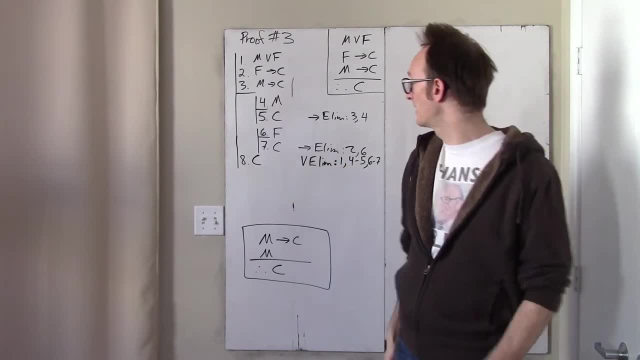 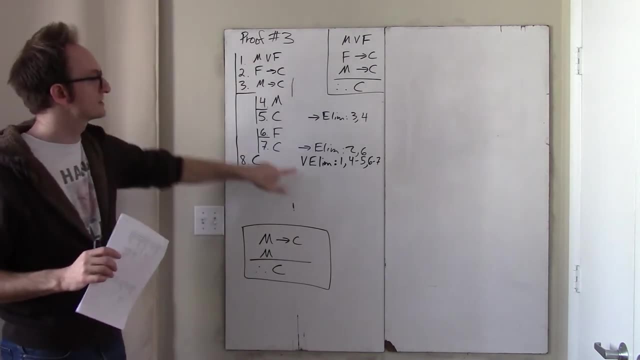 then you're entitled to assert that conclusion back in the main body And you should think of line 8 as really being sort of the result of line 1.. And that's the sense in which it's an or elimination of line 1.. 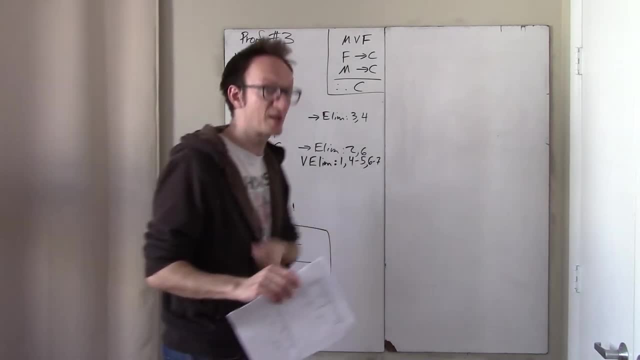 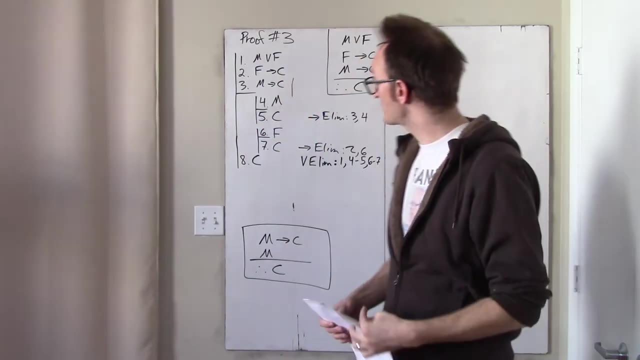 We're eliminating this disjunction. We're eliminating the disjunction by using it, by exploring it, by squeezing information out of it, And, in fact, that just this just is the way to use a disjunction, The only way a disjunction can possibly give you any kind of power. 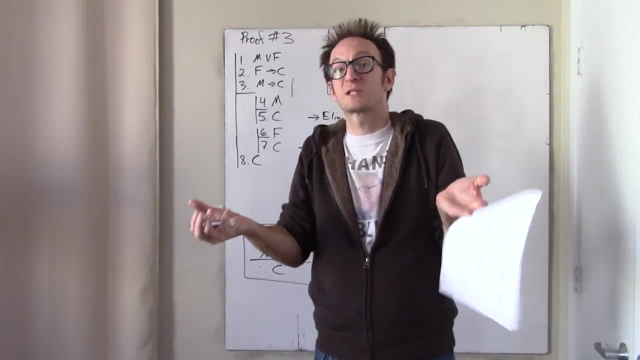 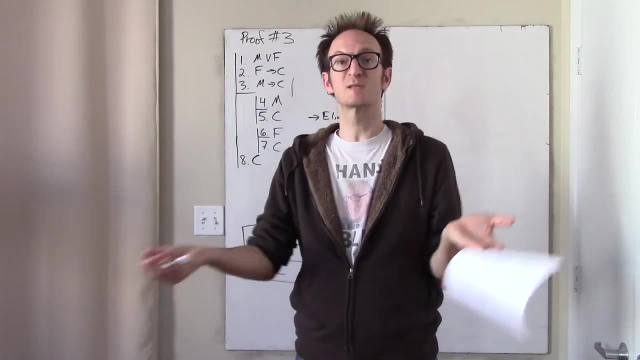 if I know, you know P or Q. the only way to explore that, to use that piece of information, is to sequentially explore each of the disjuncts, Since you know one of them must be true if they both lead to the same path. 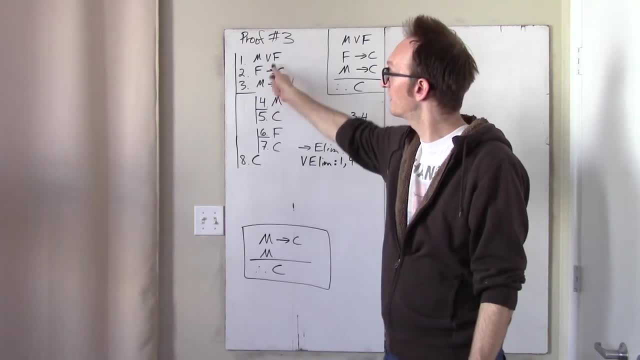 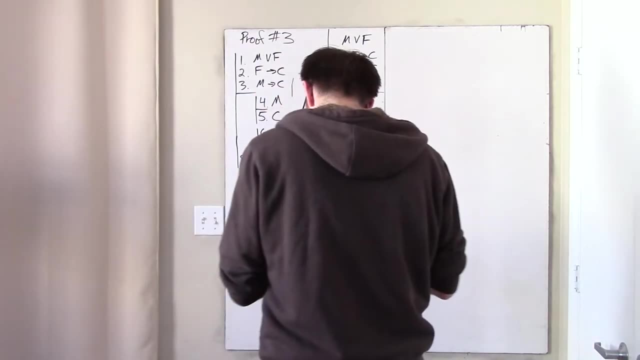 then you can be sure that this line 8 must be true. Okay, alright, going very slow, but you know, for someone who doesn't know anything, this is maybe the the right approach And for the for my own students. 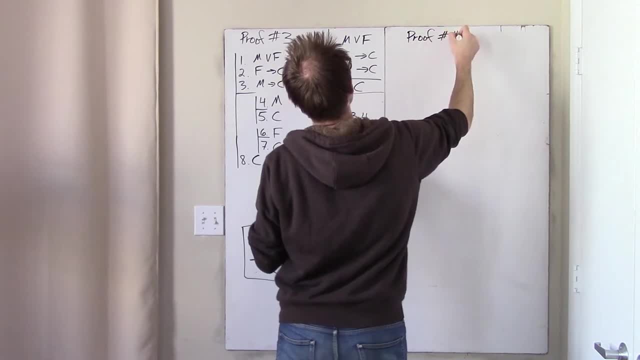 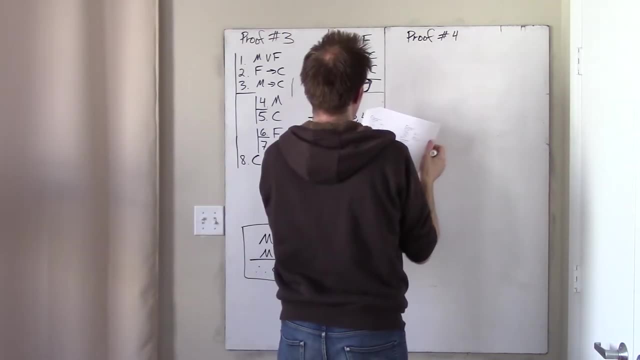 you're either not watching this at all, or you're watching this on two times speed, or you know maybe more. Now I think I have less to say, so I'm just gonna just do a bunch of these. So here we go. 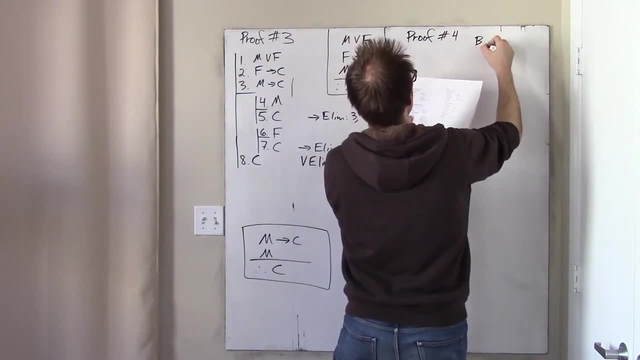 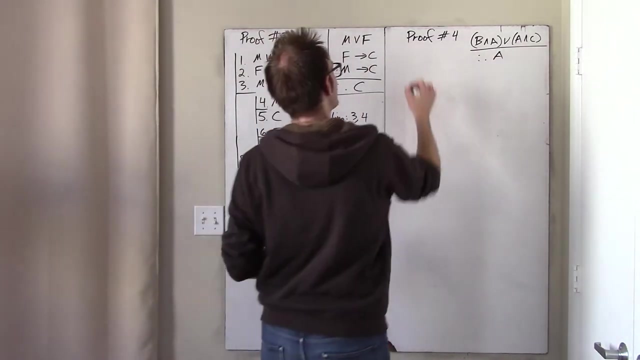 Here's an argument. The argument is B and A or A and C And that, if that's my premise, I conclude A Okay, I want to show that this argument is valid. how I'm gonna do a Fitch style proof. let's go. 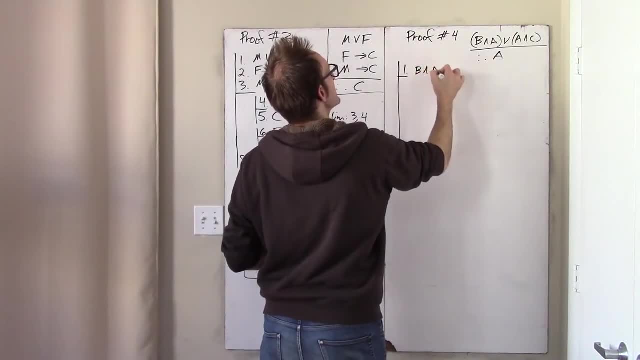 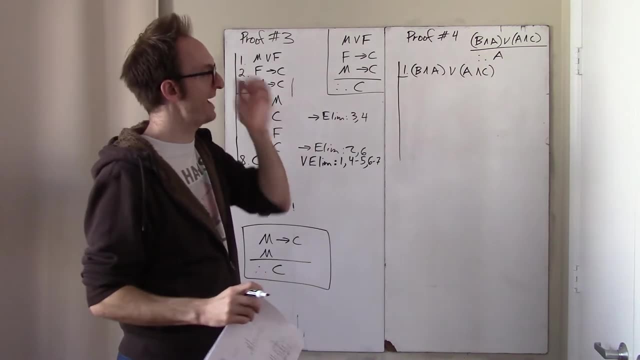 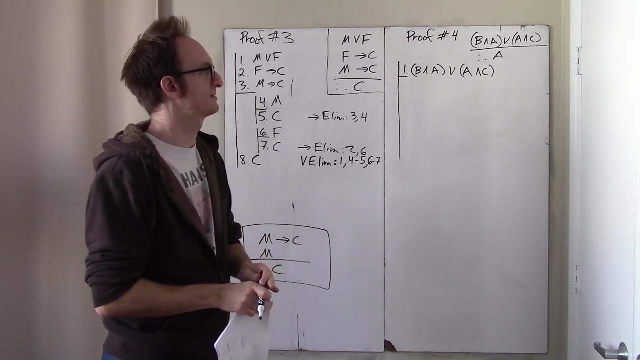 So line 1, I have B and A or A and C. I think this is how I should have made this packet. actually, I should just sort of like list at the top of every page an argument and have you show that it's valid. 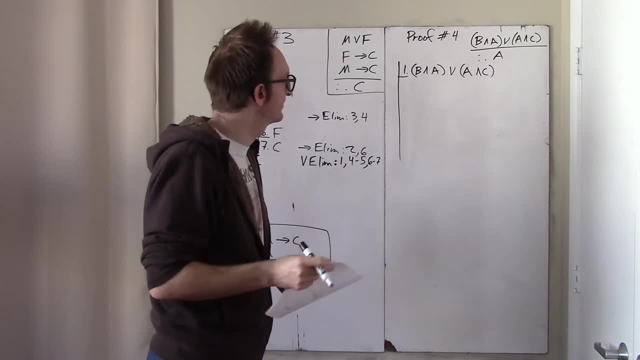 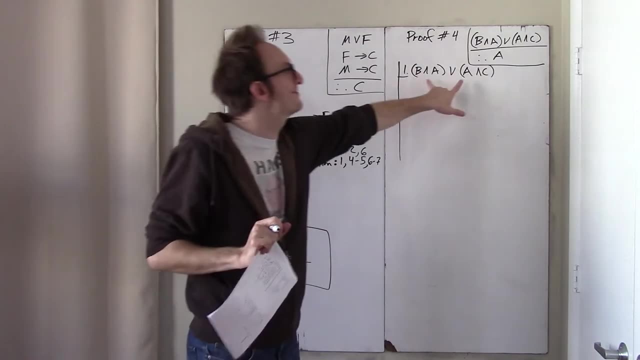 I think that's a better way of putting it. Maybe I don't know. Anyway, we begin. This is the. this is the sort of goal up here. What should I do? Well, I have only a disjunct. 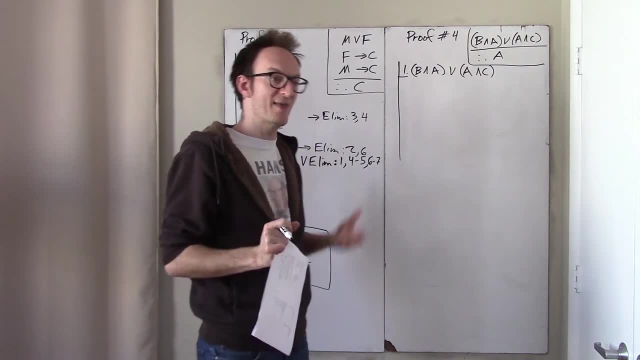 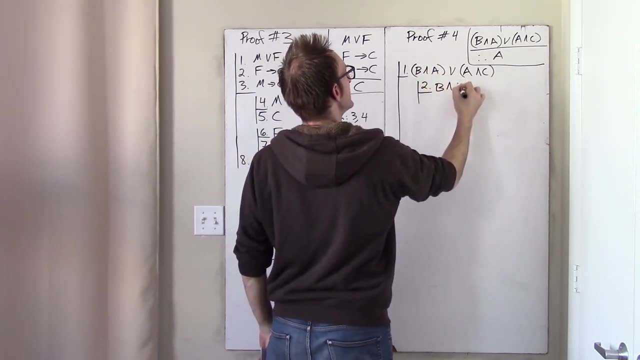 So there's only really sort of one thing to do with a disjunct, and that is to do a proof by cases, And so what I'm gonna do is indent, assume on the one hand B and A, but okay, now this just becomes silly, right. 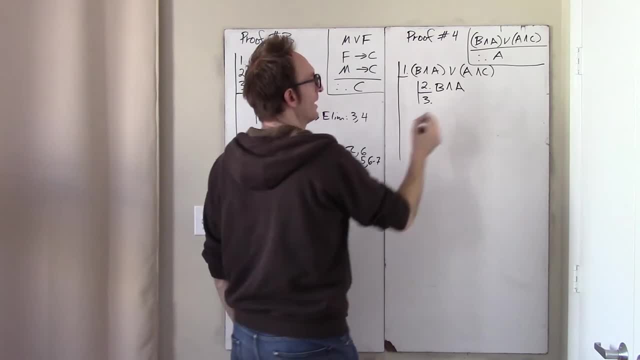 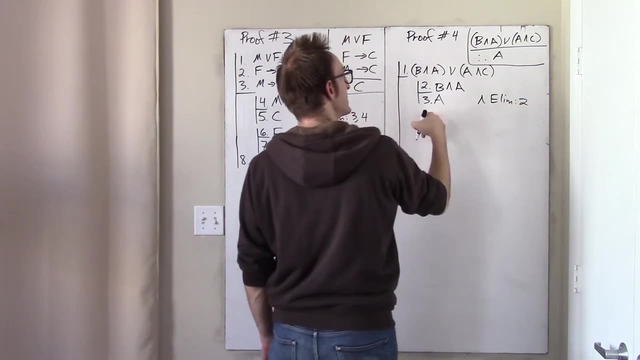 Because from B and A, of course, I know A, which is the only sort of relevant one to me at the moment: reason and elim 2.. But on the other hand, I end this sub proof because I got what I wanted. 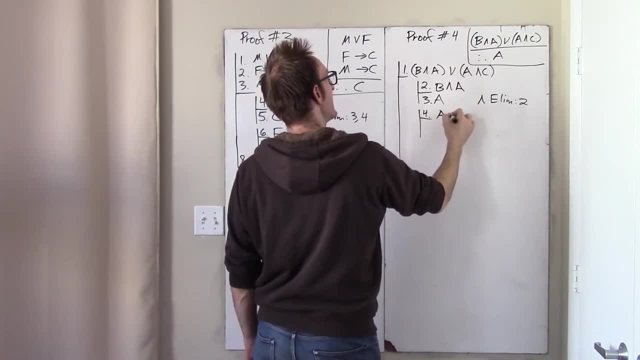 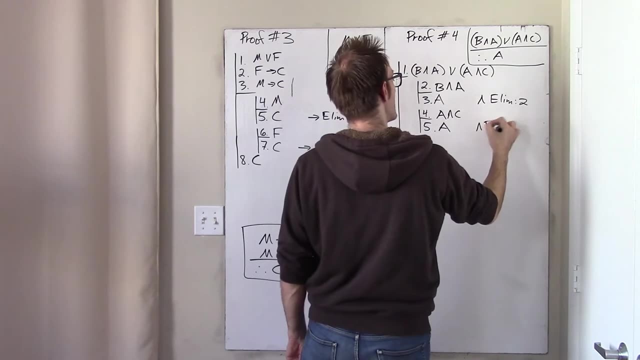 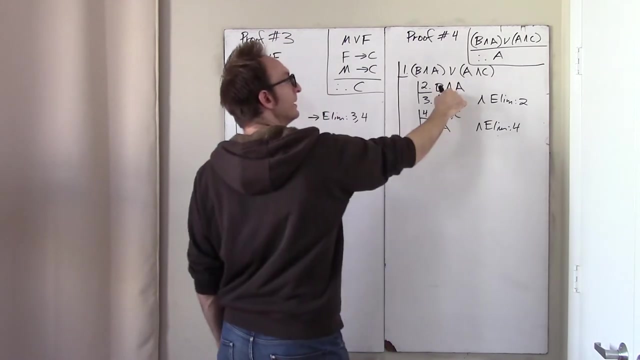 On the other hand, I know I assume A and C, the other disjunct, and from that I conclude A reason, and elim 4.. And okay, there it is right. I looked at each disjunct. 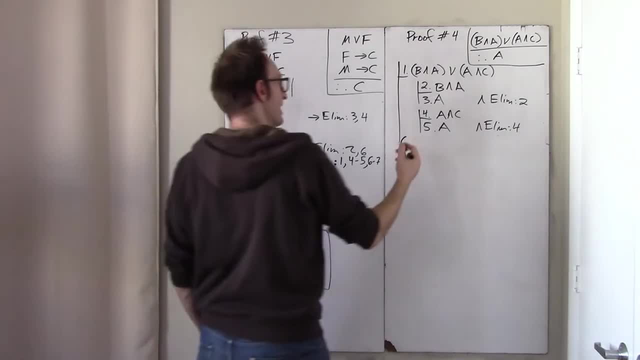 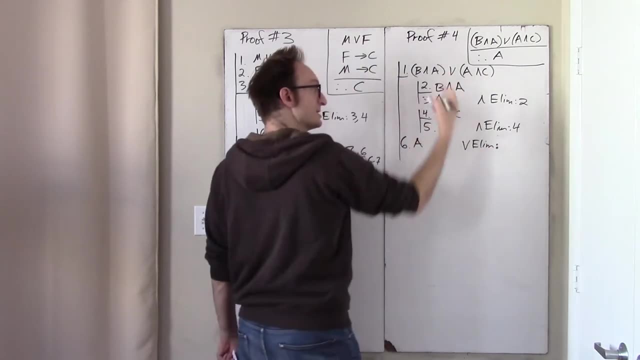 Both of them led to A. So I conclude: A reason or elimination. I began with a disjunct. That disjunct was line 1.. I explored it first in lines 2 through 3, then in lines 4 through 5,. 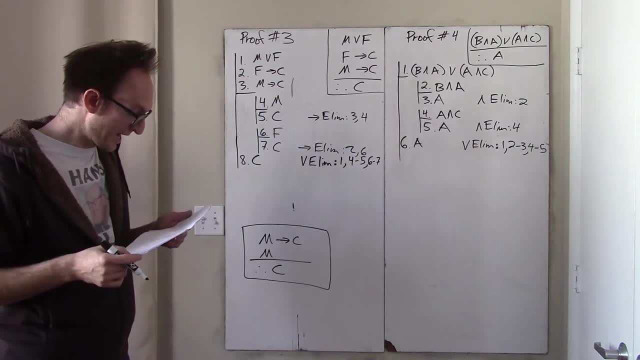 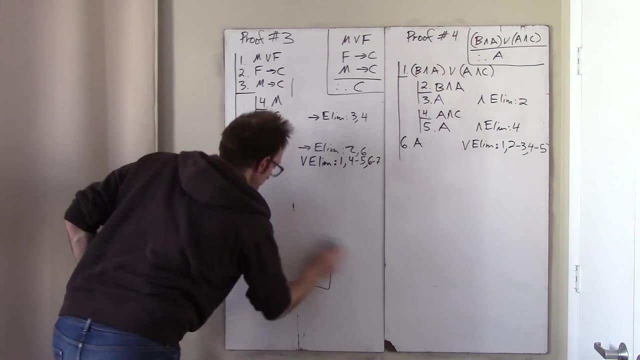 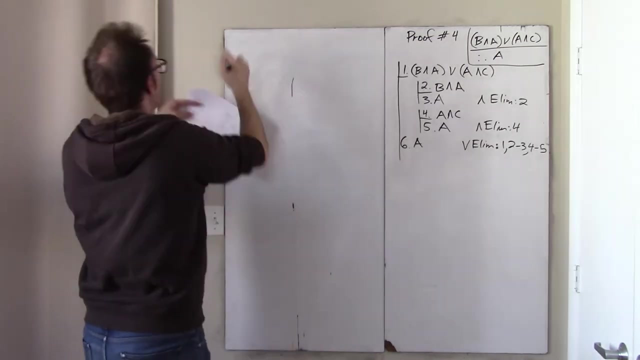 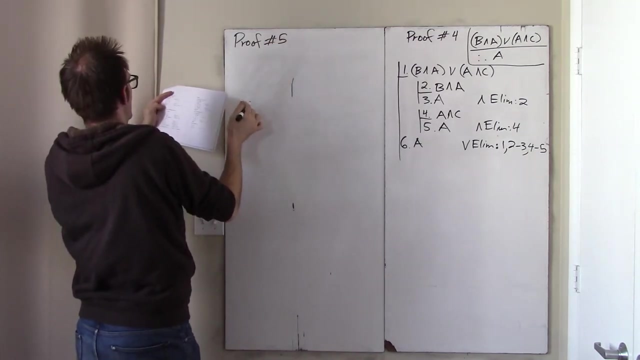 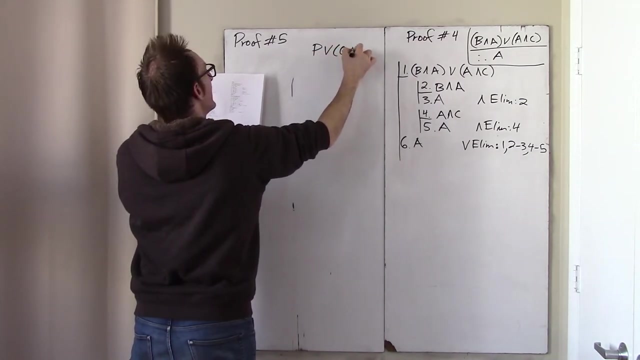 and so I proved A. Okay, good Woo, Let's keep going. Proof number 5.. Oh yeah, Okay, here we have premise P or Q and R, And from this we would like to conclude: P or Q and P or R. 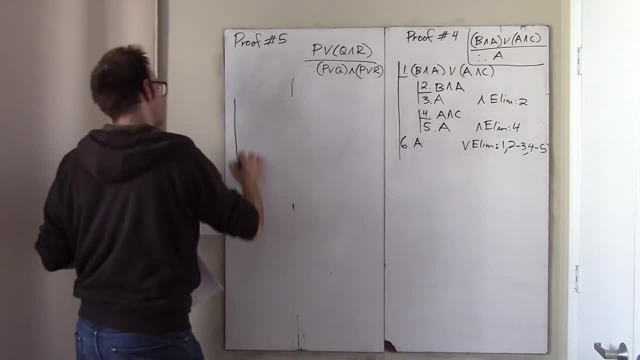 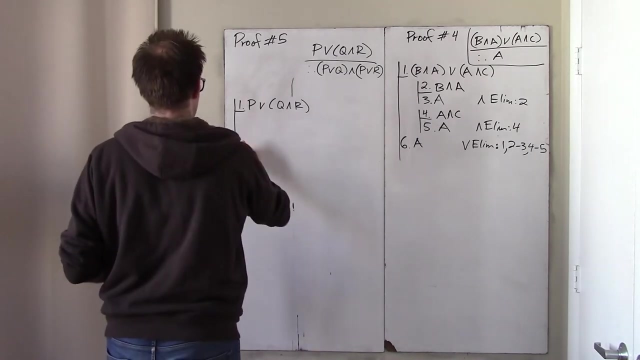 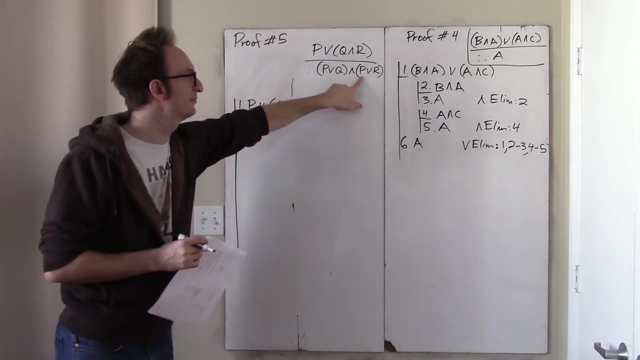 Okay, let's begin. My first line is P or Q and R. Let's see what I can do Well here. well, okay, let's sort of just maybe start. I think this is actually still pretty easy, because I have this thing that I'm trying to prove. 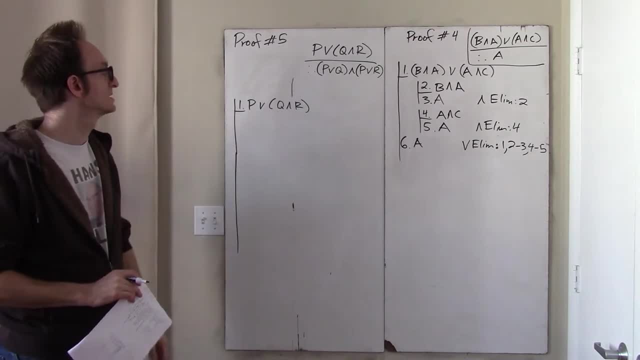 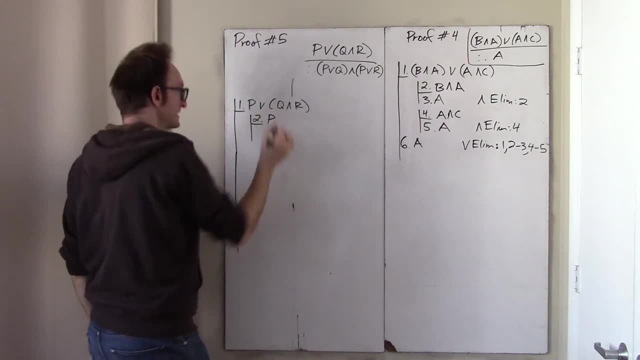 and I have really only one thing to do now, which is to prove by cases. So I'll just begin my proof by cases. This is a disjunction. On the one hand, it might be the case that P is true. Well, does P entitle me to this conclusion? 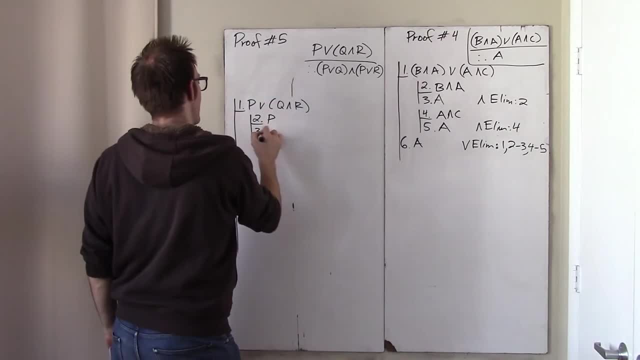 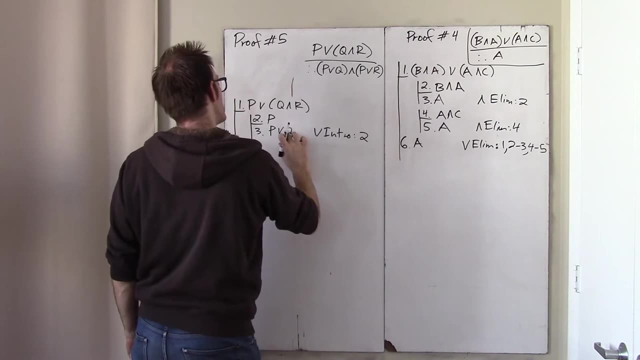 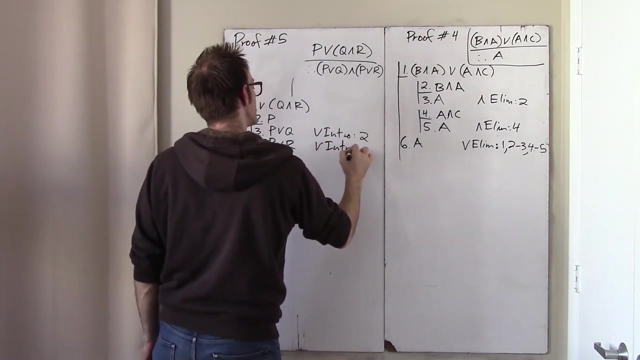 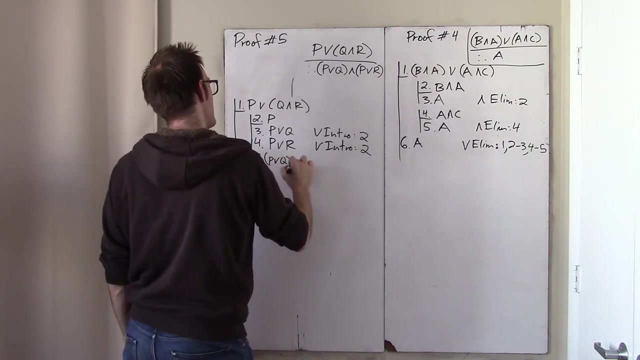 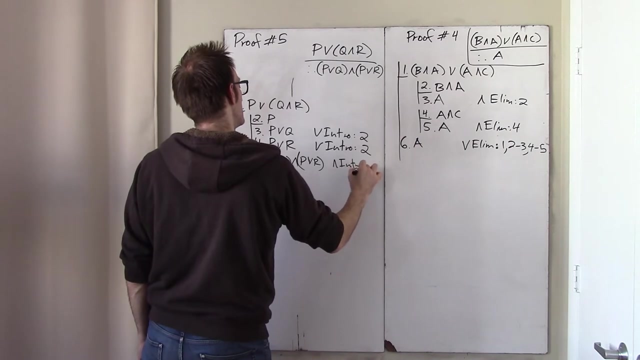 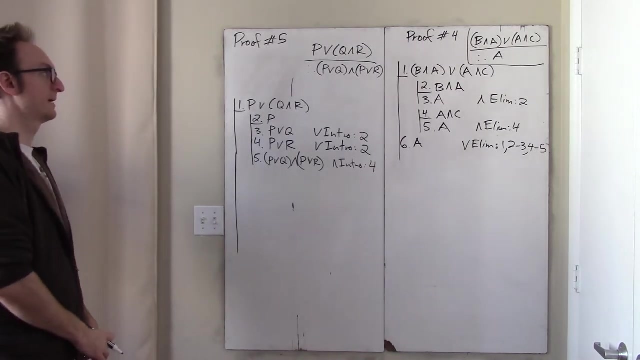 Yes, because I may, or on this Q by or intro line 2, I can then or on R, and that's also or intro 2, and then I get P or Q and P or R reason and intro 4, and that's what I wanted. 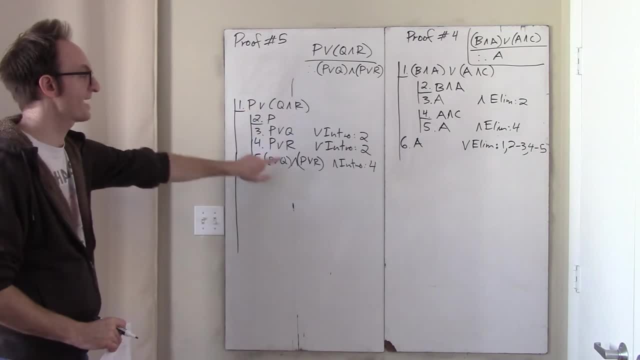 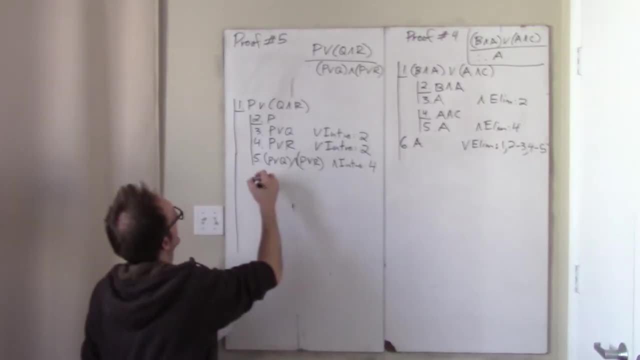 So I showed that my left disjunct P does in fact imply this, which is just kind of makes complete sense if you think about it. Okay, well, what about the other possibility? What if it was Q and R that was true instead? 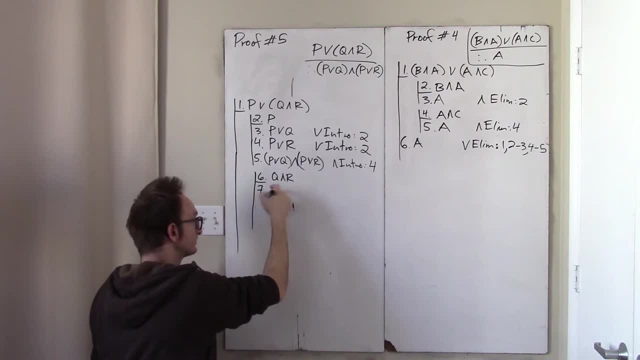 Well then, I can still do this right, Because I can get Q and I can or P onto the front of Q. On the other hand, I can get R and I can or R on or I can- sorry, I can- or a P onto the other side of R. 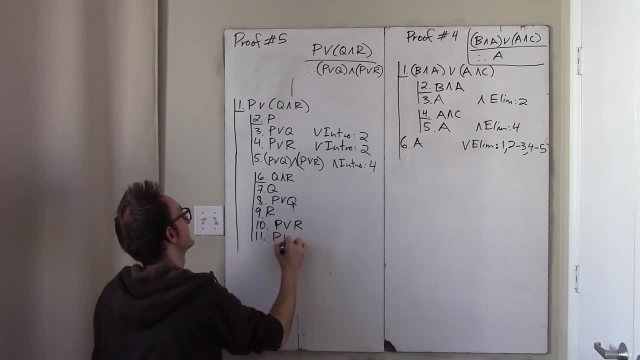 and then I can and them together, So P or Q and P or R. Okay, so here I did it to notate and here I go, So I'll sort of explain myself now. This is and elim 6.. 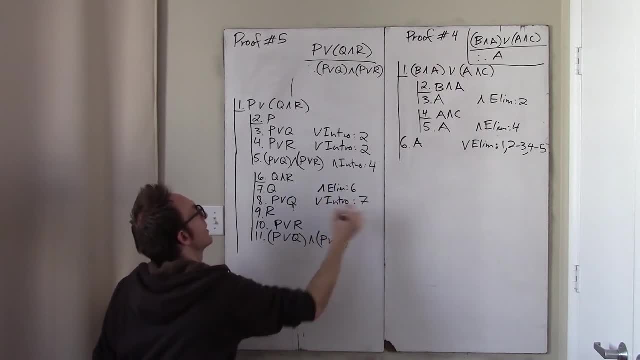 This is or intro 7.. So I just I weakened my line 7 by or-ing it together with a P, and sure you can put it up on the front like this, because we want that kind of power and it doesn't matter. 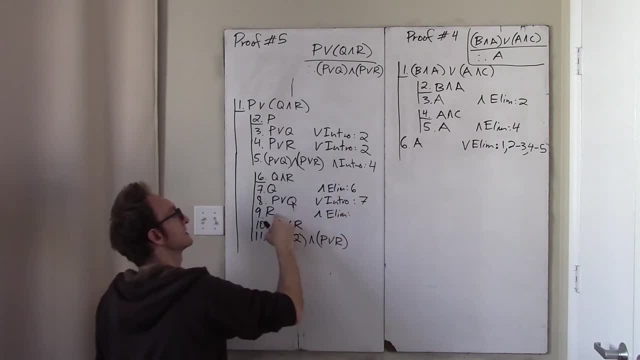 Here we have. this is also this. line 9 also just comes from line 6.. Once again, I sort of weakened my line 9 by or-ing a P onto the front. and finally this line 11 is, and oh, I guess I should squeeze it in here. 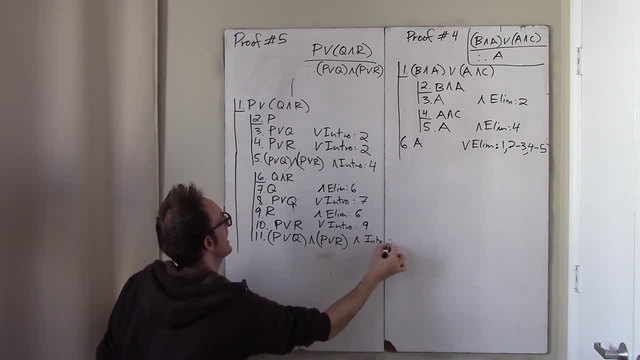 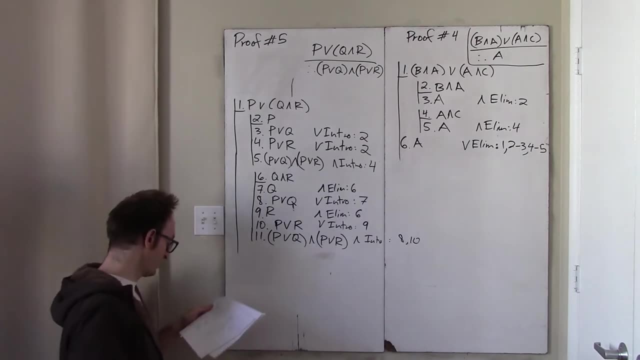 need a better board situation and intro 8 and 10.. Yeah and well, now I have finished my sub-proofs. I've showed that my left disjunct leads to my conclusion and then my right disjunct leads to my conclusion. 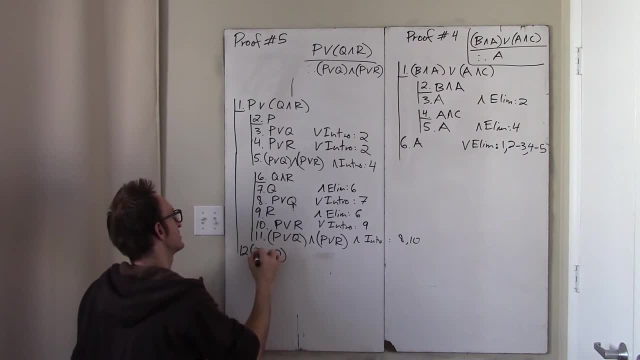 Thus I just have my conclusion, And so you're not sort of done with the proof. This kind of goes without saying or something. but you're not done with the proof until the thing you're trying to prove is out at the most sort of de-dented line. 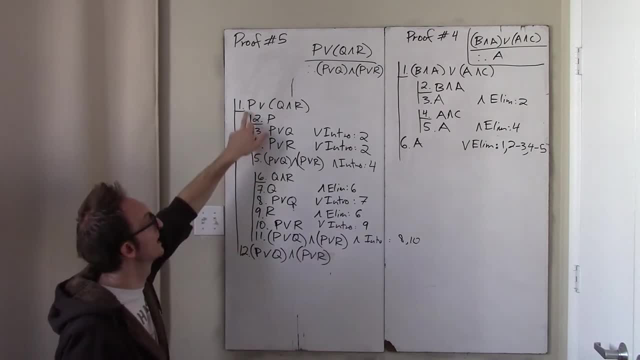 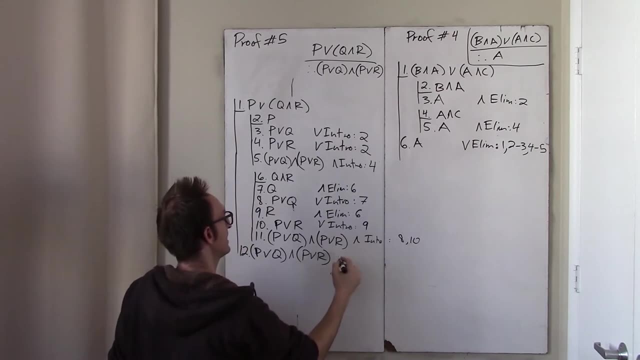 back at the main bar of the proof, so to speak, at the same line as the as the premise. I think that maybe goes without saying. Okay, what's the justification for this? It's an or, elimination and the disjunction that I eliminated. 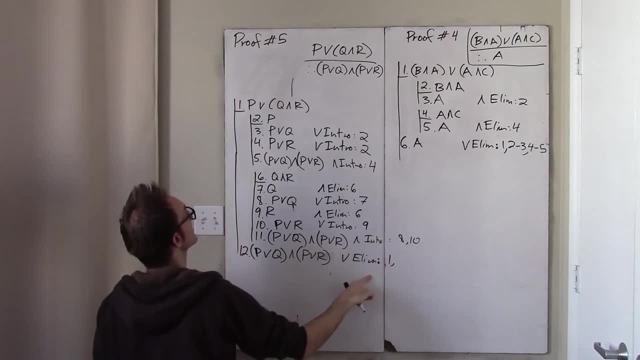 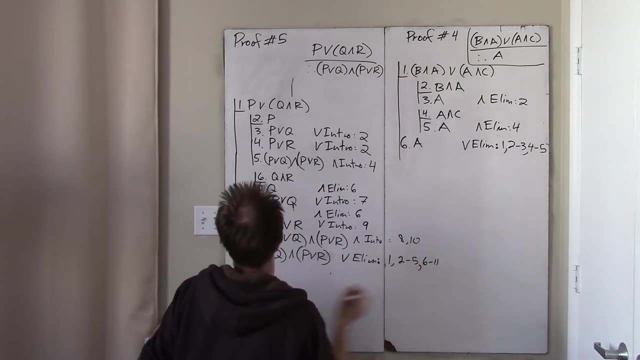 was the disjunction in line 1, and I did it via two sub-proofs: a sub-proof that went from line 2 to line 5, and a sub-proof that went from 6 to 11.. Okay, so that one was maybe a little bit harder, or something. 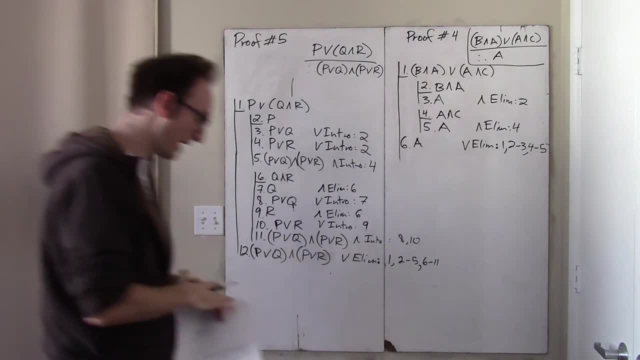 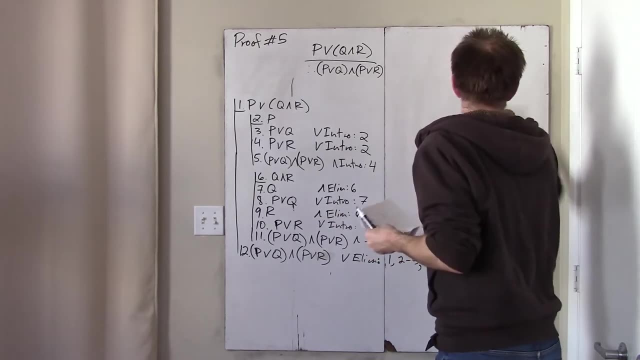 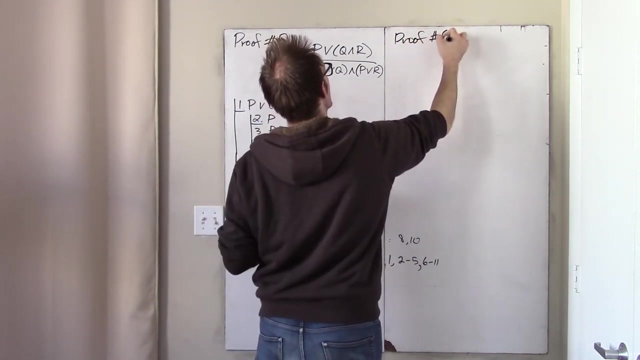 but really not Okay. then come sort of three proofs that are bordering on, you know, silly. Well, let's just, let's not disparage the proofs, Let's just do them. So that was proof 5.. 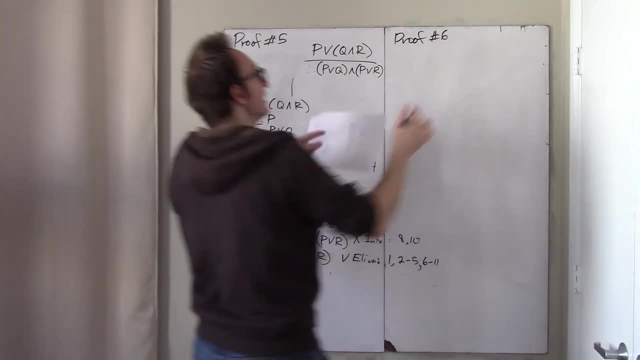 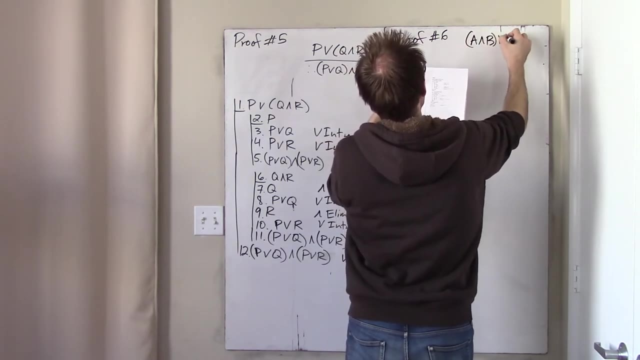 This is proof 6.. What's proof 6?? Well, this is really just more practice, right? The argument now is A and B, or C and D, And from this I would like to conclude B or D. Okay, that seems pretty reasonable. 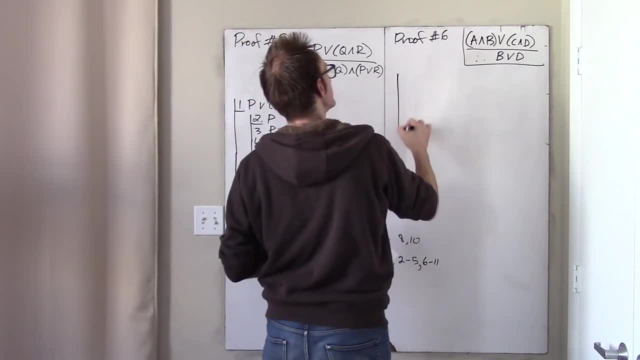 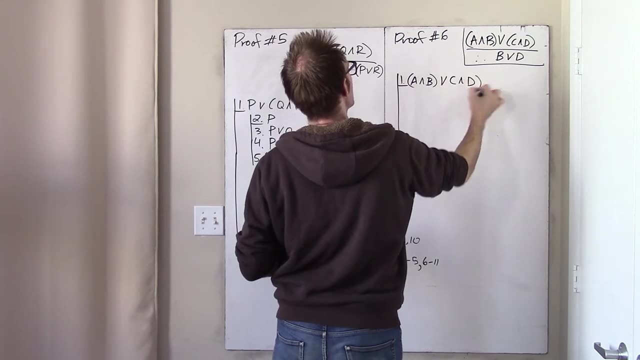 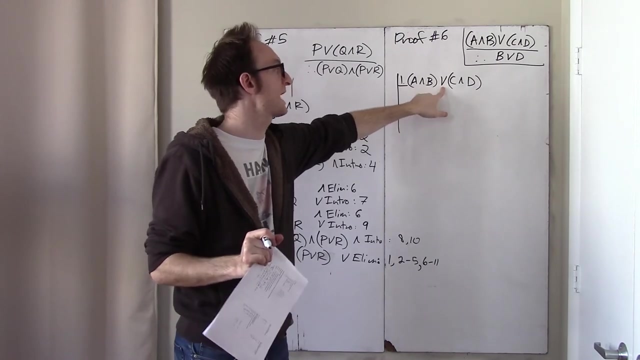 Actually very reasonable. Okay, so we begin My premise: A and B or C and D. Once again, the main connective in this proposition is, or so the overall. this line 1, is a disjunct. 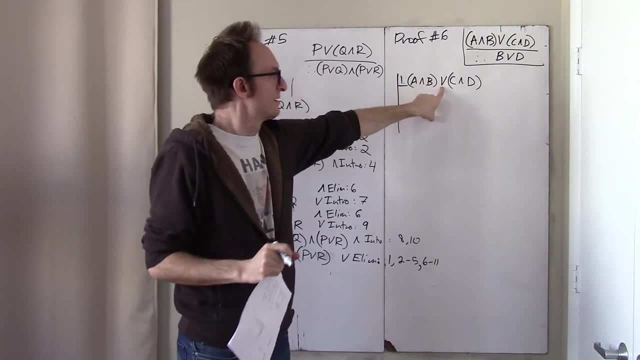 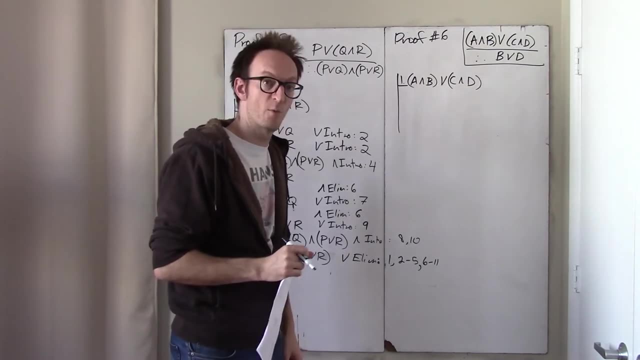 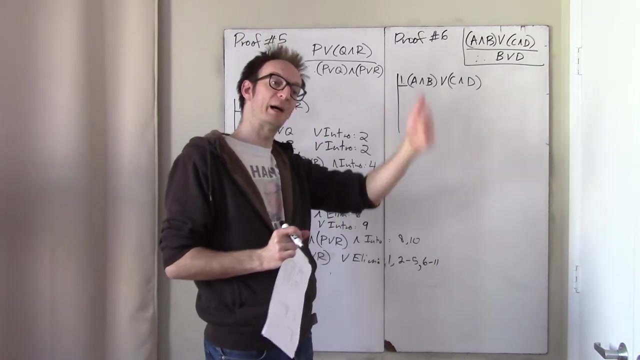 What I mean by main connective is sort of the connective which is kind of syntactically, you know, governing this sentence. What counts as a well-formed formula of propositional logic is defined recursively by applying the rules allowing you to add two propositions together. 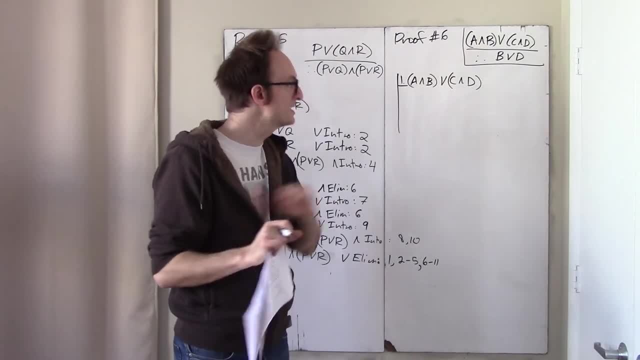 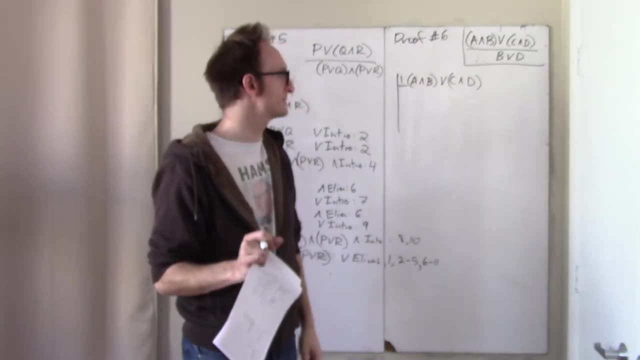 with a connective, in the middle or wherever the connective is. So here there's got to be some rule which says: hey, if you have a proposition X and you have a proposition Y, then X or Y is also a legitimate proposition. 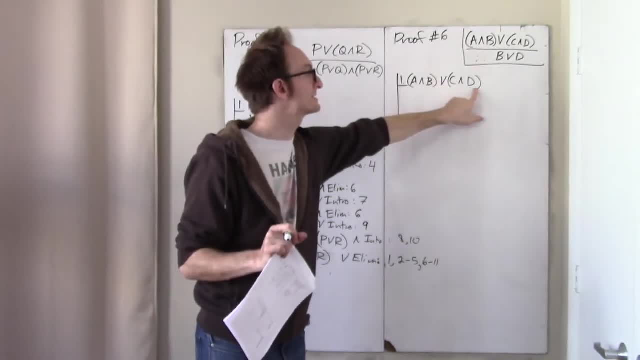 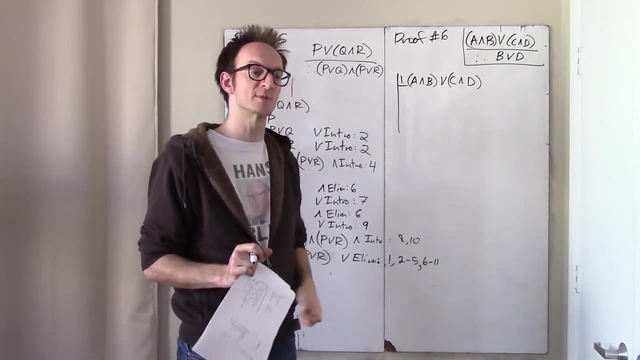 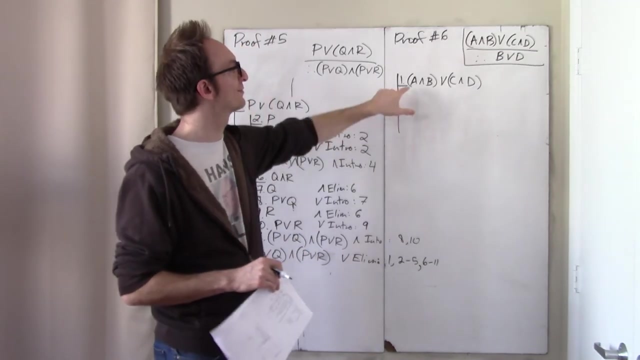 And so it's the sort of. it's the last application in the recursive definition of what makes your formula syntactically well-formed. that determines sort of what you are. The main connective here is an or, and therefore you need to sort of. 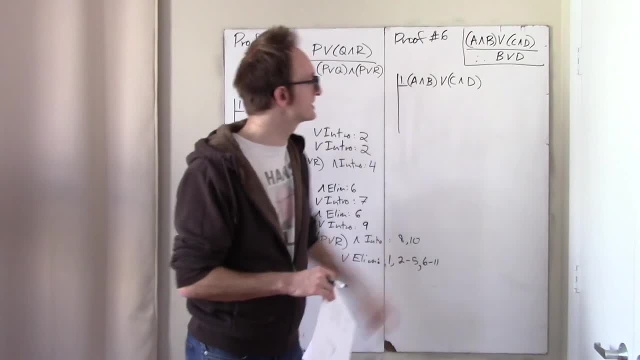 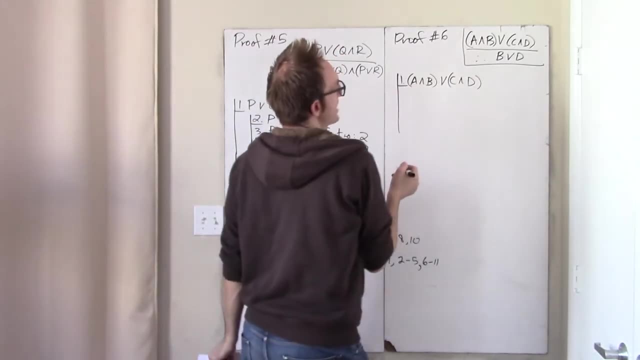 kind of let your eyes glaze over the stuff inside the parentheses and just see line 1 for what it is. Line 1 is a disjunction, And if this is a disjunction then we sort of have to do a proof by cases. 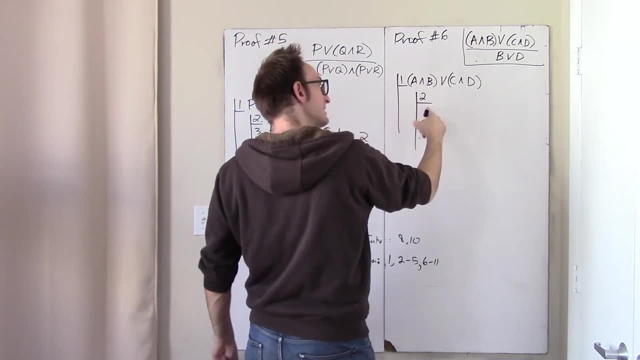 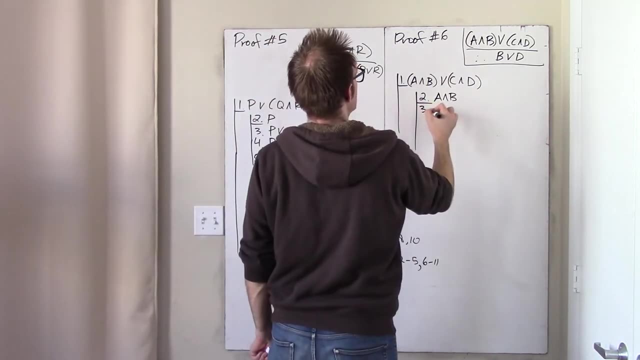 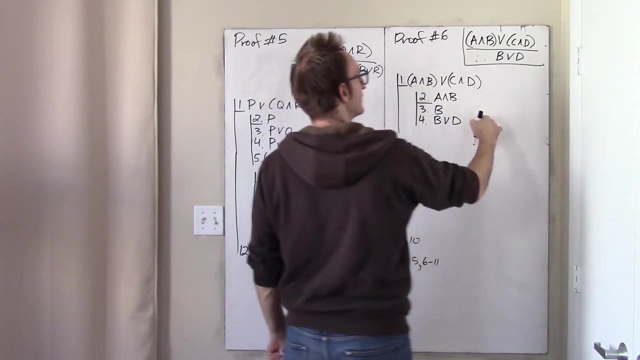 It's the only way. So I indent here to begin a proof by cases, starting with A and B. But okay, if I know A and B, then I certainly know B, and then I certainly know B or D. Here this is, and elim 2,. 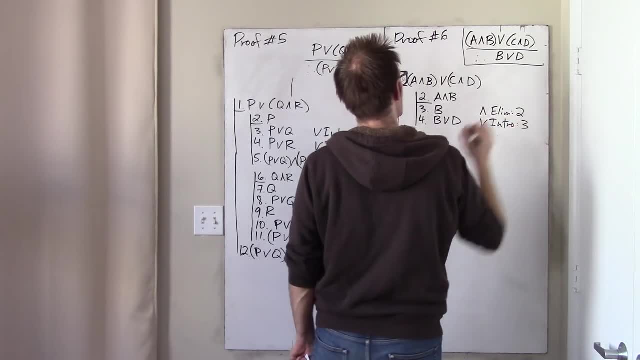 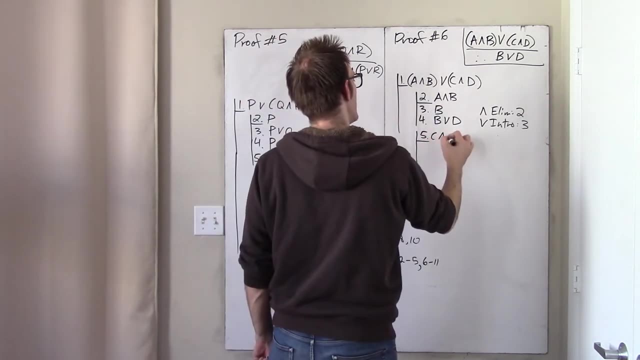 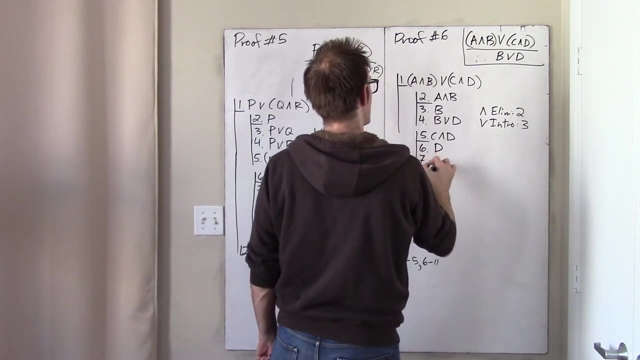 and this is or intro 3.. Okay, then I will try the other, disjunct C and D. Well, from this I conclude D, of course, and from that I can. or on B. Okay, I'm now sort of pretty much done, right. 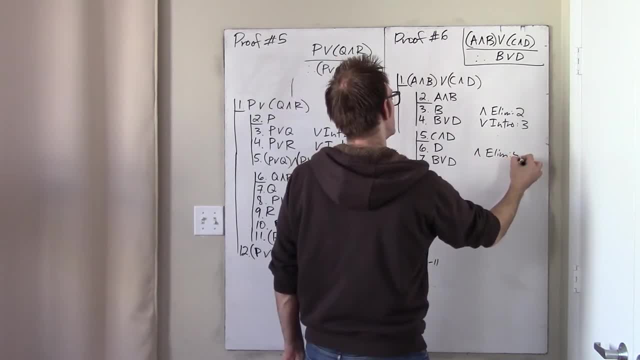 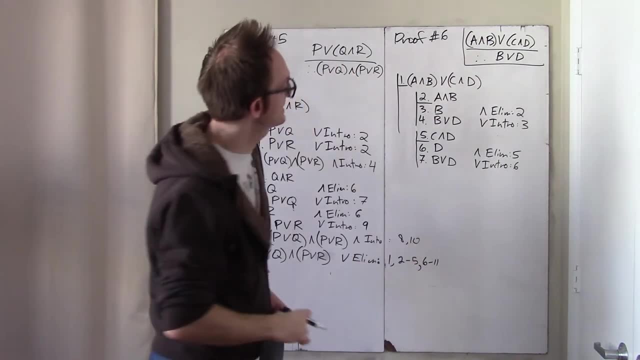 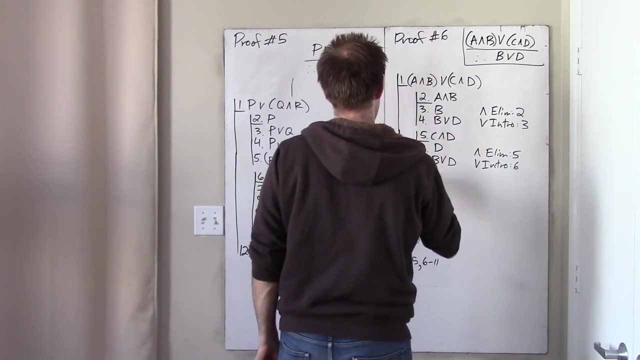 This line 6 came from an and elim 5.. This line 7 came from an or intro 6.. I did a proof by cases. now, Both of my disjuncts led to the same conclusion and therefore that conclusion just holds. 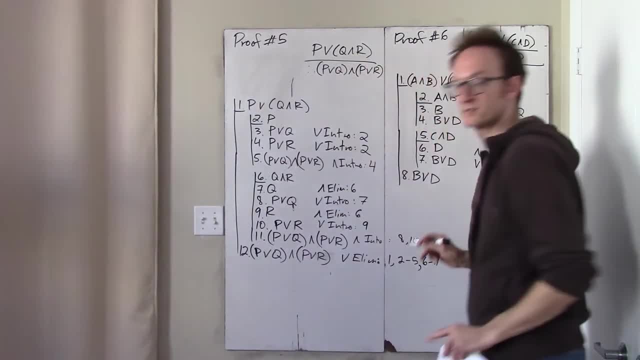 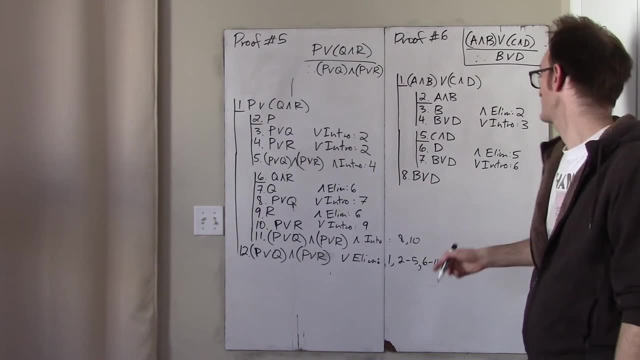 B or D. And you know, just because my proposition in line 8 is a disjunction, the justification for this line 8 is a disjunction: elimination. because the justification for line 8 is that it was the result of a proof by cases. 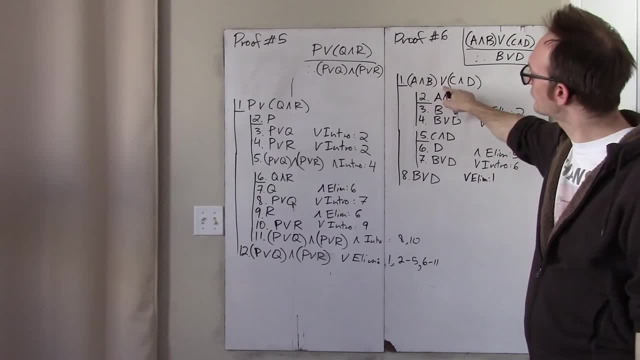 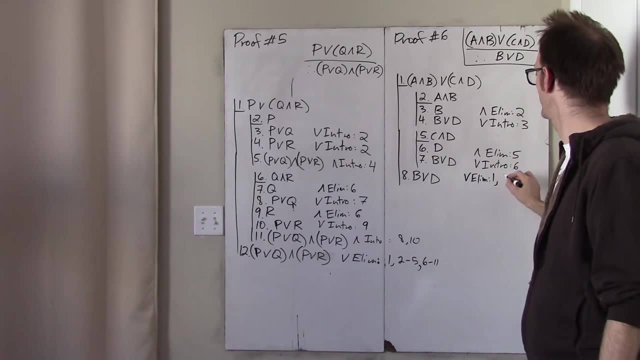 In other words, I began with line 1, I eliminated that disjunction in line 1 by virtue of conducting the proof by cases on that disjunction, And I did that via the subproof 2 through 4 and the subproof 5 through 7.. 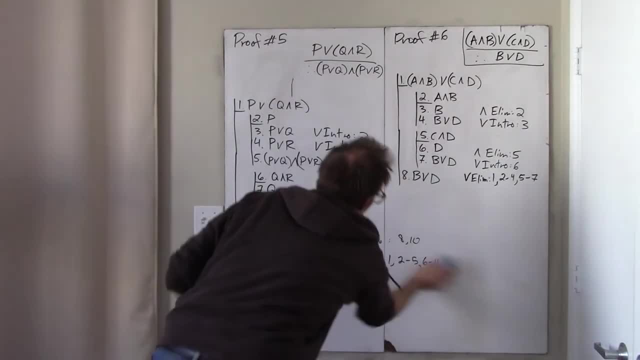 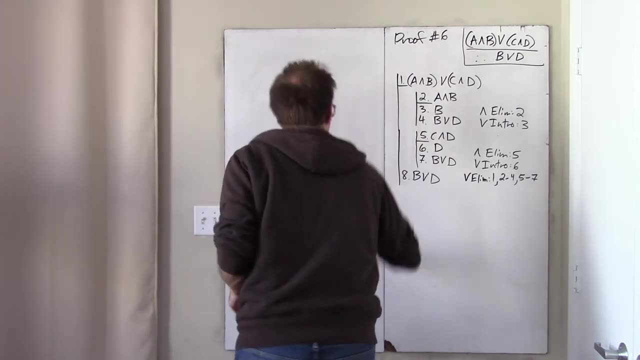 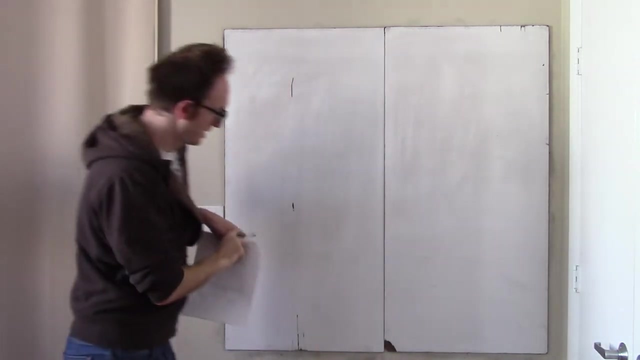 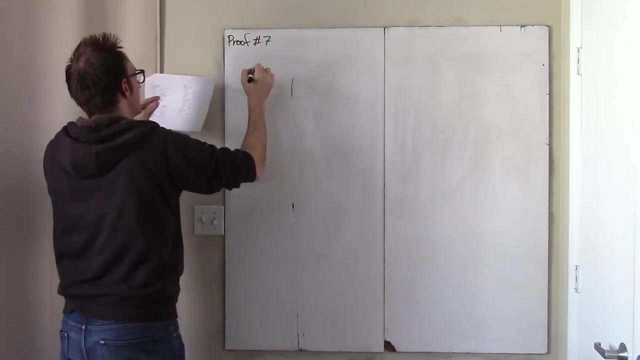 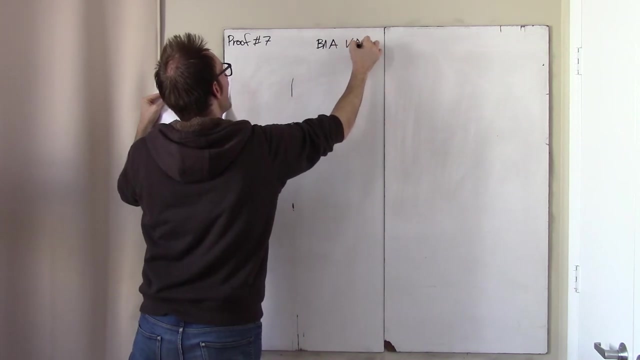 Okay, we're just going to keep going, Yeah, 7.. Proof number 7 says: all right, take this premise B and A or A. I hope I haven't changed this packet at all. I think this is still proof 7.. 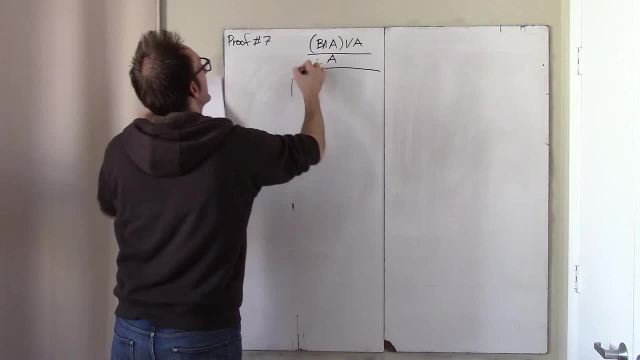 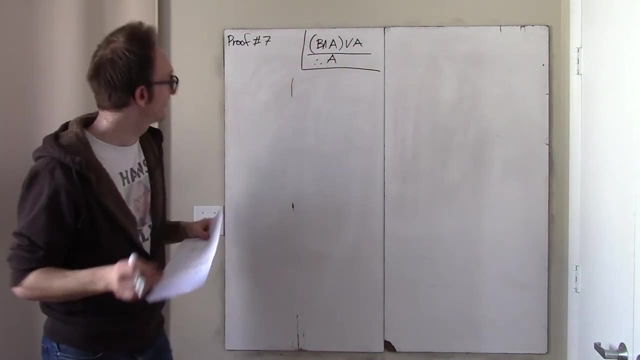 And from this I'd like to conclude. A- Is this argument valid? Oh, of course it is. Come on Either B and A so A, or just A so A. But there's actually a nice opportunity here to learn something. 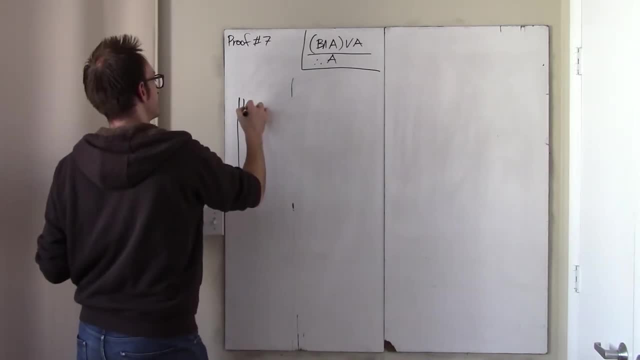 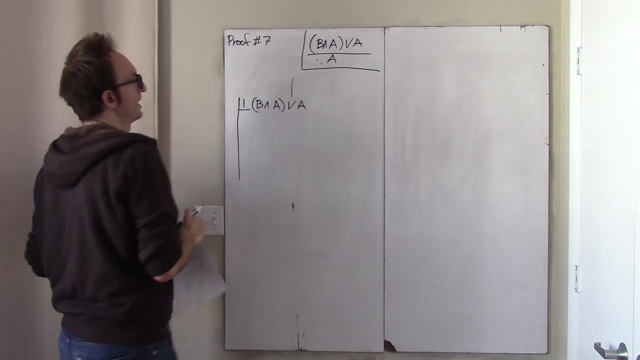 Well, there's one sort of feature of our system which you're about to be exposed to. So B and A or A, Okay, well, I have a disjunction, of course. so I need to do a proof by cases. 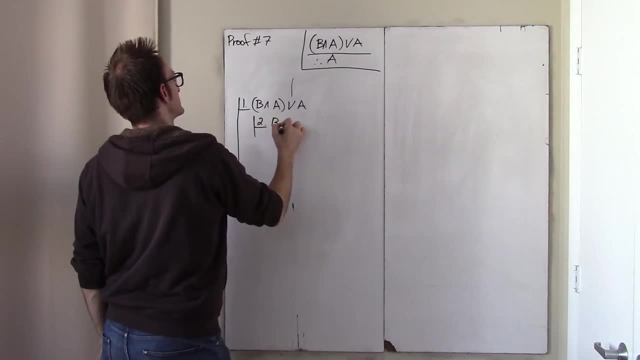 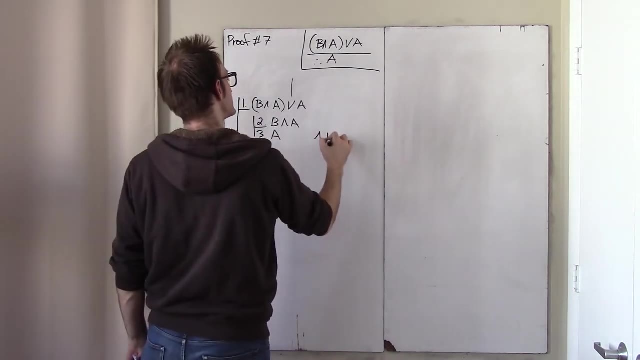 so I just begin that proof by cases kind of without delay. So I have B and A And all right, it seems I'm done because there's just A right. So reason and elim line 2. All right, so far, so good. 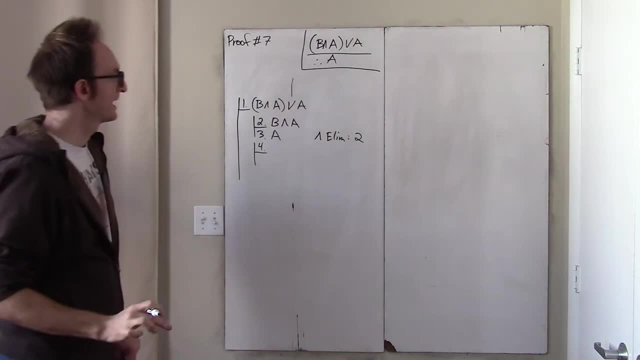 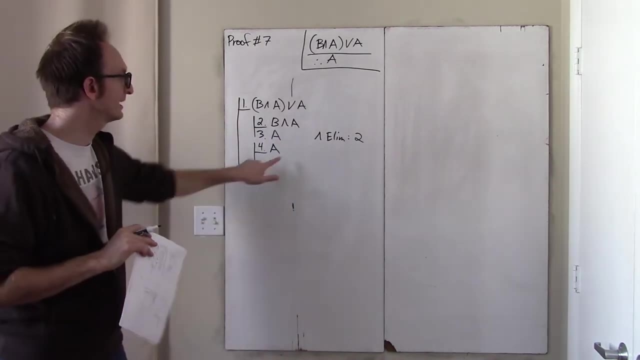 And now the sort of nature of our proof system is that I consider the other case, the other case being A, But now I see that, like I already, even just in the premise, have the thing that I want. So, okay, you know. 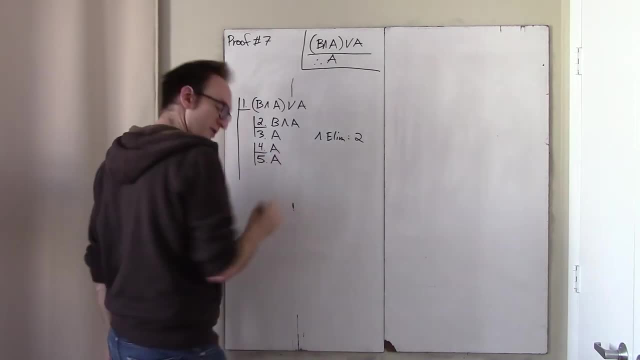 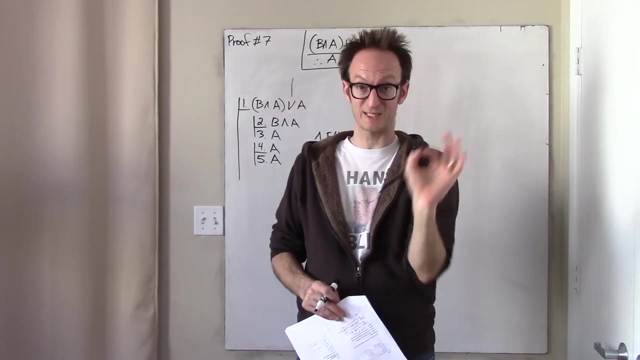 you could argue about this kind of thing, but you know the sort of. the formal nature of this proof system requires that you stick to a certain precise syntax. I'm talking about the syntax of the proof itself, And here the syntax of the proof itself is. 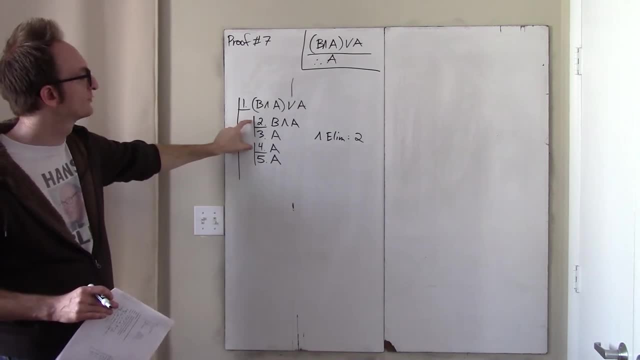 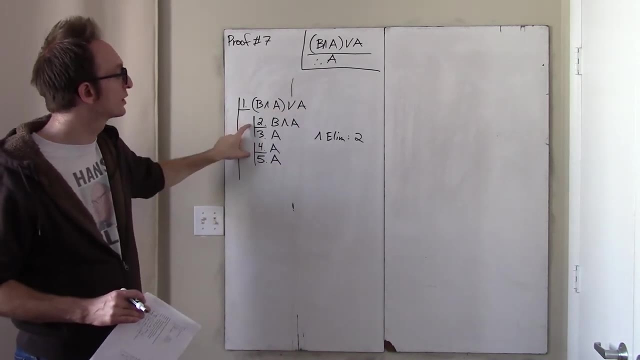 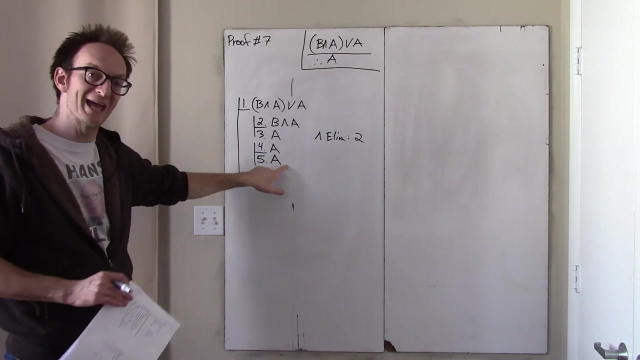 that these two things here in line 2 and 4 need to be the disjuncts that you're exploring, and each of these sub-proofs need to conclude with some kind of line here, And so it is for that nature that I really do want to sort of rewrite that A like that. 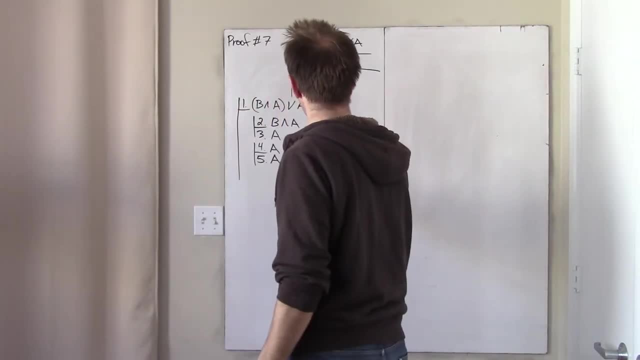 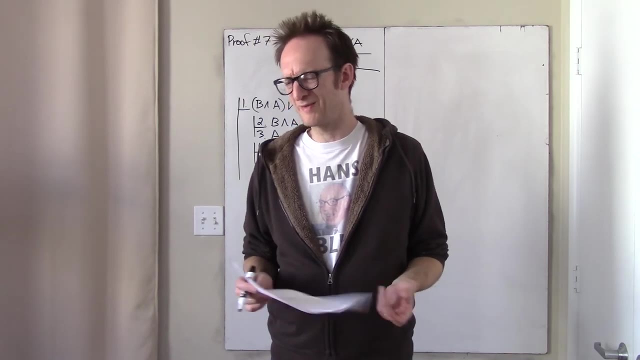 And so there's a rule for this. It's called reiteration, And I think I mentioned this as maybe the very first rule of this proof system in class. I did, And you might have thought: why would I ever want to just like? 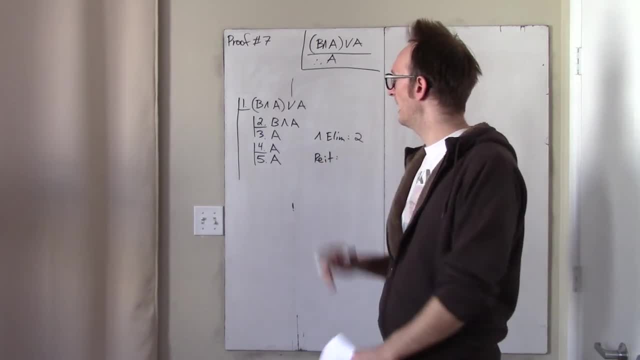 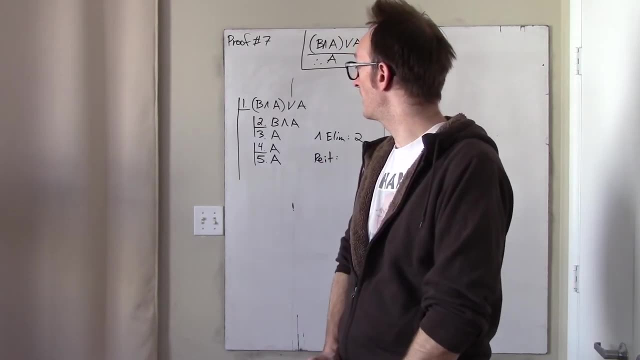 restate something for no particular reason. Well, sometimes you need to kind of force your. you need to force your proof to be in a certain format in order for the proof to be correct according to the rules we've set up, and this is one of those cases. 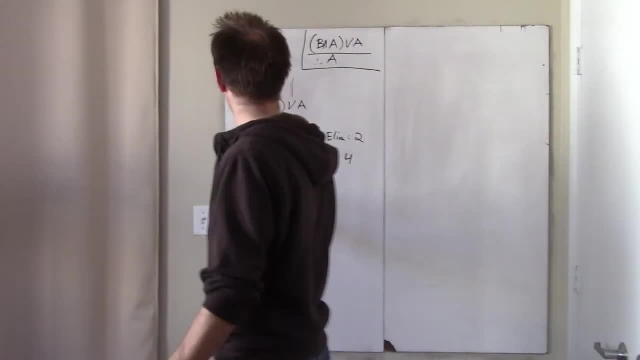 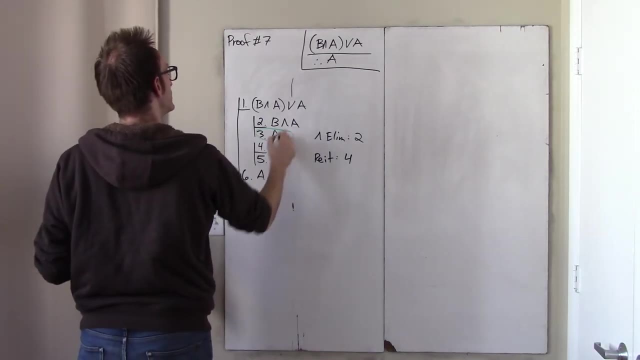 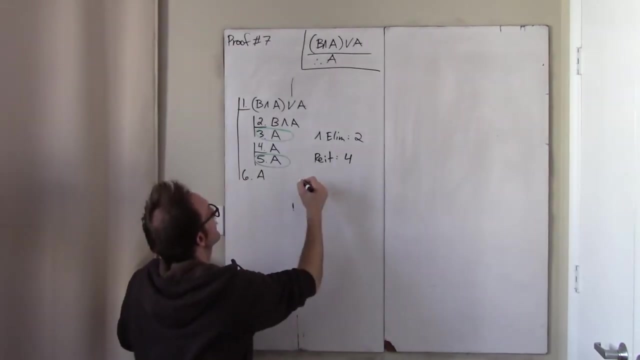 So I just sort of repeat line 4.. Therefore, I can say that line A holds. I just really needed both conclusions of each case to end in the same exact kind of way like that. Okay, and where did this come from? This is an OR elimination. 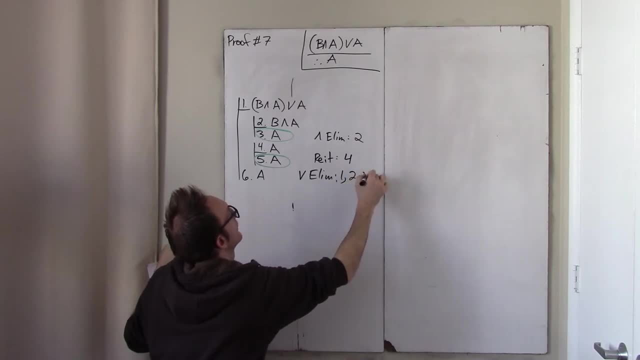 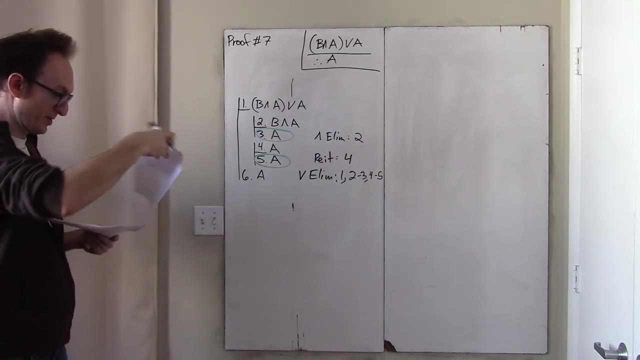 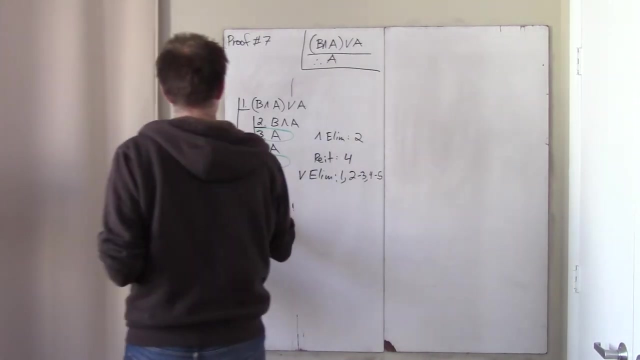 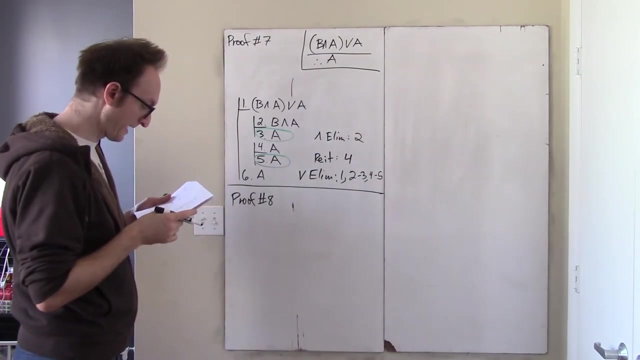 I started in line 1, and did 2 through 3,, 4 through 5.. Oh, we got a crying baby, but he's going to just cry because I'm doing three more proofs. Yeah, Proof 8 is quite short. 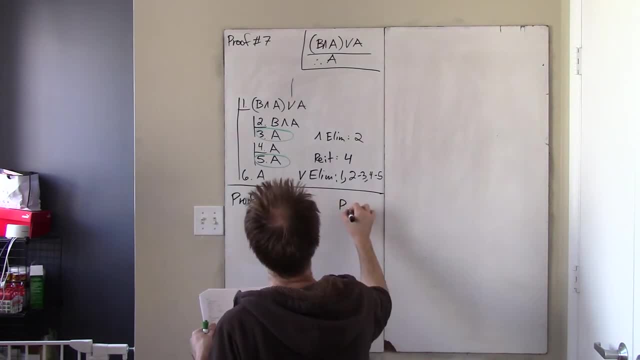 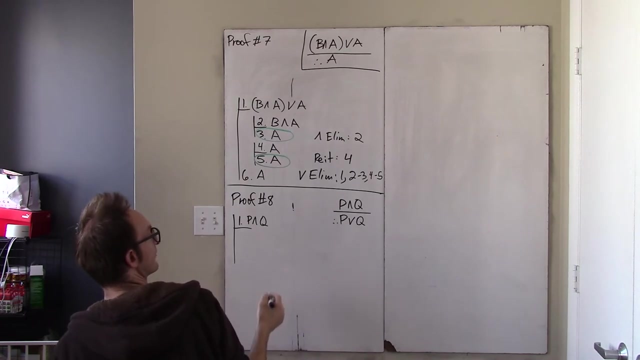 Not even sure why this is on here. Um, the argument says: dude, if you know P and Q, you can certainly conclude P or Q. Okay, this is just simple proof. We have P and Q. From this I conclude. 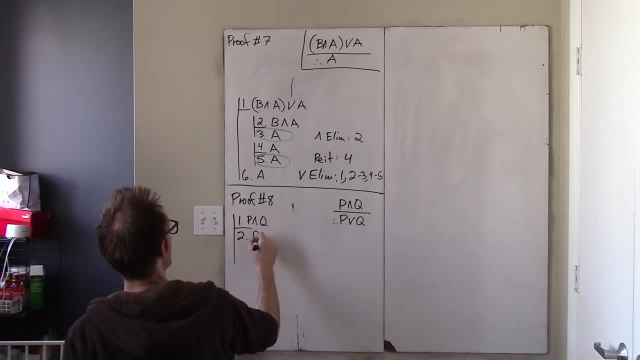 I guess there's a bunch of ways of doing this. I guess I can conclude P. I might have cut this proof out, I can't remember, Anyways. so from that I conclude P and that reason and elim 1, and then I conclude P or Q. 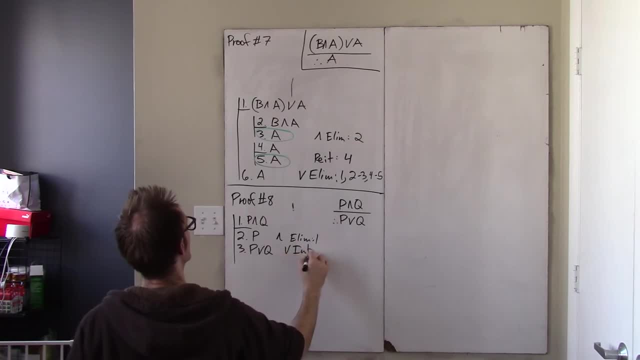 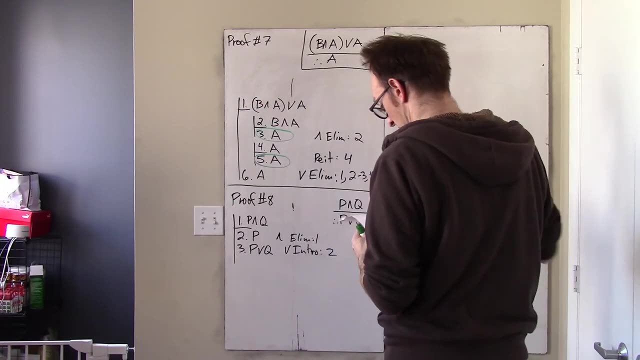 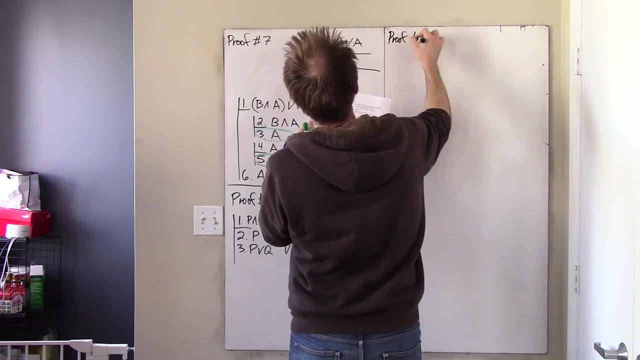 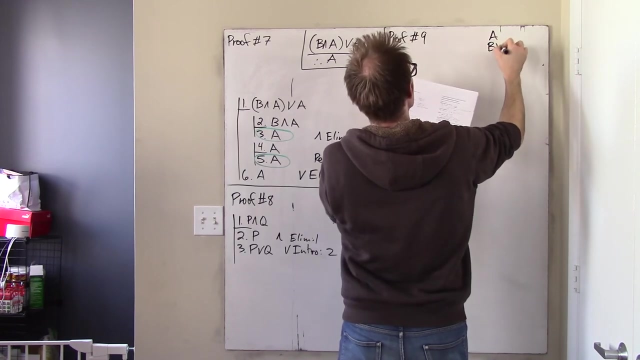 reason OR intro 2.. Okay, two more, Two more. Let's do it. I think I can squeeze them both over here on this board. There's proof 9, which says: okay, I have two premises, A, B or C. 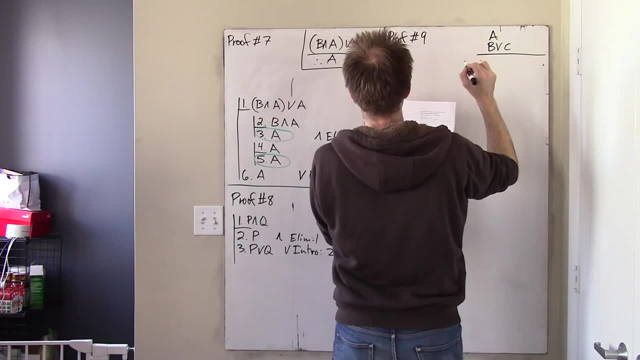 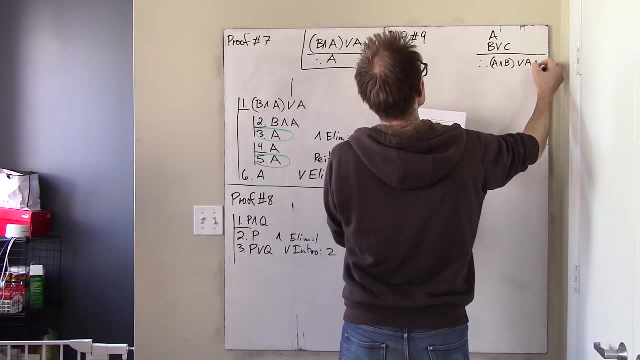 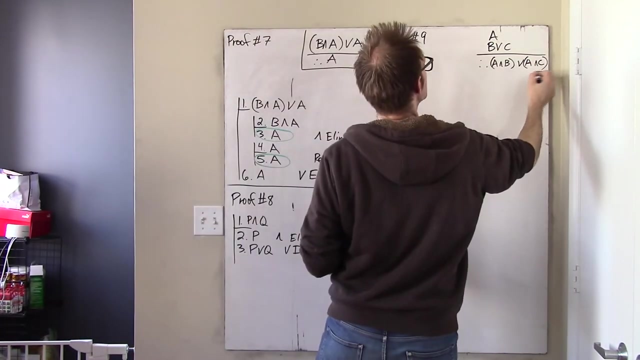 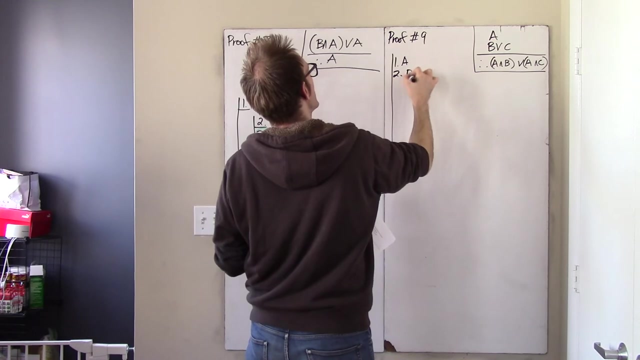 and from those two premises I would like to conclude: A and B or A and C, All right. Well, that seems pretty reasonable if you think about it. Let's not think about it too much, Let's just begin Line 1A, line 2B or C. 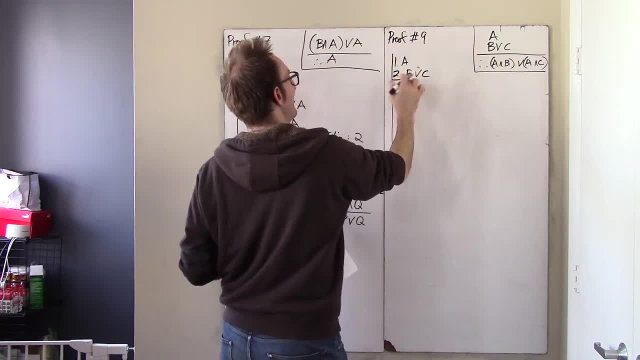 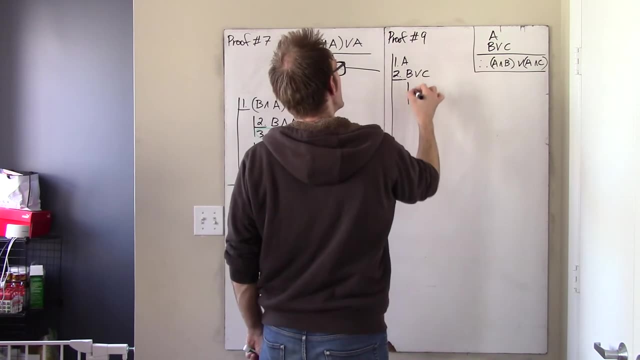 What am I going to do? Well, I have to use line 2 somehow, And there's only one way to use line 2, and that's to do a proof by cases. So let's do that proof by cases. now, I assume the left disjunct B. 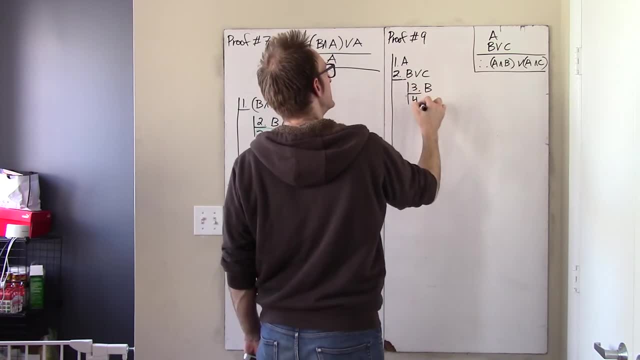 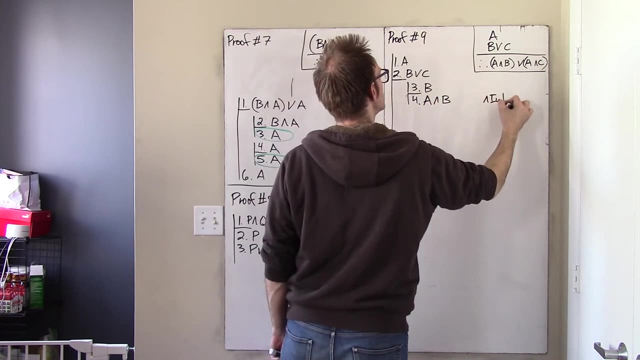 Oh, okay, Well, I also have line 1, right? So line 1 says that if I now have A and B, then I have A and B reason and intro 1 and 3.. But of course this is pretty close to the thing. 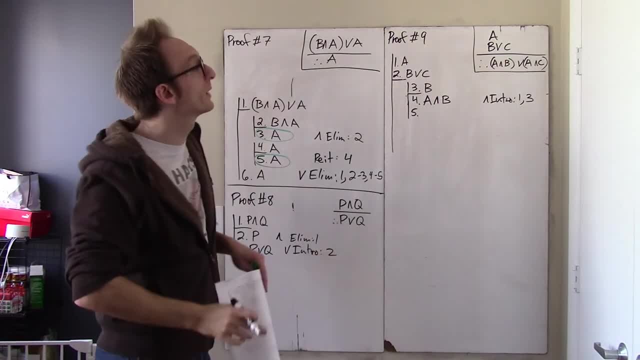 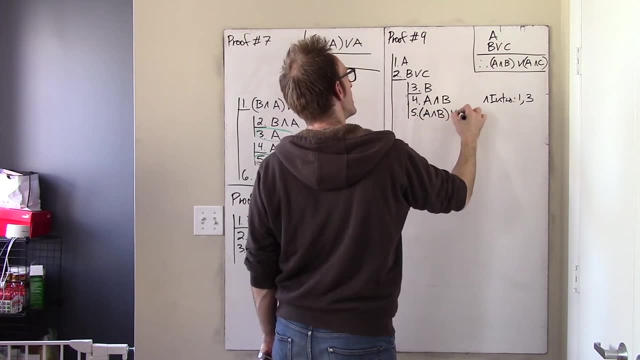 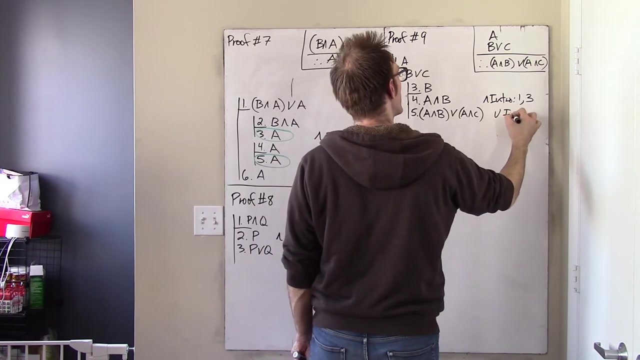 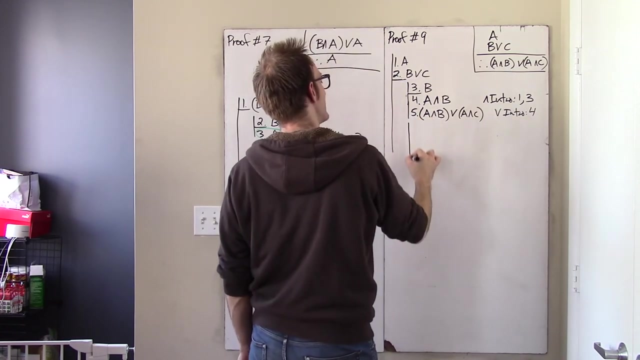 I'm trying to prove, because the thing I'm trying to prove is a weaker version of that, And so I say A and B or A and C, And okay, reason or intro 4.. Okay, And that concludes my left disjunct. 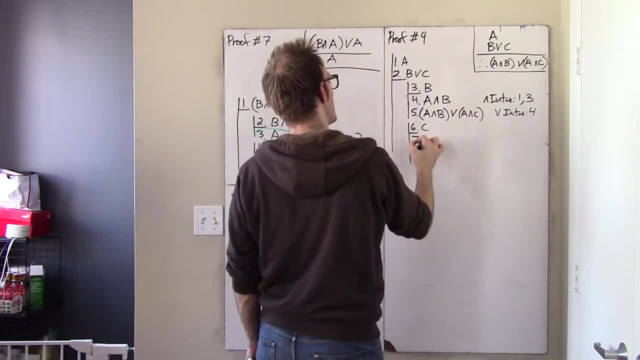 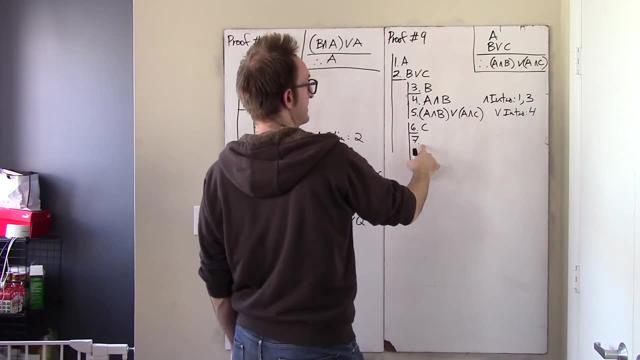 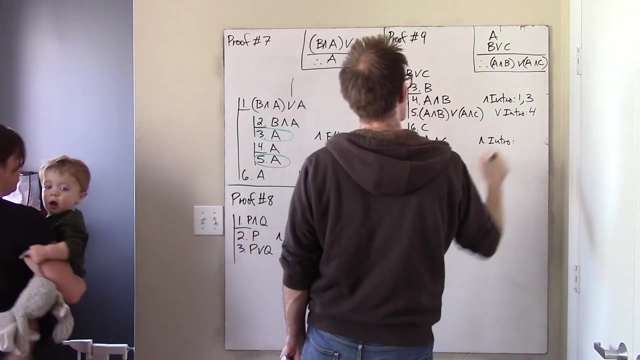 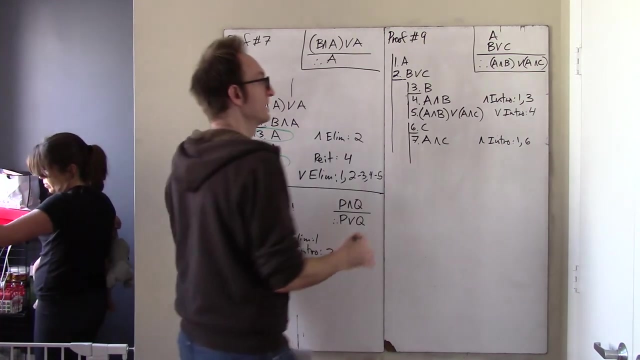 Now we go to the right disjunct, which is C, And yeah. So if, on the other hand, C, then I can make A and C by and intro 1 and 6.. And then that line 7 is pretty close to my conclusion. 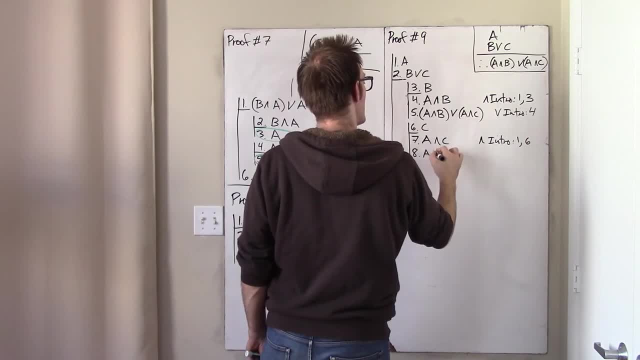 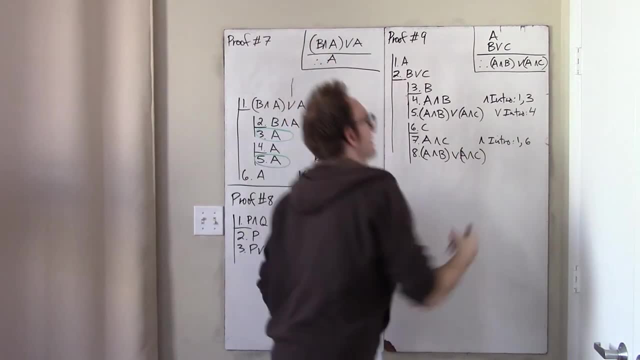 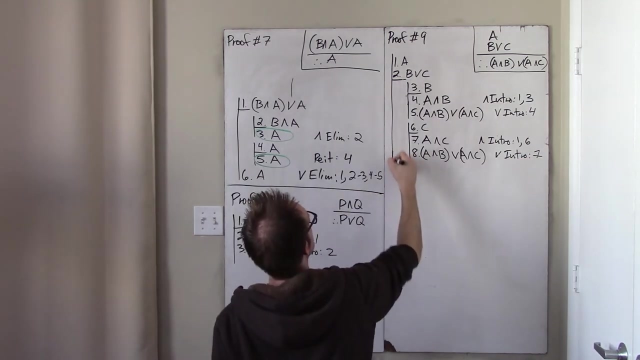 My conclusion is just a weaker version of that, So I OR on this thing to the front of it. Um yeah, And that is uh OR intro, uh, line 7.. And I did indeed hit the same spot in both of my sub-proofs. 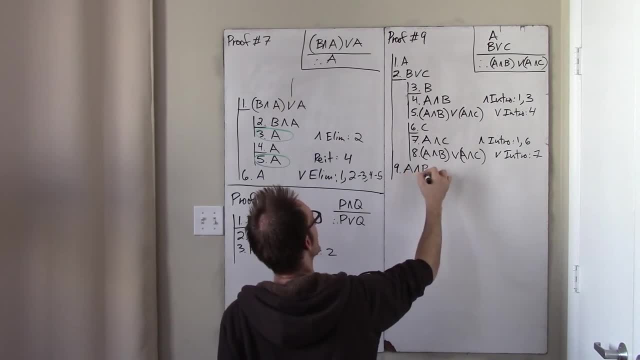 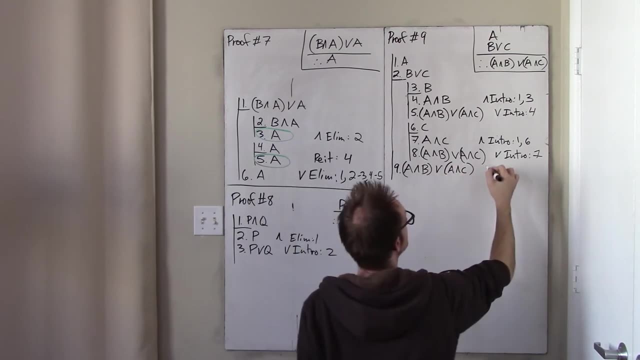 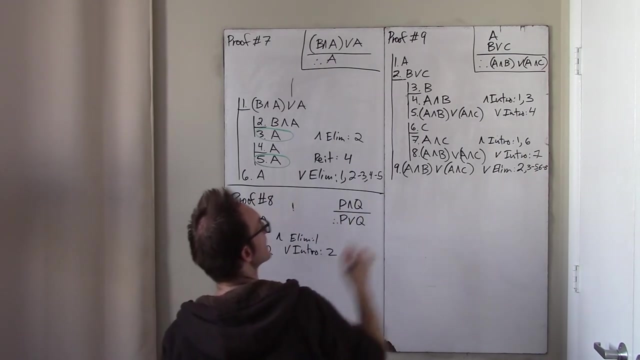 And so I may now assert back on the main line: uh A and B OR A and C, Uh reason OR elim, uh line 2.. Uh 3 through 5, 6 through 8.. Okay, Good. 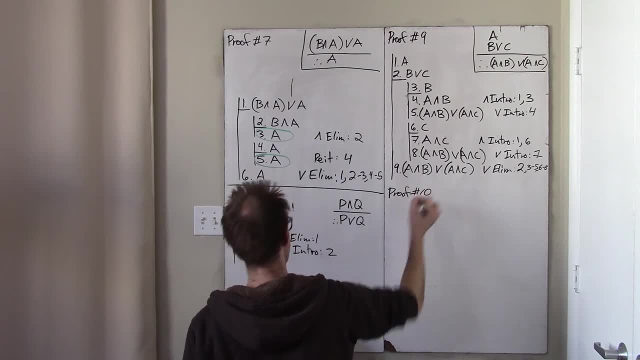 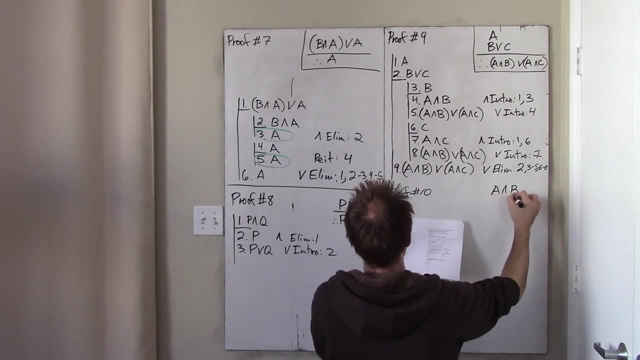 Last proof, Proof number 10.. Uh, this is what it says. I have a premise, The premise is A and B, uh OR C, And from this I would like to conclude C OR B. Okay, This one's kind of maybe a little bit nice. 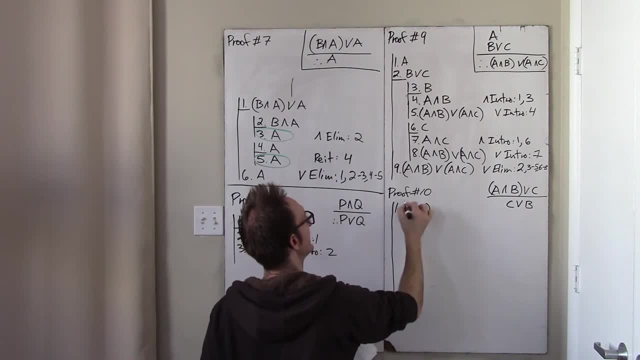 Uh, so let's go. My one premise is A and B OR C And um. uh well, once again, the main connective is a disjunction. So there's only really one way to do this, which is to do a proof by cases. 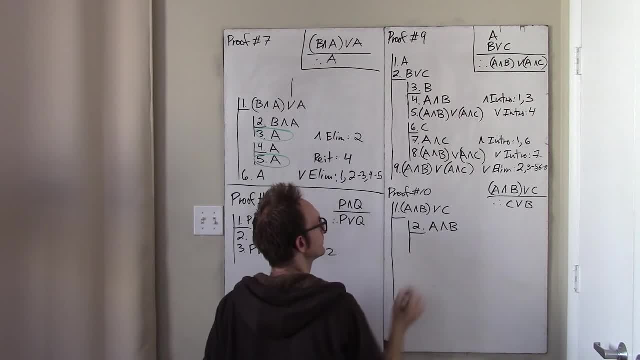 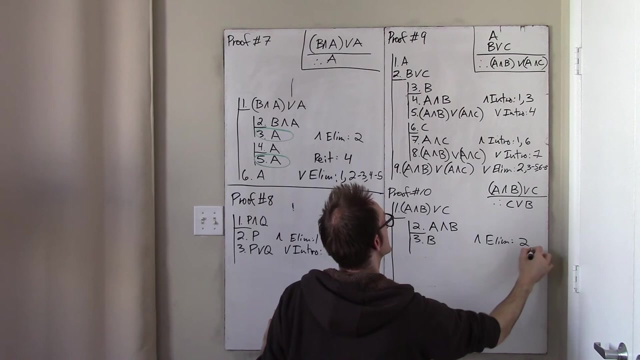 So this is A and B? Um, okay, Uh well, my goal is C OR B. So, keeping that in mind, from this I can get B reason and elim 2. Just comes directly from line 2.. And now I can just OR a C. 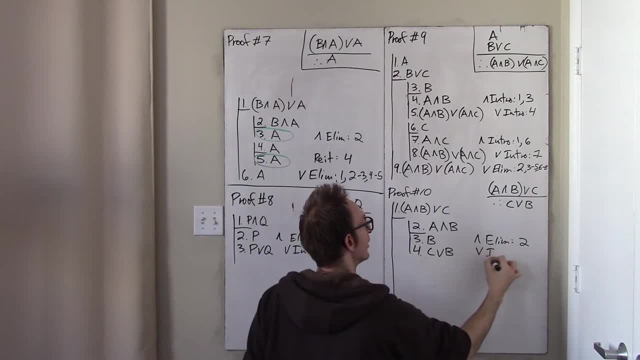 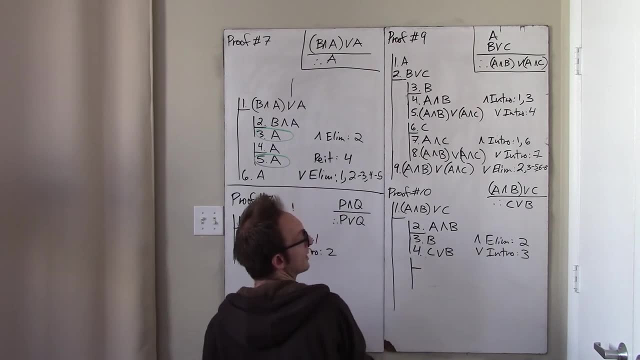 onto the front of that B, Uh reason, OR intro 3.. Okay, That concludes that, uh, sub-proof. Um, what about the other option? uh, that that it was C, that was true, the right disjunct. 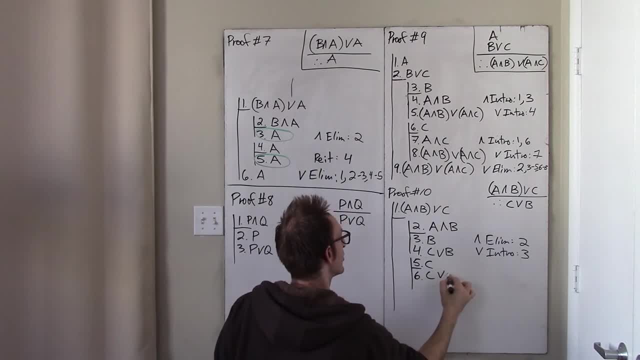 Well, now it's even sort of simpler to just OR on that B. So that's OR, intro 5.. And here I have uh concluded C OR B. So back out at the main, uh body of the proof. 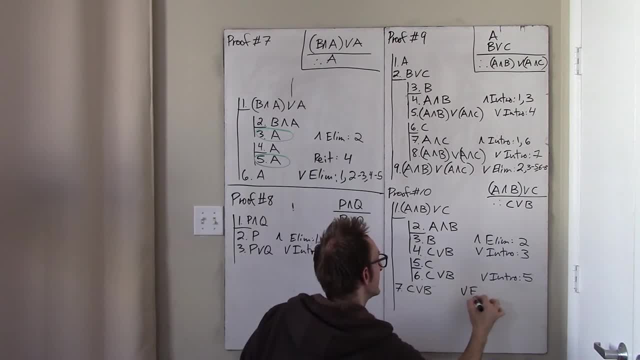 I now know C OR B, Reason OR elim. In other words, I started with line 1.. Uh and um uh. yeah, Sorry, zone out for a second: Um 1, uh. 2 through 4, 5 through 6.. 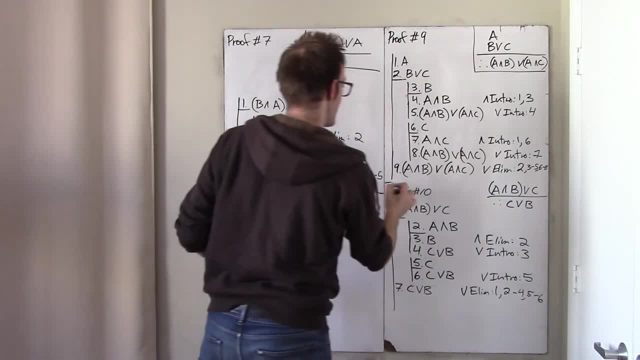 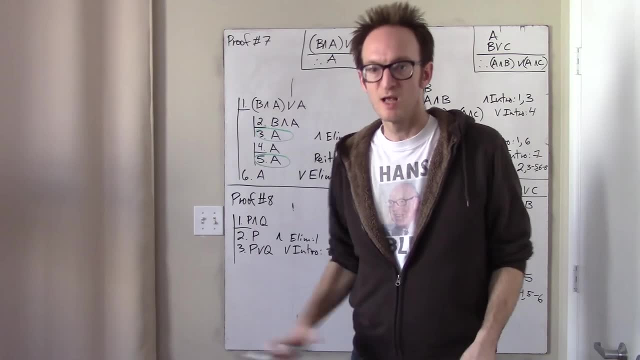 Okay, There it is. Uh, this is a um, uh, this is this is me doing all of proofs 1 through 10, but also kind of uh, uh, making this video sort of appropriate to an audience who even. 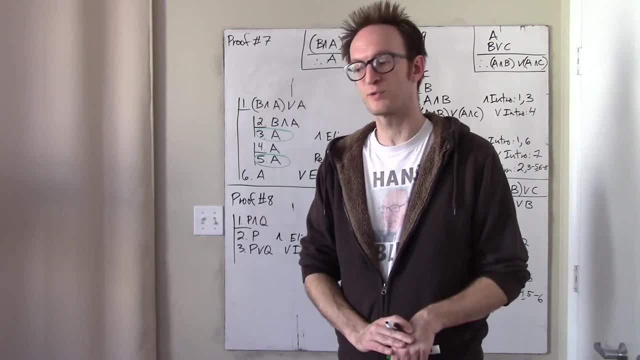 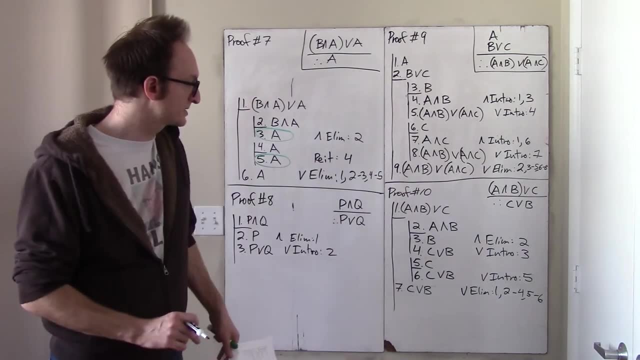 uh, who even maybe didn't have the packet and wasn't even there for for the lesson. on on on what the whole point of all this was, Um, so hopefully this was helpful for whoever is watching it. Uh, this is, this is uh. we are in no way complete.